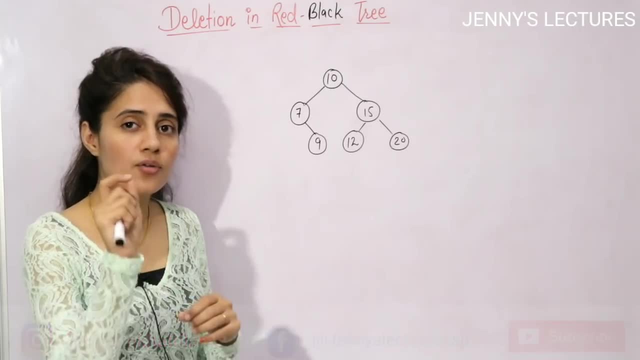 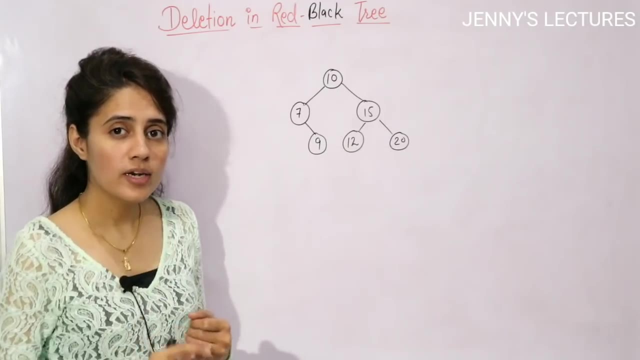 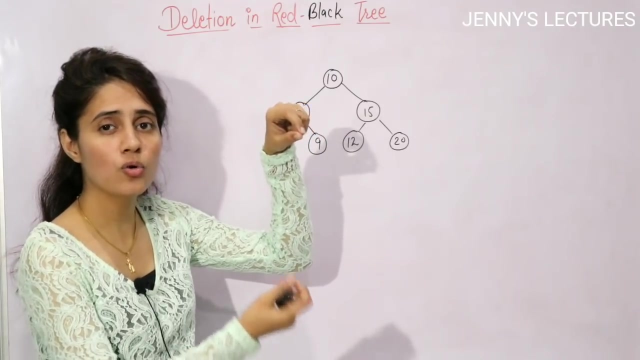 you will do. We always create a node in red color and we will insert as a leaf node. Then, in that case, which property Red? Which property is going to be violated? That red-red conflict property? right, Because if parent is red and always we will insert a node in red color, then parent and child would be red. but this should. 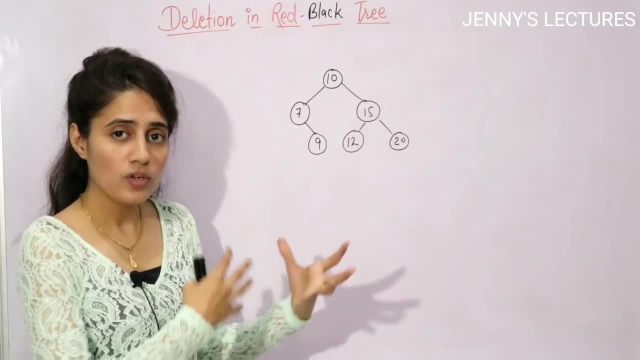 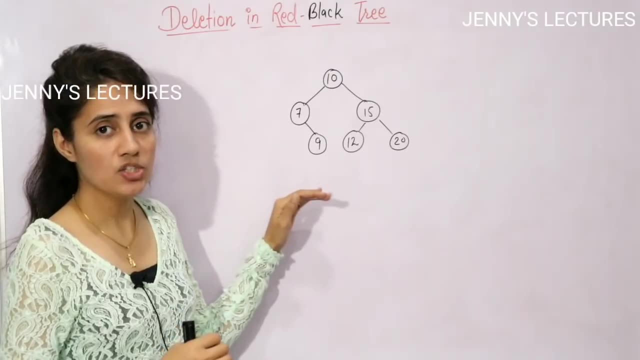 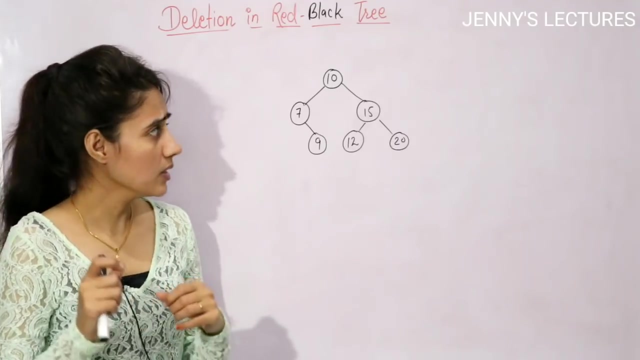 not be a case in red-black tree Right. So for solving, for resolving that conflict, we need to do some rotations or recoloring. Fine, now here in deletion, out of these three important properties of red-black tree, which property is going to right? see, if you are going to delete a red node, then there would not be any. 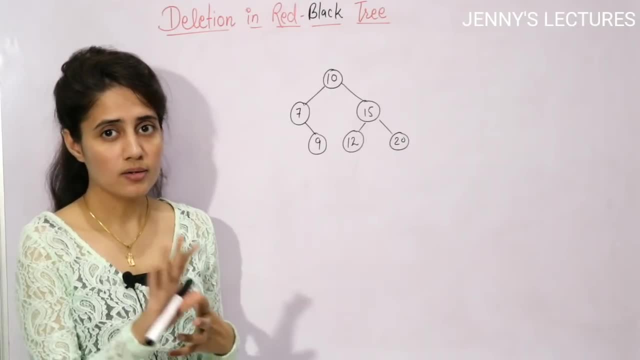 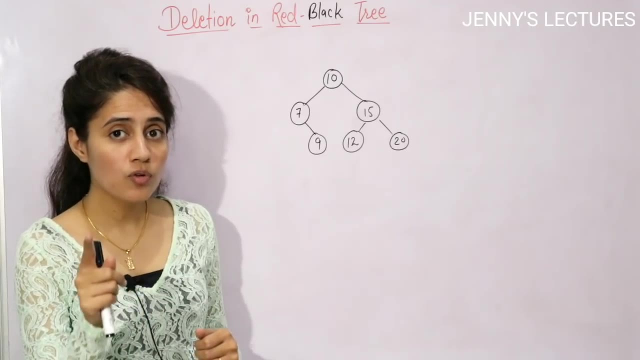 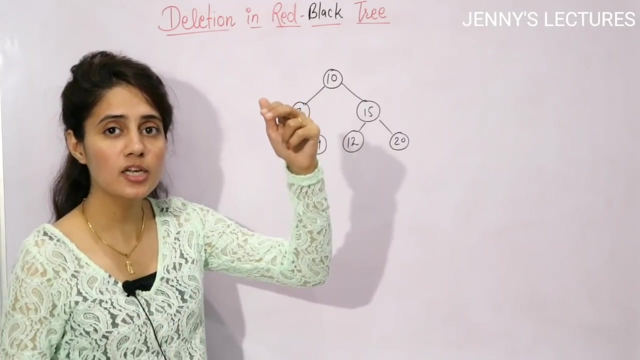 problem. just delete that node and exit, right. but if you delete a black node, in that case which property is going to be violated? that the number of black node in each path from any node to its descendant nil node would be same, should be same. that property would be violated if you delete a black node, because if 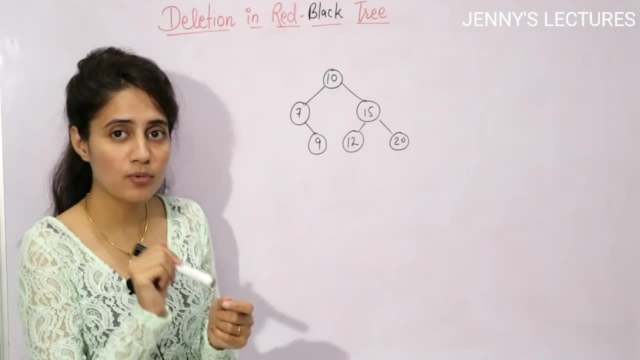 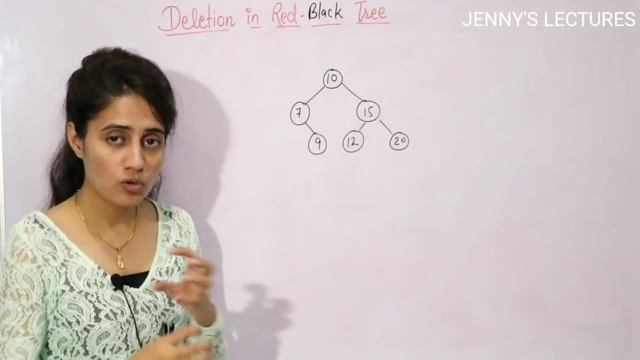 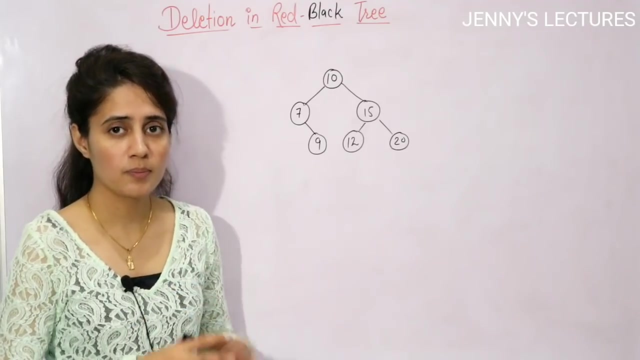 you delete a black node, then in that path the number of black node would be less than the other paths. then you need to take care of that property. so, first resolving that issue, you need to do some rotations, maybe some recoloring as well. many cases are there. we will see all the cases. simplest case is what, if you want? 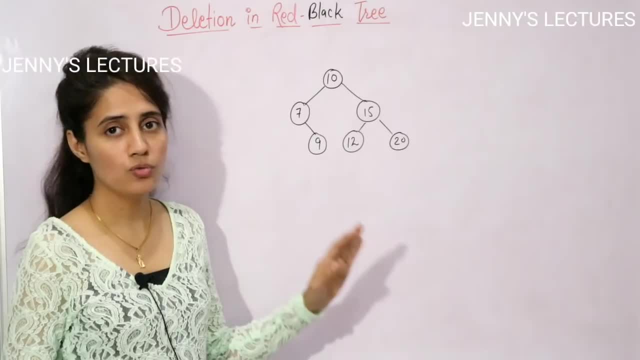 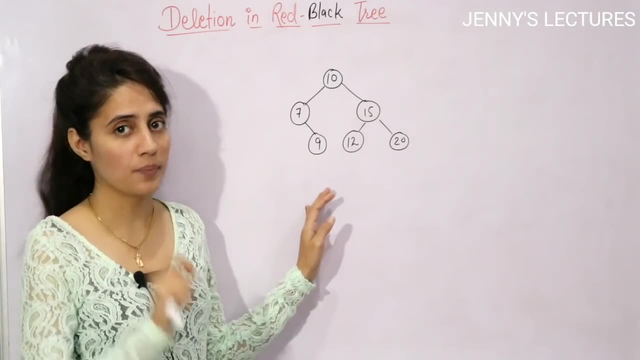 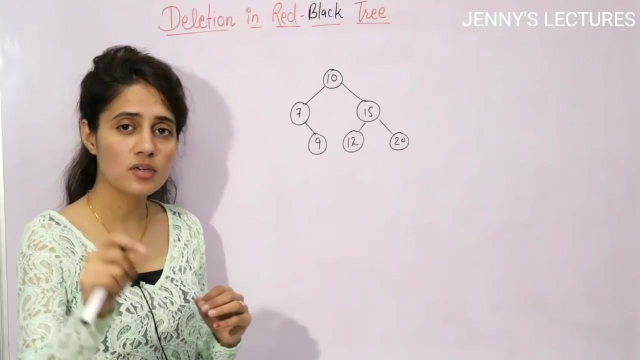 to delete the red node, simply delete it, no need to do anything. but if you want to delete a node and that node is black node, in that case you need to do something. now, in deletion, the very first step is what you have to perform, just standard binary search tree deletion. 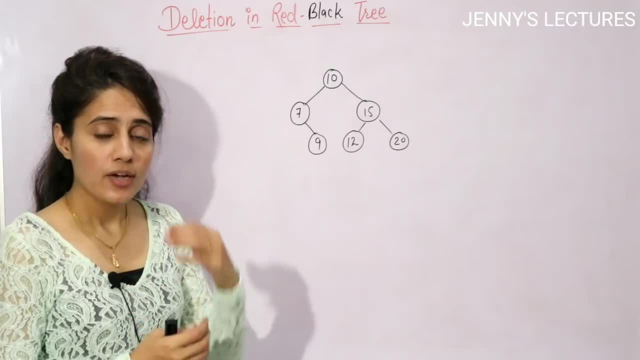 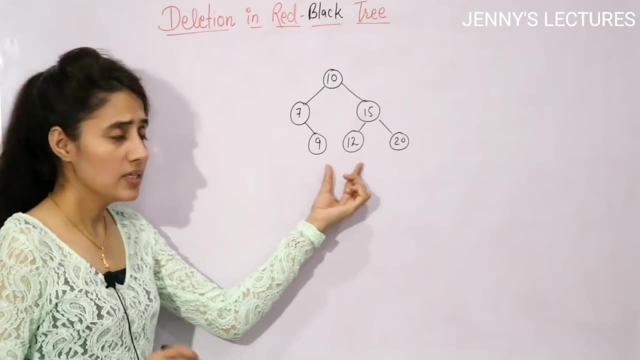 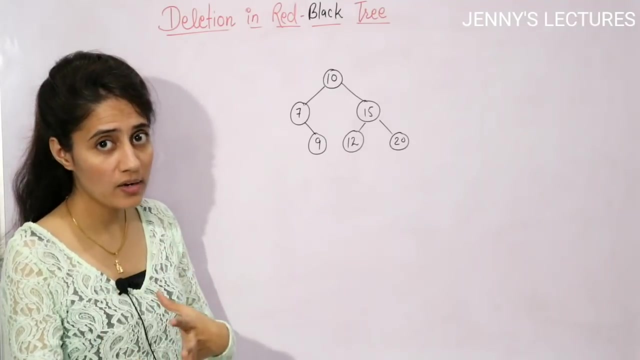 right now how to delete. see, I have already discussed insertion and deletion in binary search tree. you can check out that video in the side button, right? suppose I am taking this as a binary search tree and here you want to delete this 12? first of all, we need to search 12. where is 12 in this tree? we? 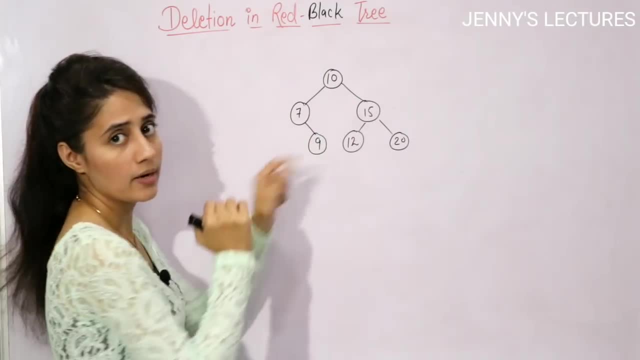 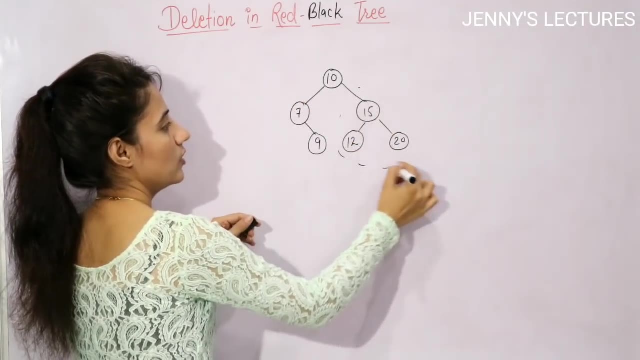 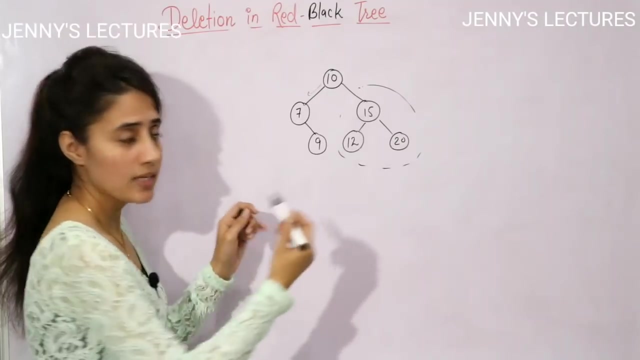 have the address of the root node we are going to start from here. 12 is greater than 10, so we know that 12 would be here in the right subtree of this 10. no need to check the left subtree right now. again, 15 means 12 is less than 15, so 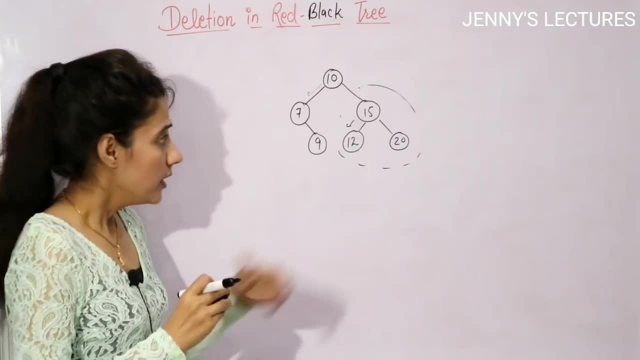 just go left. so here you find 12 right now. if the node you want to delete is higher than 15, then you can delete this 12, and if you want to delete this 12, then you can delete this 12. and if you want to delete this 12, then you can delete this 12. 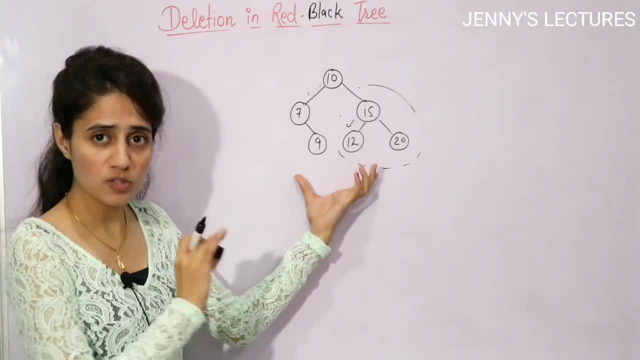 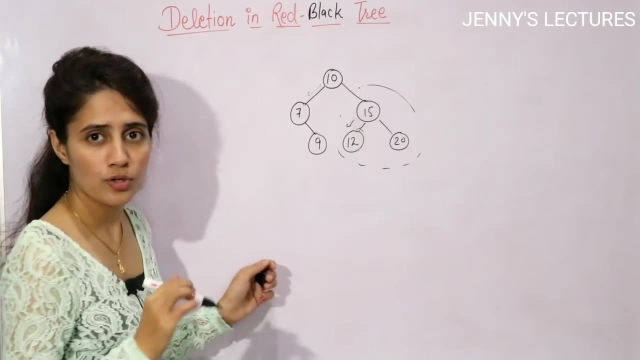 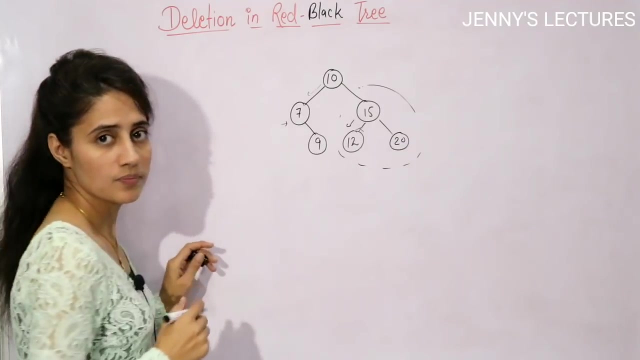 having no children. I am just considering. I'm just taking a case of binary search tree. I'm not taking red black tree here, right, so simply delete it. no need to do anything right now. second case was: if the node you want to delete is having only one child, suppose I want to delete this seven. first of all, search the seven. 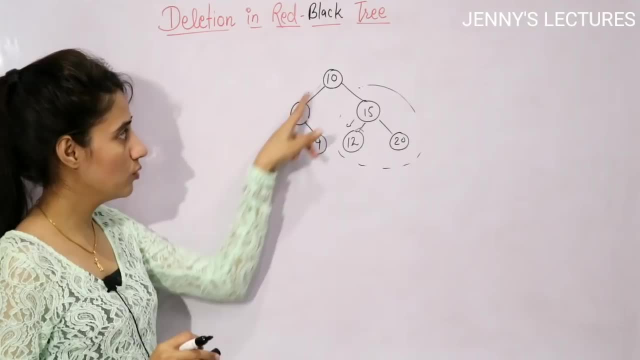 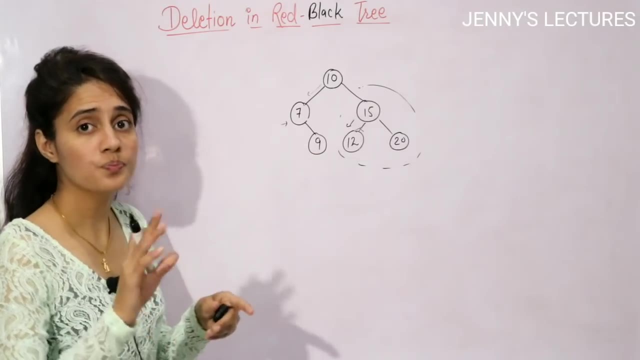 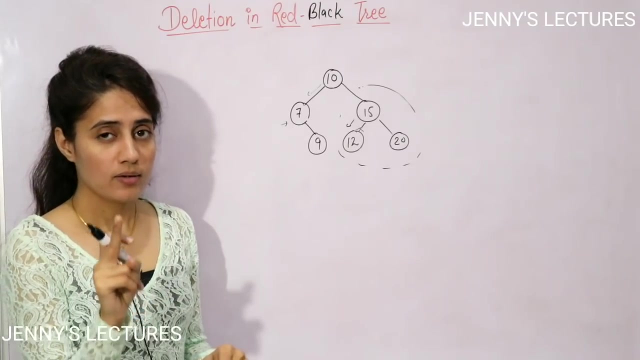 right. compare with this: 10 less than 10. so we are going to to the left of this 10. now here you got seven. now seven is having only one child, no problem, what you will do see now see seven is what an internal node. so one thing you need to take care when you are going to perform: 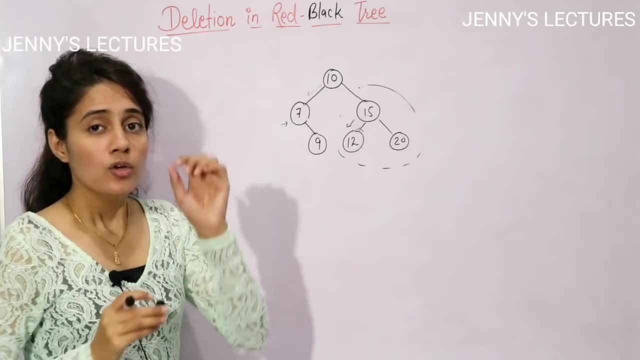 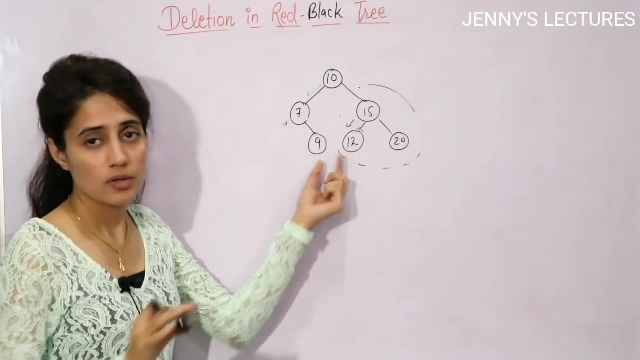 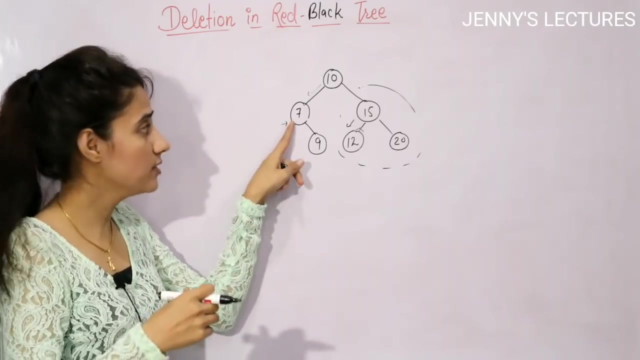 deletion in binary search tree or in red black tree. we do not delete internal nodes, right? we always delete leaf nodes. now, seven is what internal node? so you are not going to delete this node, you are going to replace it now. you are going to replace it with child, because it is having only one. 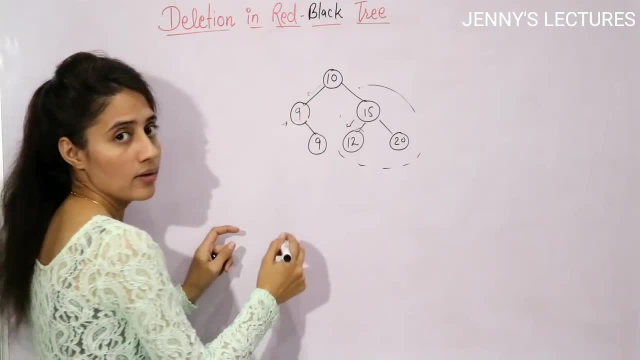 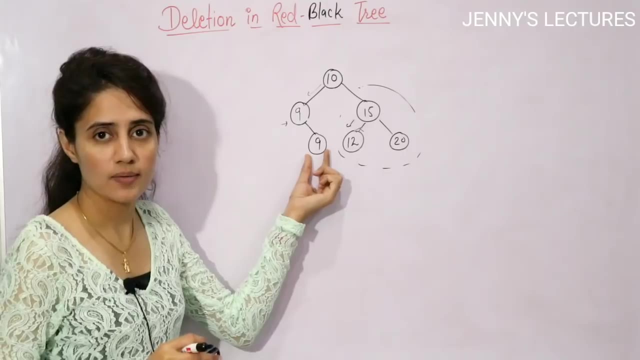 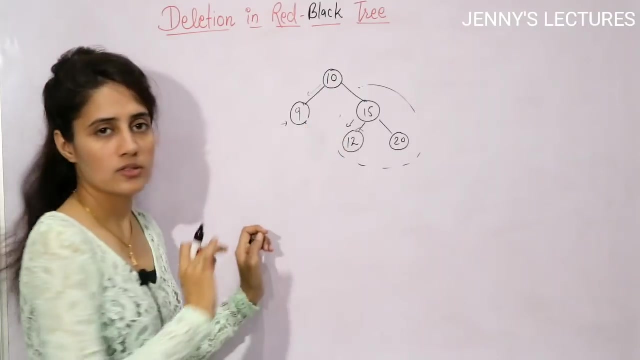 one child, so here you put nine. now here we have nine and nine. two nines are there now recursively. you are going to call the delete function on this child and now we are going to delete this child. only right. so after deletion. this is the binary search tree. 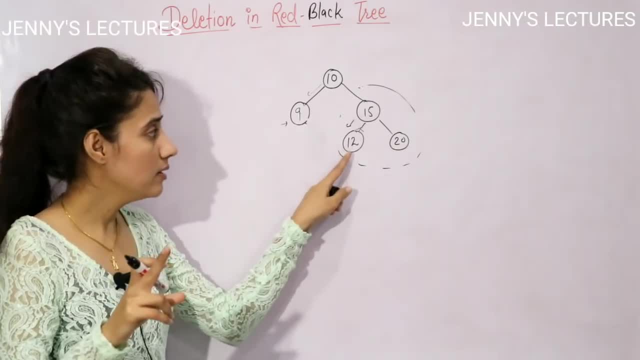 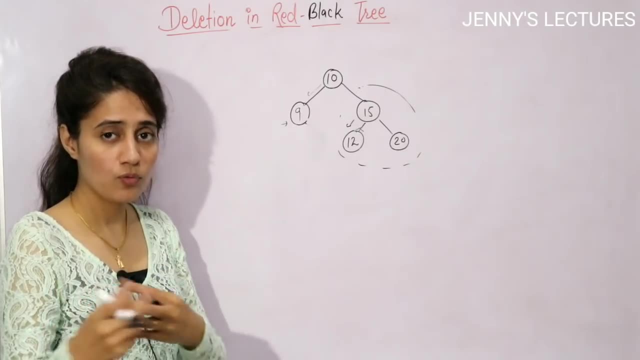 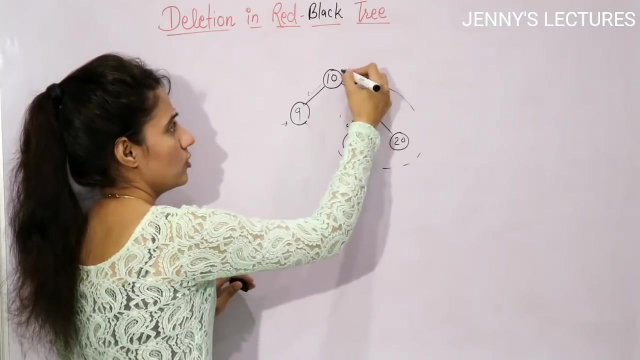 internal nodes. we are not going to delete, only we will delete the leaf nodes. internal nodes is going to be replaced with its children, right, with which child you need to take care of that thing now. third case was: if suppose i want to delete, suppose this 10, now 10 is having two children. 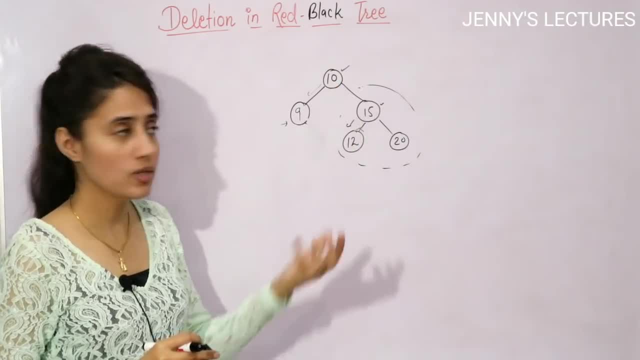 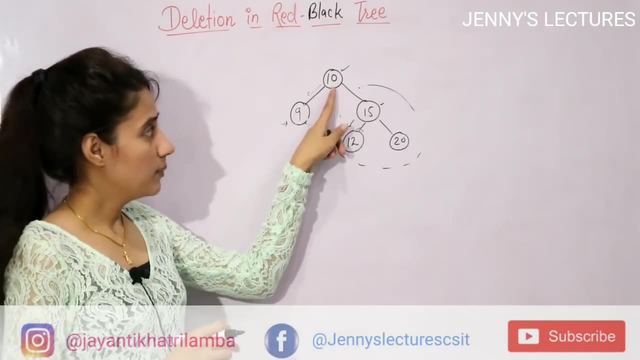 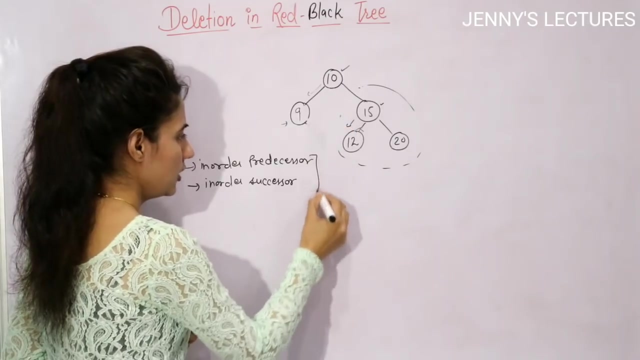 now we will replace this 10 with which children with 9 or 15, or with what? this thing you need to take now here. two cases are there. either you can replace it with its in order predecessor or in order successor. two cases are there, so these two approaches are there. suppose i am. 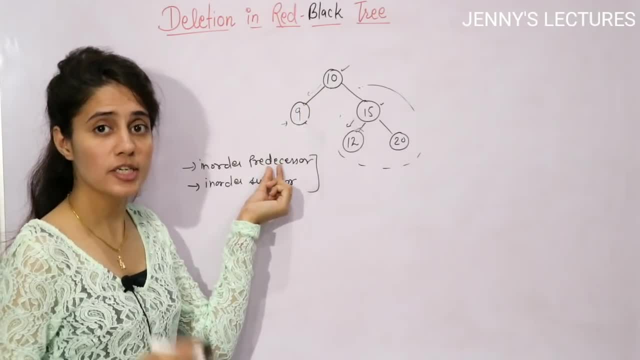 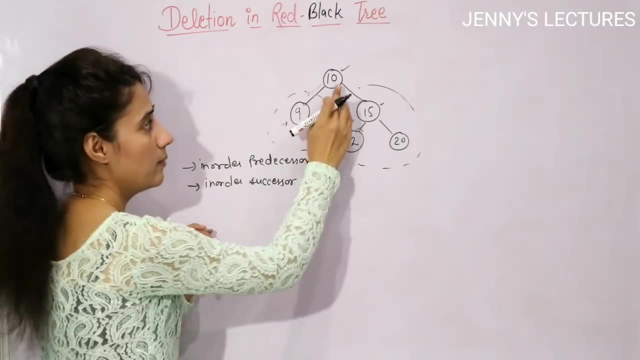 replacing this 10 with it's in order predecessor. predecessor means in order, predecessor means the largest element from the left subtree of that node, because i'm i want to replace this 10, so find out the left subtree of this 10 and from that left subtree. 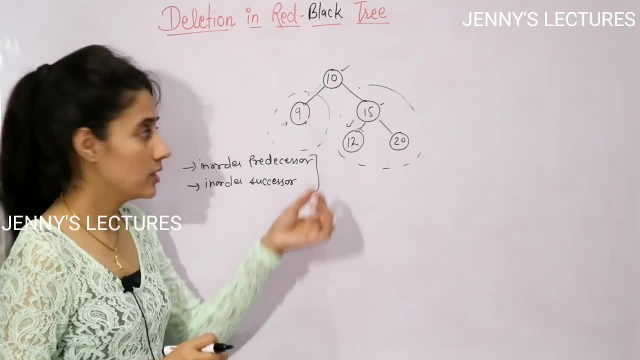 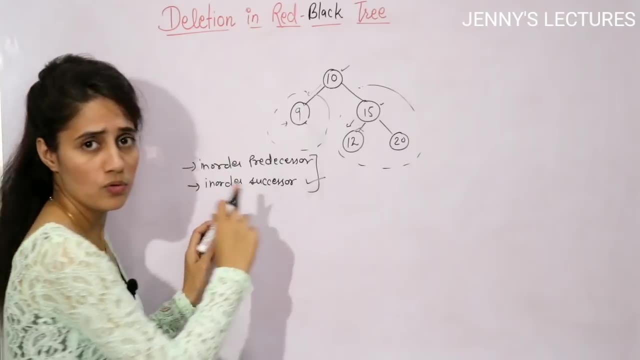 the largest element would be the in order predecessor means. here we have only one element. that is nice, so you can replace this with 9, or, if you follow this approach, if you will follow this approach, then you are going to replace this 10 with its in order successor. now how to find in order successor. 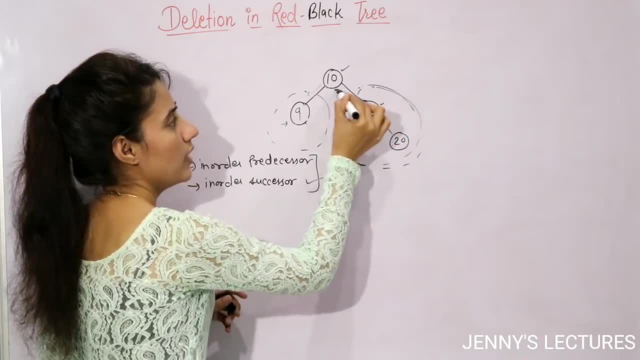 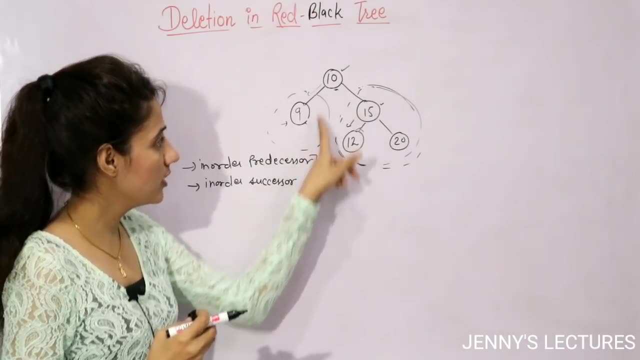 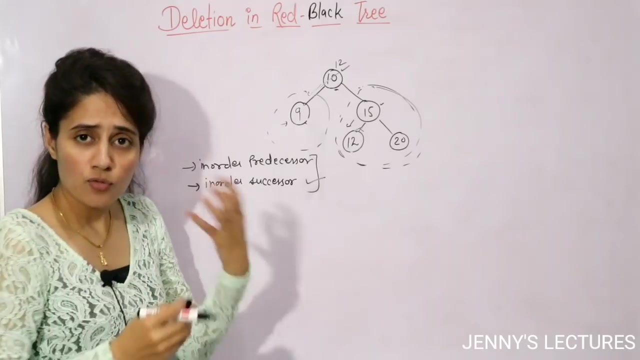 the smallest element from the right subtree of that node. right, i want to replace this 10. or you can say i want to delete this 10. so the right subtree of this 10 is this one. now the smallest element from the right subtree is 12, so we are going to replace this 10 with this 12.. see how. 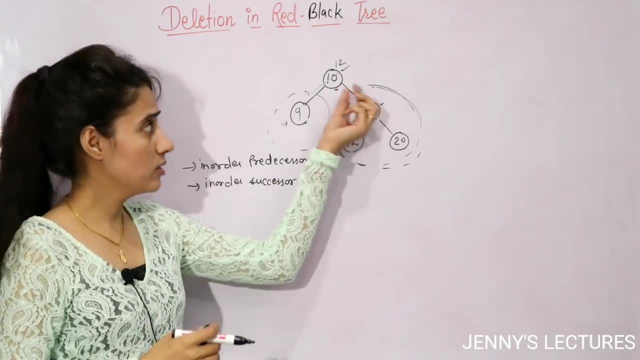 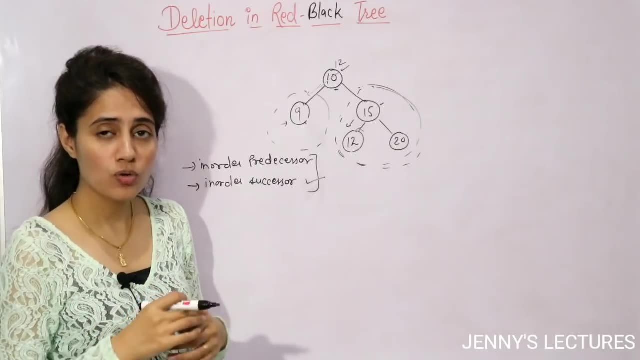 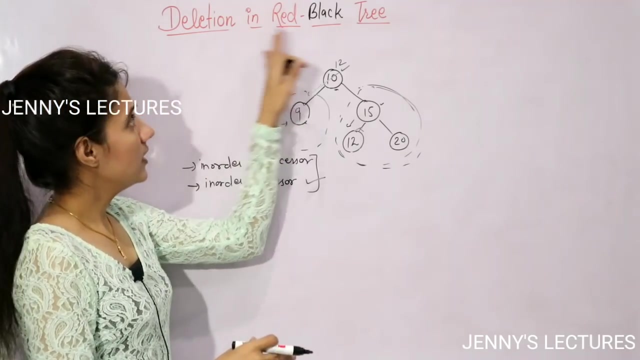 to find this in order- predecessor, successor- and how to replace that node. this thing we have already discussed in detail when we were discussing the bst insertion and deletion, so you can check out that video in the description box as well right now. first step is in this: in this deletion, in. 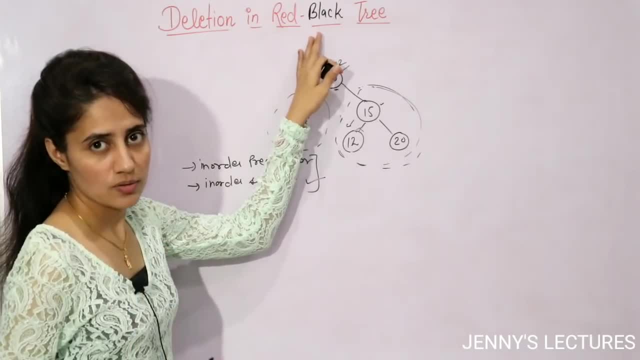 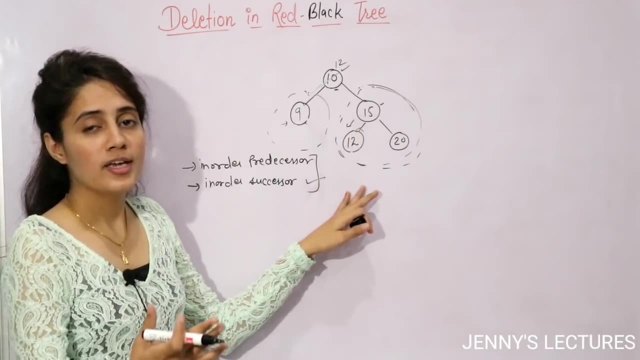 red black pre is what simply performs standard bst deletion, right the same rules here we have discussed. these rules would be followed after that you need to take care of that property, that is, that is not unique like, let's say, if we are talking about a bst problem here, we have to take care of. 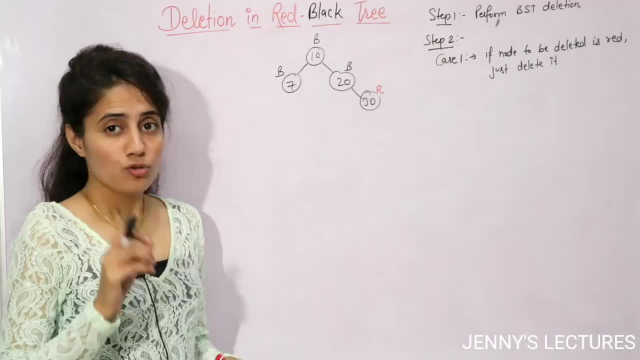 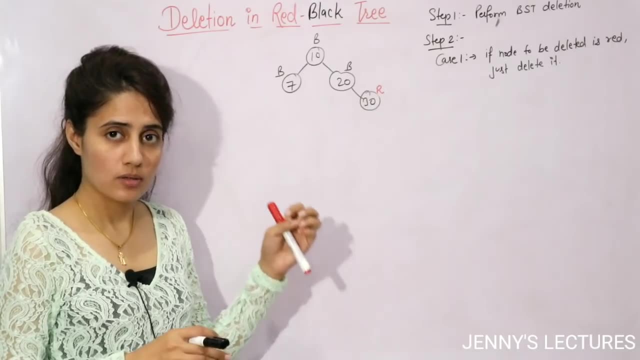 the same rules. after that you need to take care of that property. that is, that is the bst problem: red black property of this tree. so now we will see all the cases one by one, with the help of example, and at last we will also discuss that. we will take example of one red black tree and we 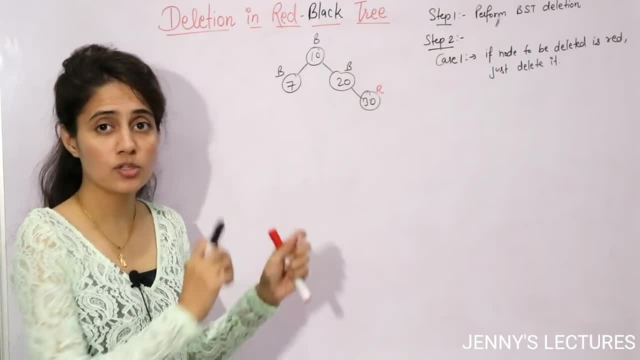 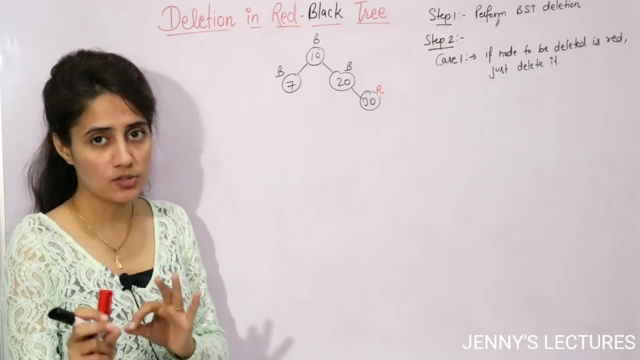 will apply the deletion operation and we will discuss all the cases in one example right now. first step is simply perform bst deletion. so you should know how to perform bst deletion, right? suppose i am taking this is a red black tree. now you can see this is a red black tree because this: 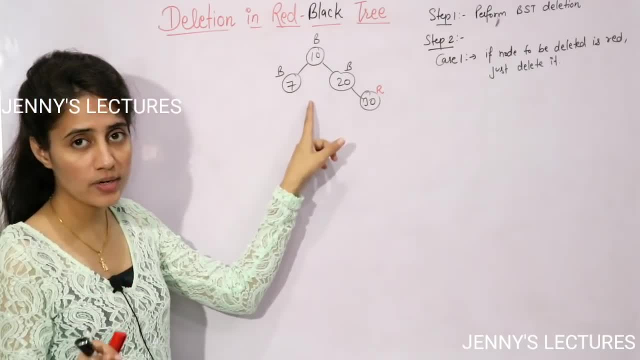 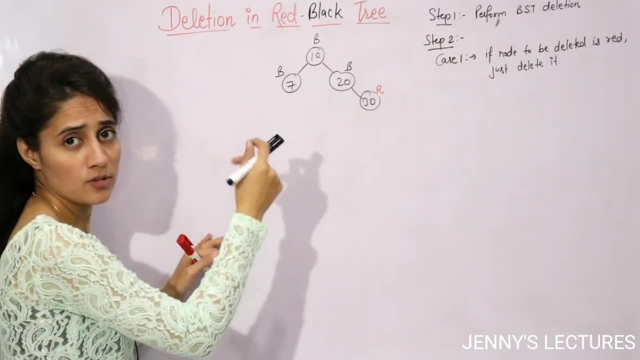 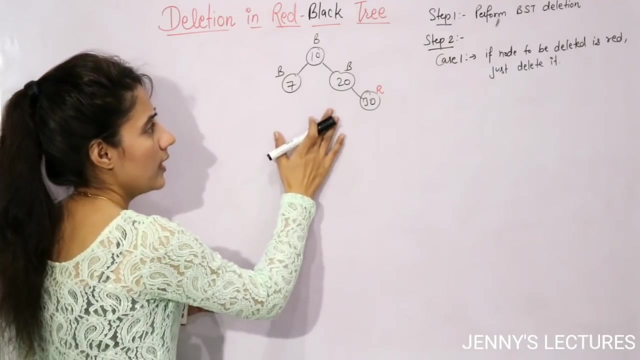 is a binary search tree. first of all, root is black. no red, red conflict is there. and height? you can say that from any node, the path, every path, from the node to its descendant nil, is having same number of black nodes right now. here the case one is: what if the node you want to delete is red? 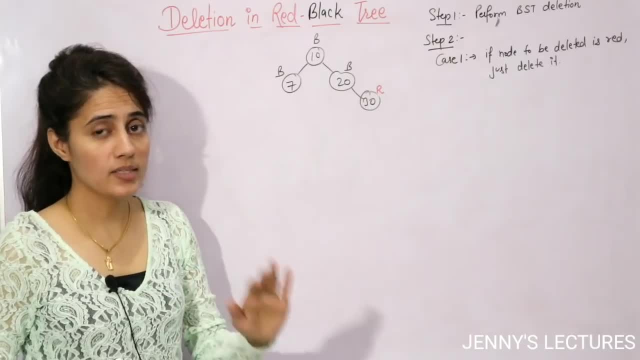 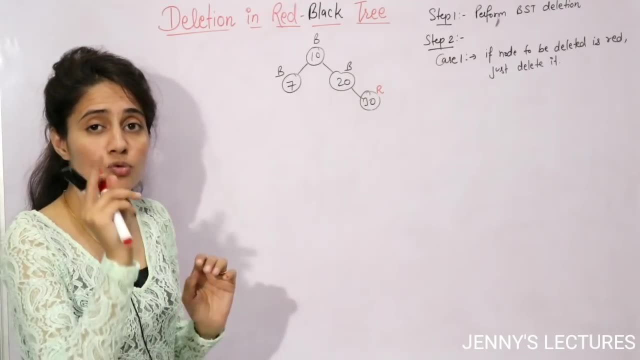 in that case, just delete it. this is the case. one is, what if the node you want to delete is red? in that case, just delete. it is the simplest case in deletion, right? so suppose here i want to delete 30.. now, first step is you need to search where is 30 means binary search. you need to apply here, compare with this root, because 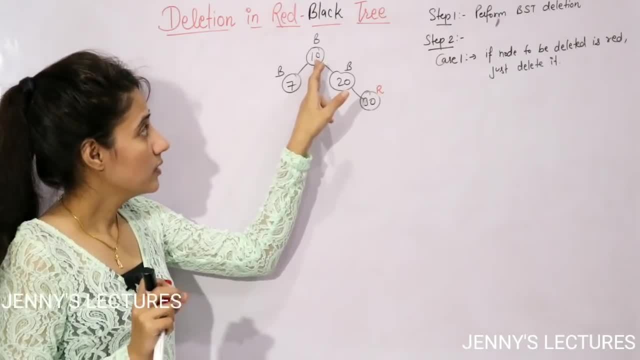 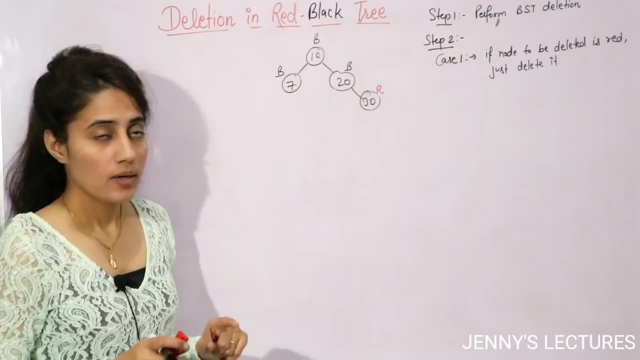 i am having the address of the root node only right. 30 is greater than 10: go to the right side. 30 is greater than 20: go to the right side. here we got 30 right and this node is: this is what leaf node, or here somewhere it is also. 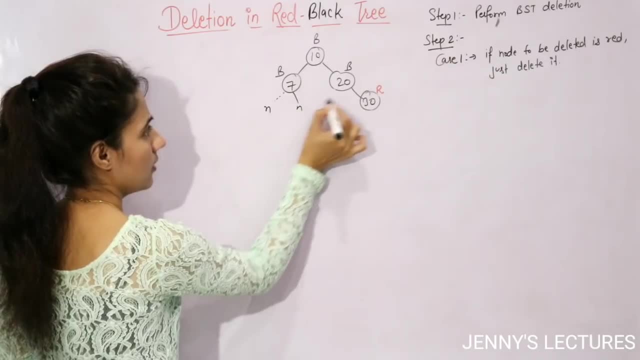 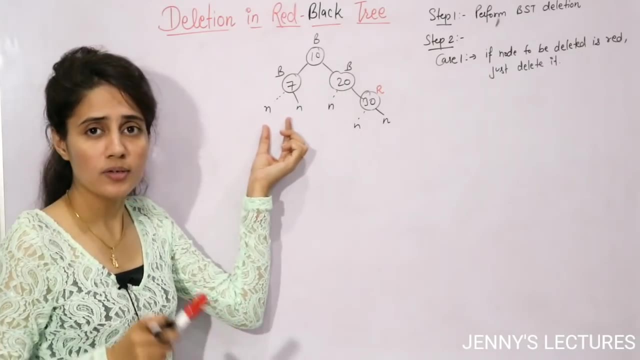 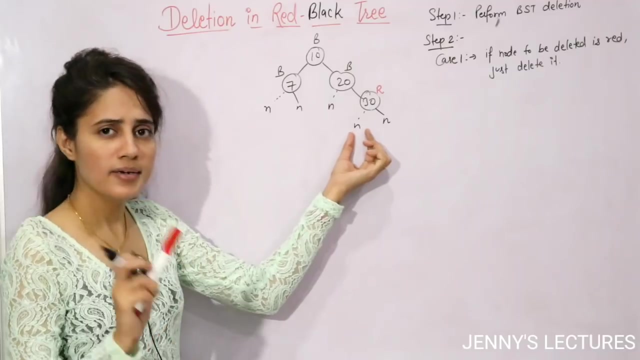 written that because obviously we are. we are having here null, null, here also null, null and null. or you can say nil and all the nil nodes are having color black right now. if you want to delete this 30 and it is having only nil children, no, not null children is there. 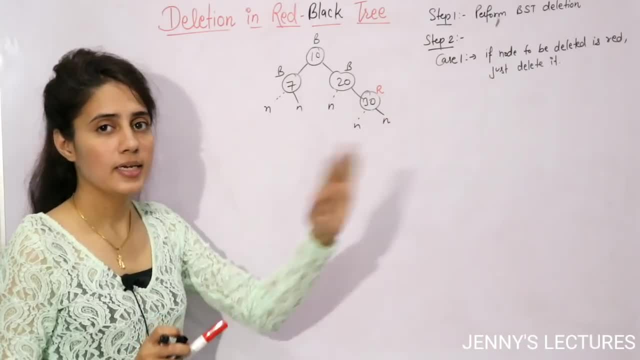 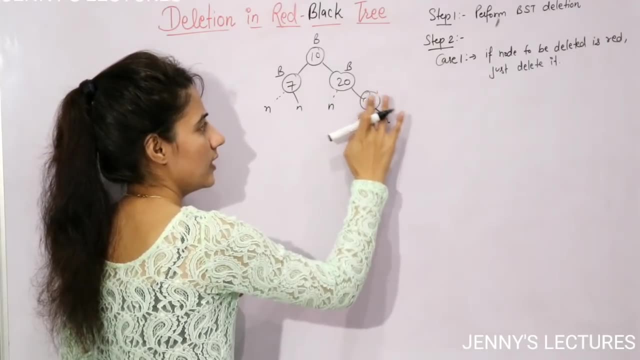 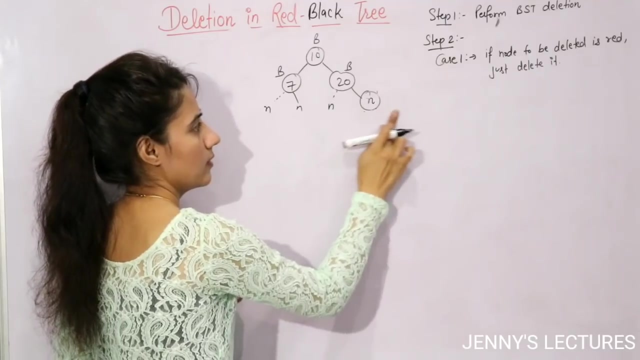 so now, and the red is the color is red, so simply delete it, right? and if you delete it, so here somewhere it is also written that when you delete it, then simply replace it with this: either of its nil: children. so here you can write nil. and this is also in black in color, so you can. 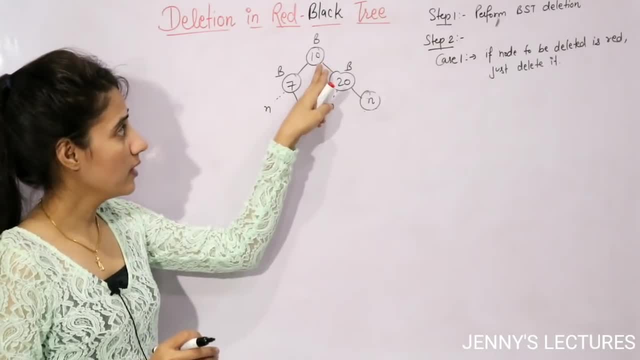 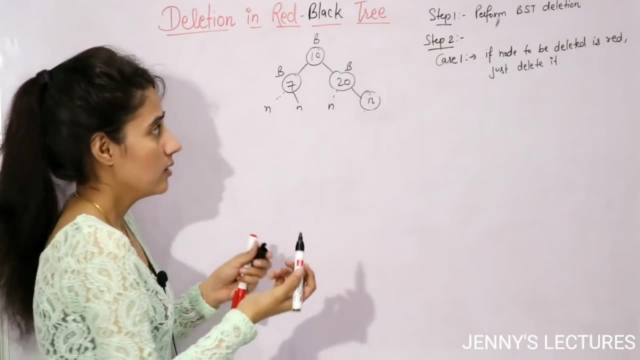 see, it is still a red black tree. right root is black in every path. see here, you can see here we have one and two black node, one and two here also one and two and one and two somewhere. uh, they count that one, two and three. this nil also has a black node, but here i'm not counting this thing, or? 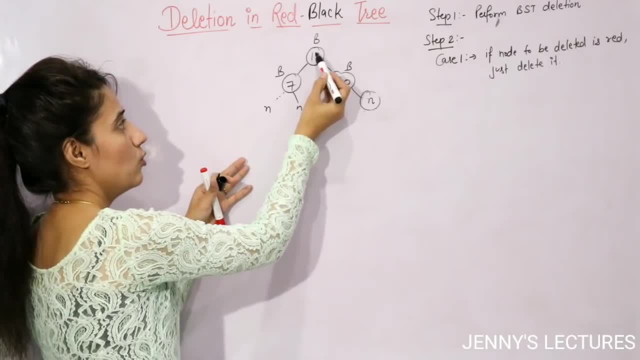 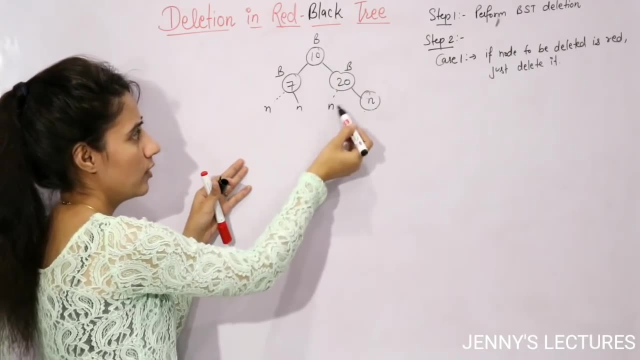 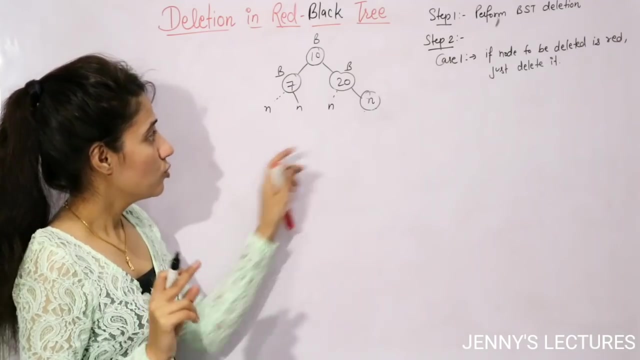 some, somewhere, it is uh counted that they don't count this root in the path because this is always black. so they count this: one, one and two, one and two, one and two and one and two. it's up to you how you you are going to count, but the logic would be uh correct, right? so now the node. 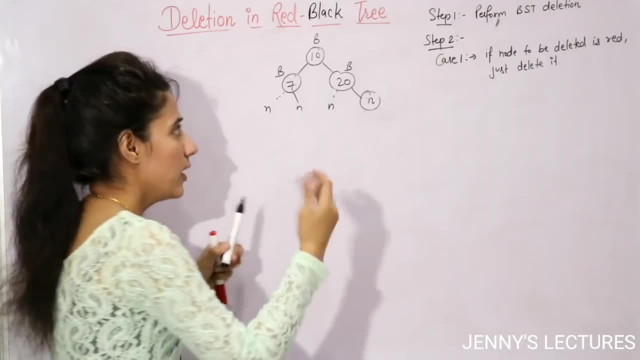 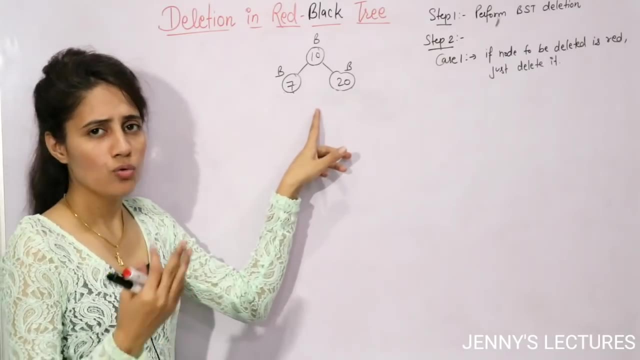 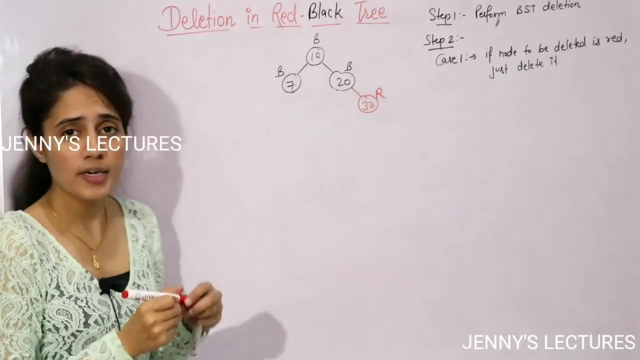 was red, we simply deleted it. no need to do anything. now, here i'm writing simply like this: i'm not writing the null nodes because these are null nodes, so no need to write down those nodes right now. second case is now: suppose here i want to delete 20, now search where is 20 greater than? 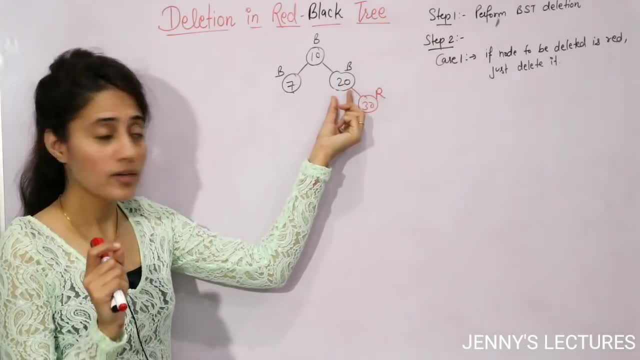 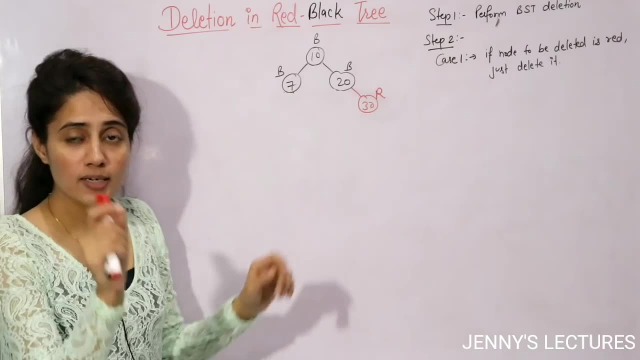 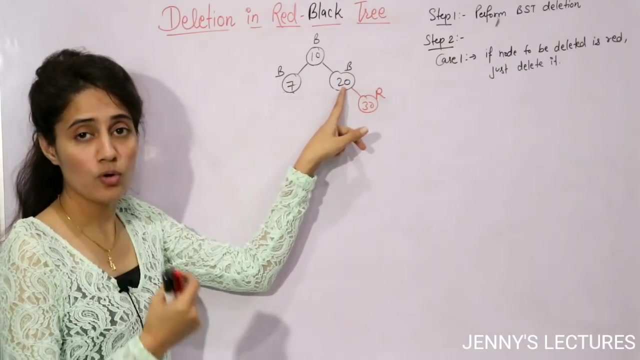 10, so here i got 20. but 20 is what is having one child, so it is internal node. so you cannot delete this 20 internal. we cannot delete internal nodes. we can replace those nodes. so now, with which node you are going to replace this? 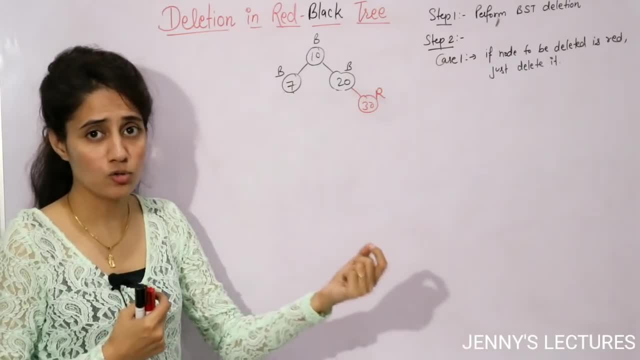 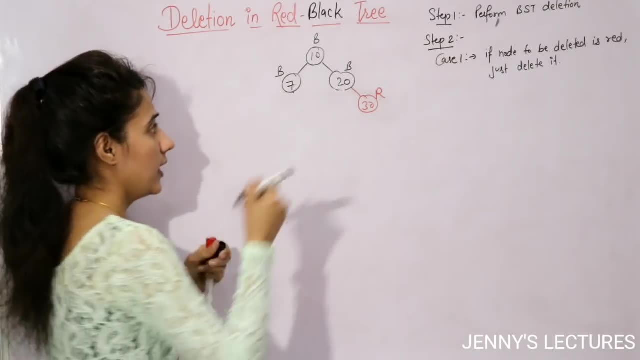 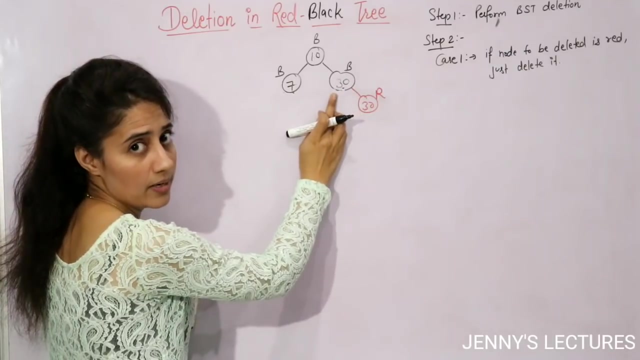 20 because it is having only one child. so just follow the rules of bst deletion. we are going to replace this 20 with this 30. now, here i'm writing 30.. now 30 is red, but here i'm not recoloring it. this is still black. why so? 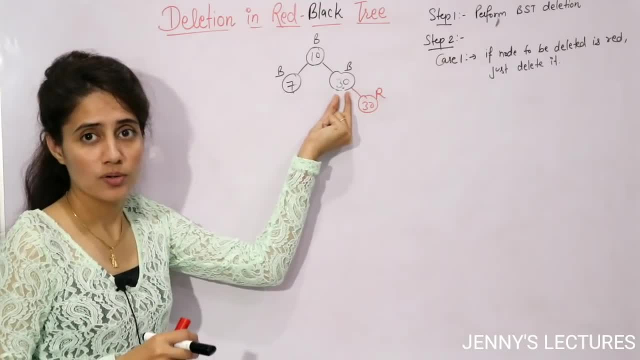 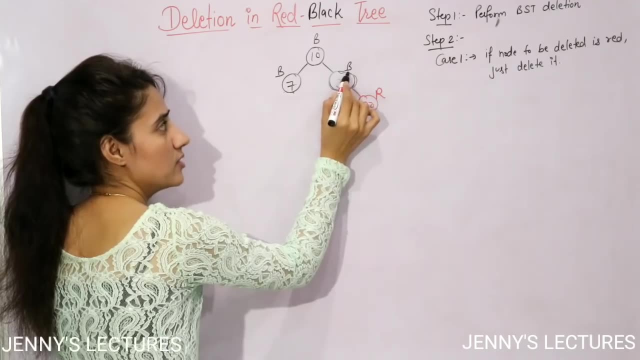 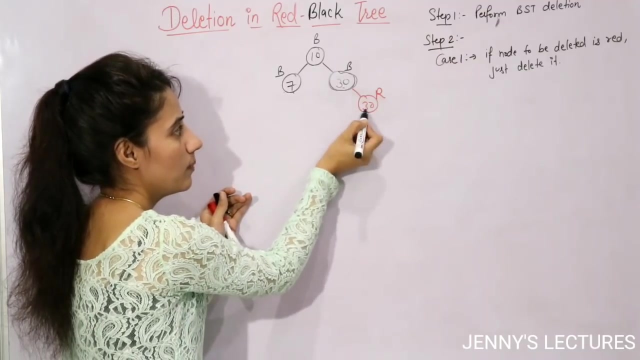 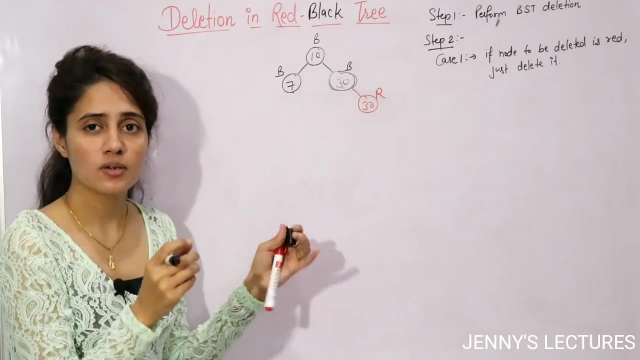 because here we are not going to delete this node. and if you will not delete this node, then this node still having its color black. we are just replacing the value. now, rather than 20 here, we have replaced this 30. we are not deleting this node, so that is why internal node will always preserve its. 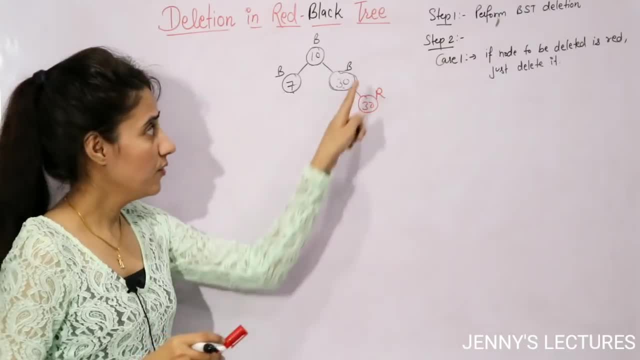 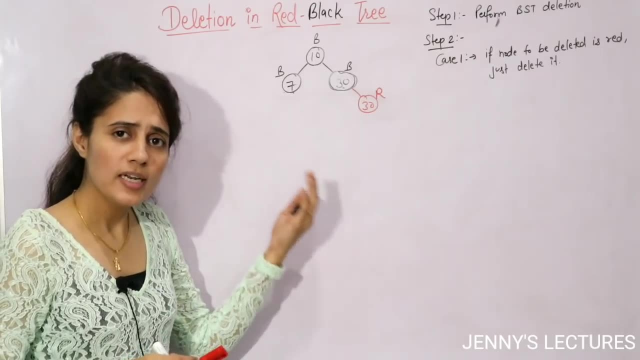 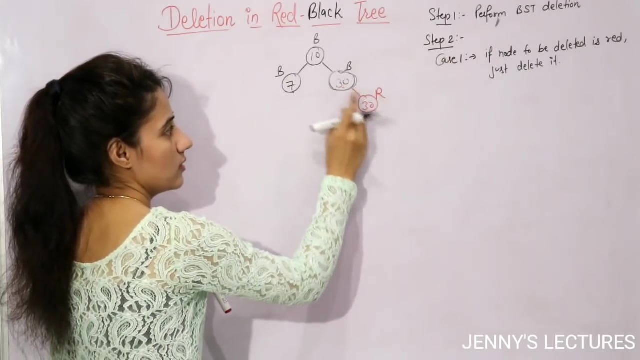 color, its retain its color. if it is black, it would be black. if it is red- internal node is red- it would be red. because the common sense is what if you don't delete any node, then obviously the color of that node would be same. now, right, so we are just replacing this, we are putting this 30 here. 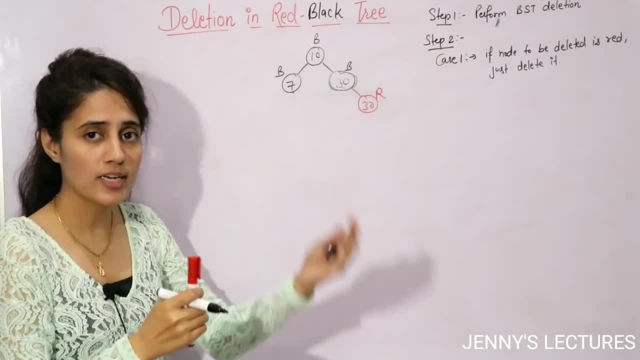 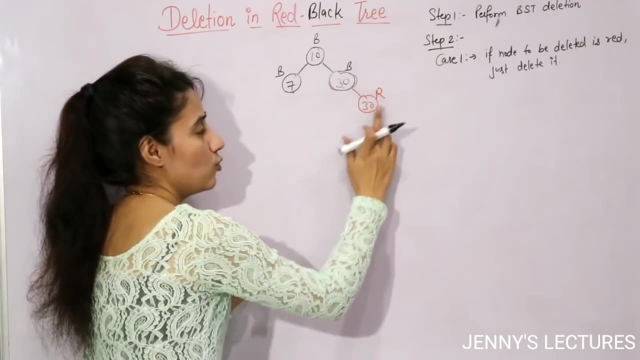 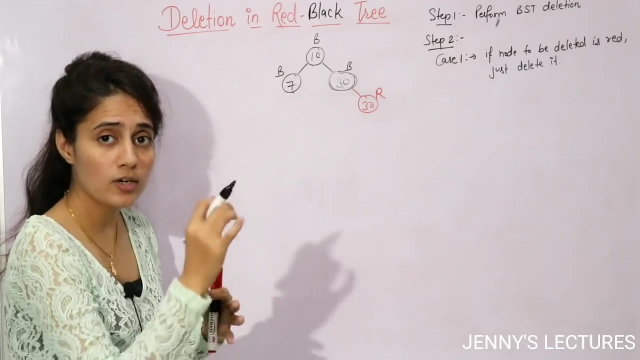 now we have 230 here. now apply that delete function on its in order successor or you can say on the children. right, so now delete this one. this is red. so if the node to be deleted is red, this is leaf node. so we can simply delete it. right, we can delete leaf node. we cannot delete internal nodes. 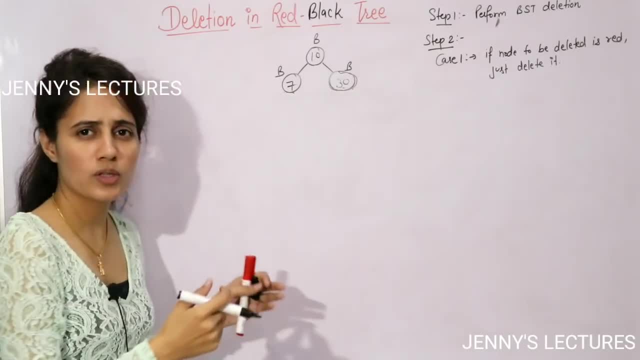 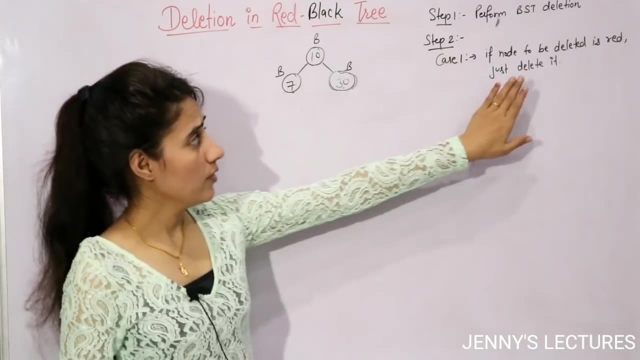 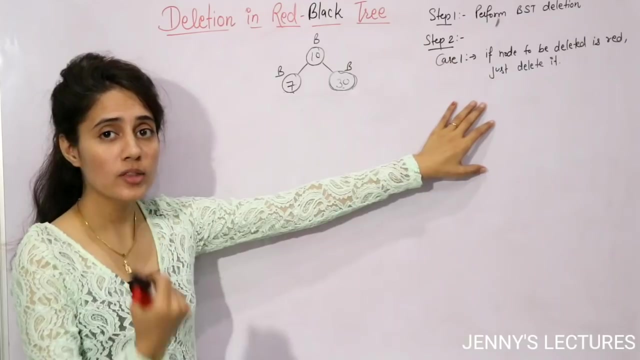 so simply delete it. i'm not replacing this with its nil children, or you can do it something like this here: nildan land nil. so here what you can write: if the node to be deleted is red, then just delete it, and if the node you want to delete is black with one child in color red, then simply. 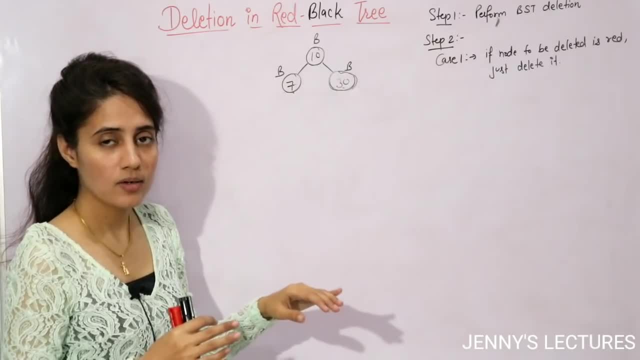 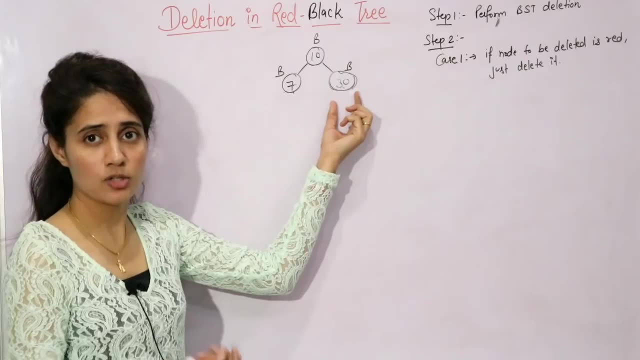 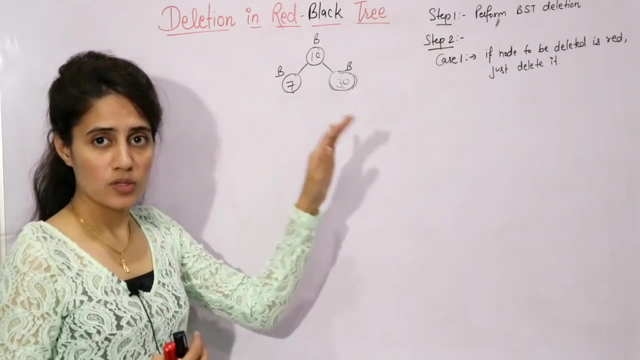 replace that node with its child right and delete that child because child is red. so simply you can that and that node would be having its own color because we are not going to change its color right now. let us take few more example of this case. so here in this example, i want to delete 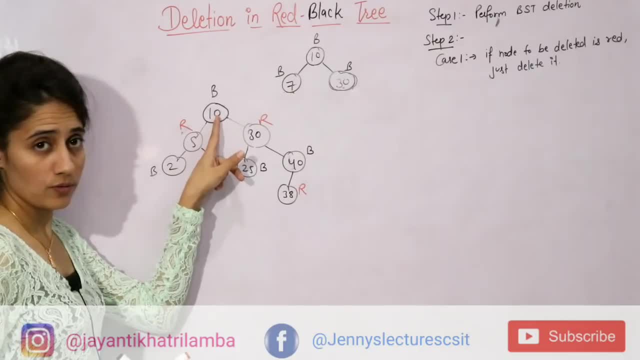 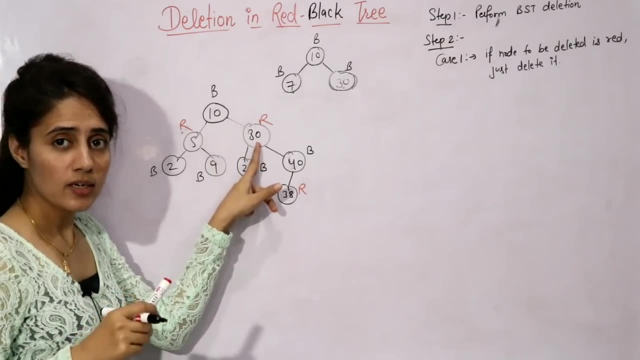 suppose 30. now search where is 30. start from the root. 30 is greater than 10, so go to the right of this root. now here i got 30, but this is what internal node here you can see this is having left and right, both the child. so the case is what? either you can select in order: predecessor. 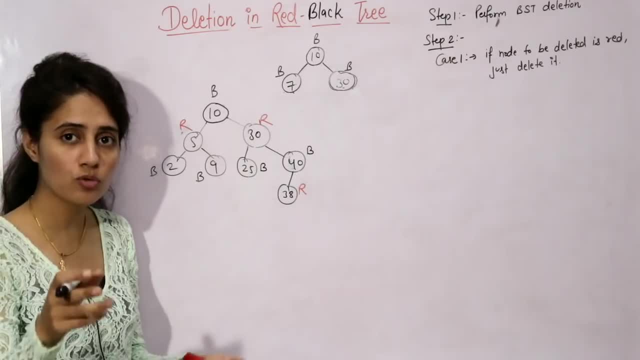 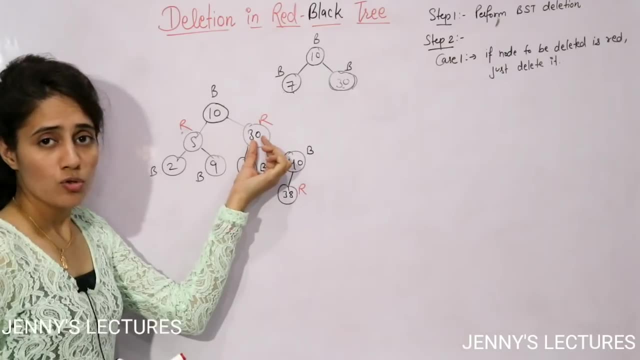 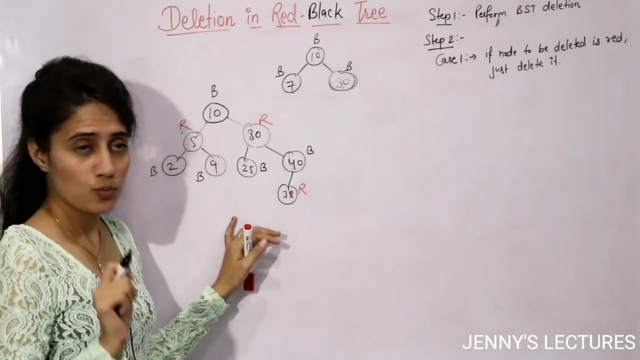 to replace this or in order successor. here i am following the approach where i am going to select in order successor right now. see this: 30 is internal node, so we cannot delete it. you can only replace it. we will delete the def node. this point is very important you need to take care of. 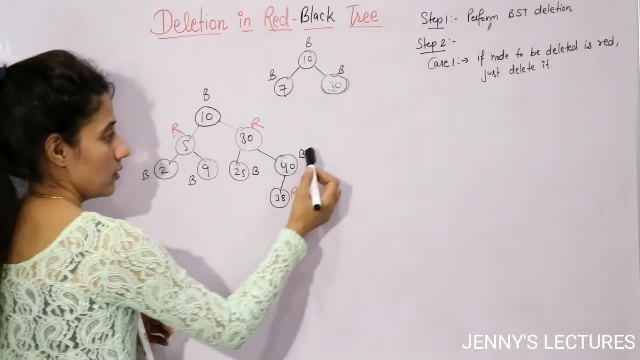 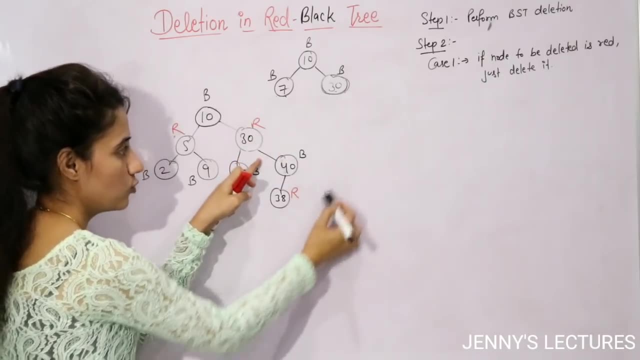 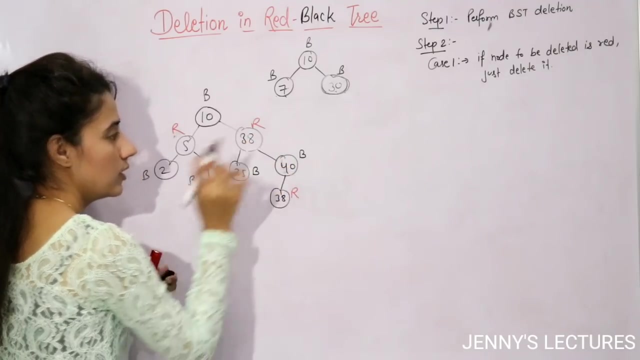 this point. so now the in order successor would be what? the smallest element from the right subtree of that node? because i want to delete this 30. so the right subtree of this node is this: one smallest element is 38, so we will replace this with this. 38 means rather than 30. here you will write 38, but the color would: 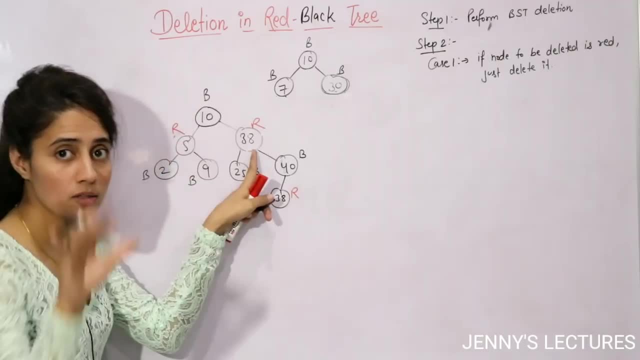 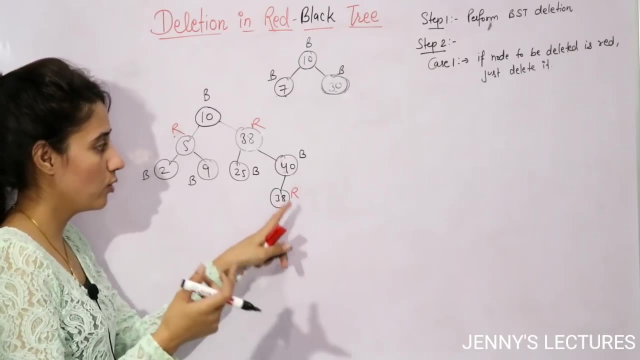 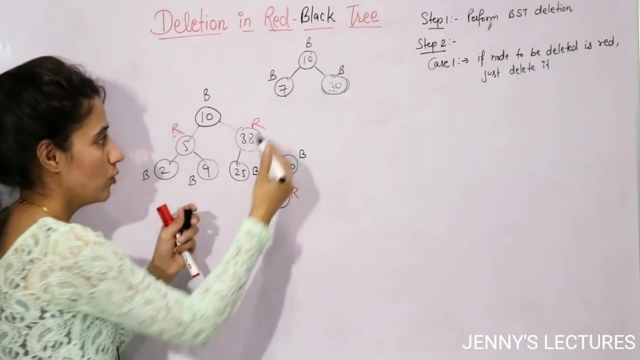 be same. see, it is internal node. you are not going to delete the node. that is why the color would be as it is. if 30, it's not like that, if 38 is black or it's red, then you are going to take the color of 38 only. no, the internal node will having its own color, so we are not going to change its color. 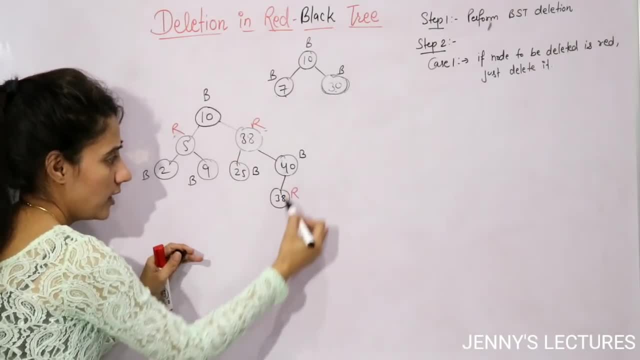 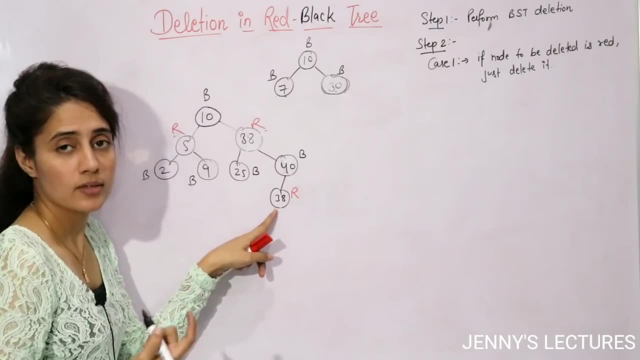 that would be red. only now that on that in order, successor. now we are going to call recursively that delete function here. now can you delete this 38? yes, obviously it is the leaf node and it is red. so simply delete it. you know no need to do. 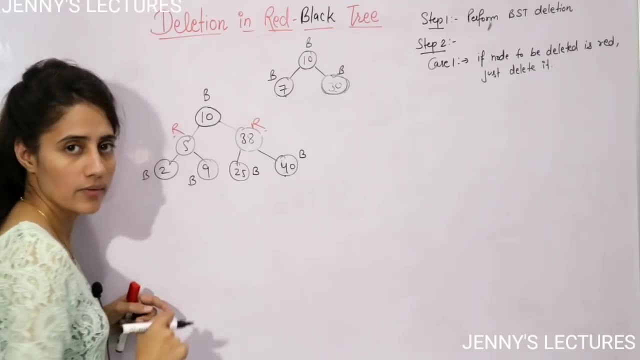 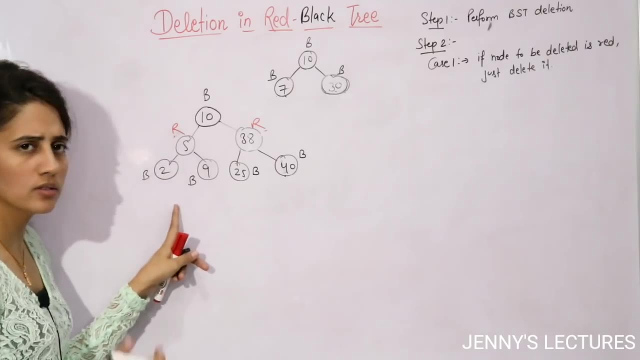 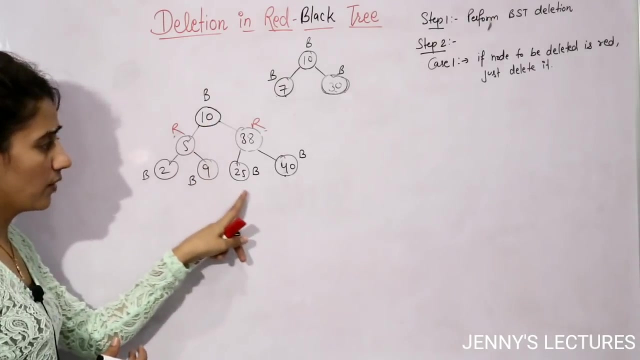 anything, so you can simply delete it, right. or you can say: here we will replace the 38 with its nil children. so nil is black. each node is having its nil children, right. as you can see, this is still a red black tree. no red red conflicted is there in each path we are. 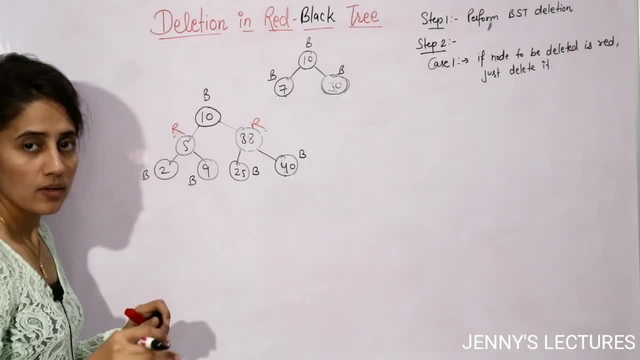 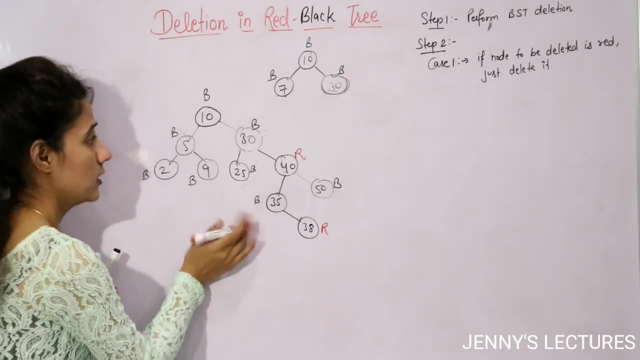 having same number of black nodes and root is black. right, let us take another example now. let us take this example here also. see, this is a red black tree. you can check out all the properties now. here also, i want to delete this 30. first of all, search where is 30. it is greater than 10, so 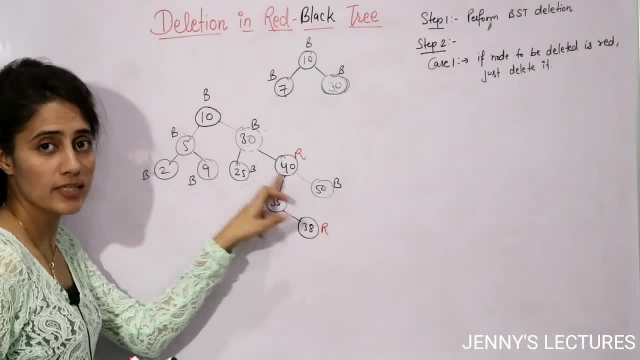 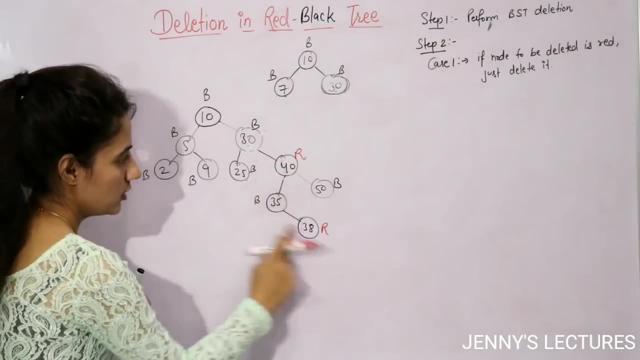 here i got 30. now it is having two children. now i will replace it with its in order successor. in order successor is what: from the right subtree of this 30, find out the smallest element. smallest element from this is what? 35 right, so now i will replace it with its in order successor. in order. 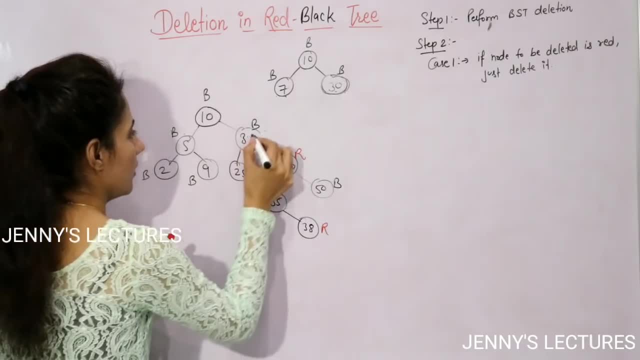 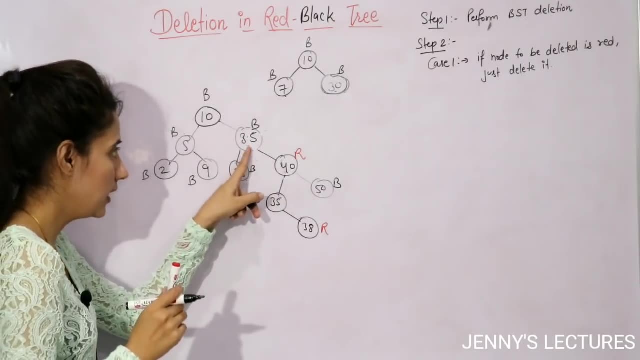 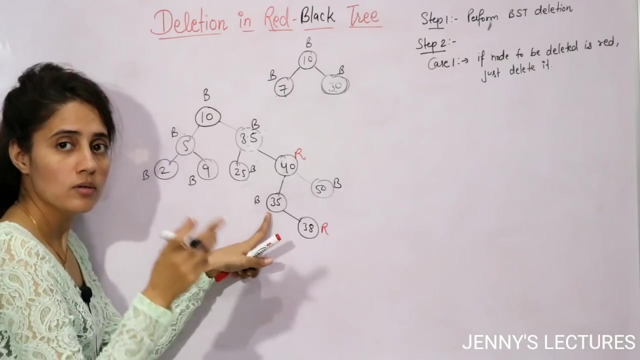 here you will write 35, 35, right, and it will. it is black, so it is going to contain its own color, right, because it is internal node. we will not delete internal node now. the problem is we have 235 now on that in order successor, call the delete function recursively now. now you want to delete? 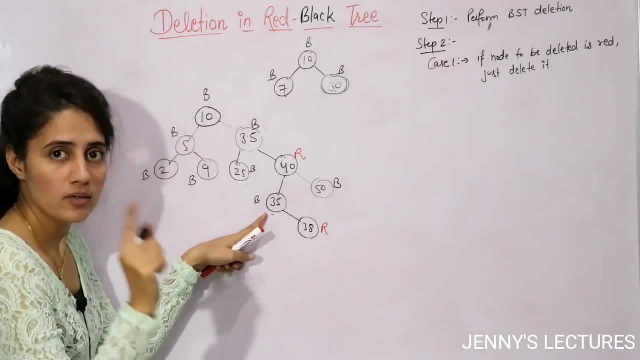 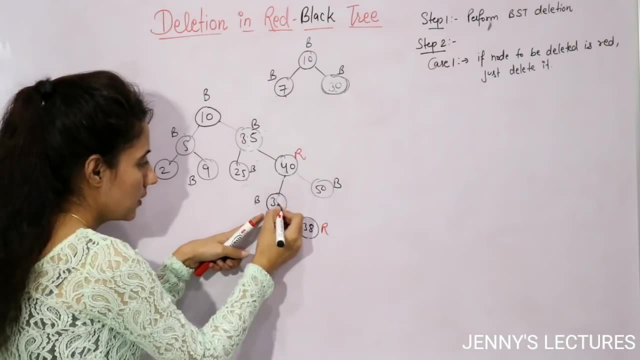 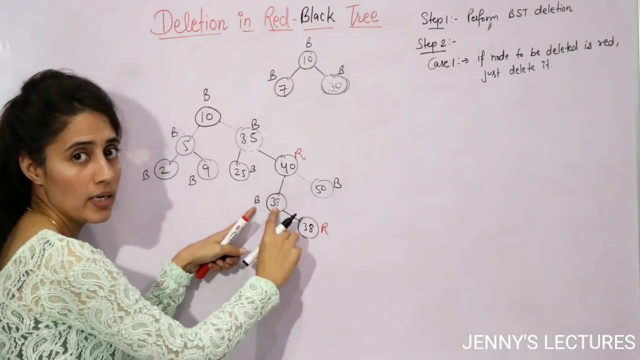 this one, right, but this is still having one child, right, so we will not delete this. we will replace this. so here we will write 28 and it will contain its own color, right? it is not like that 38 is red, so we are going to make it red. no, it is internal node. we will not delete this, so it is having its own color now. 38. 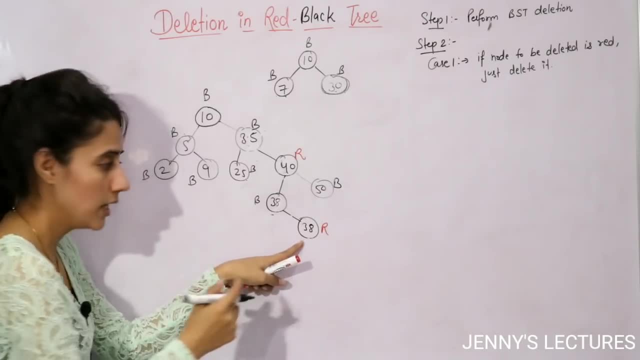 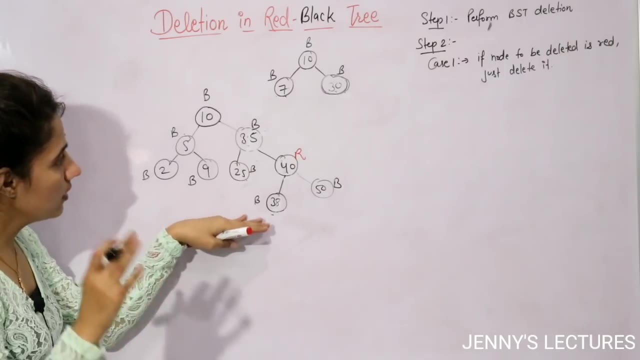 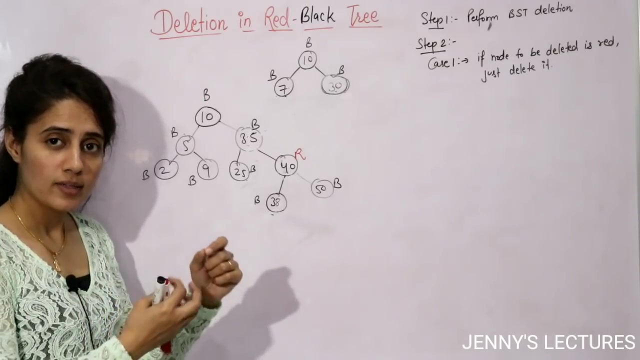 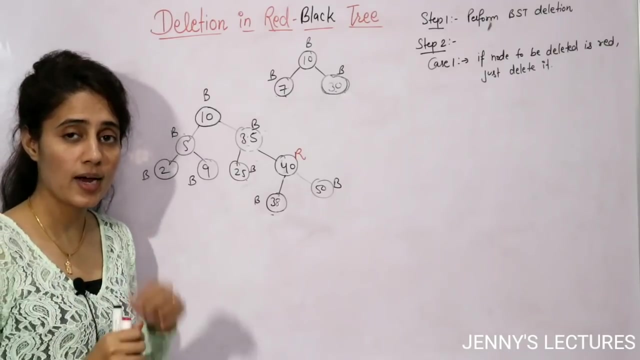 38, now again recursively called a delete function on this 38. now it is red, so simply delete it, right. so, as you can see, this is still a red black tree, right so now the problem comes when you will delete a black tree node and that black node is having black children, right so there a double black situation will arise. 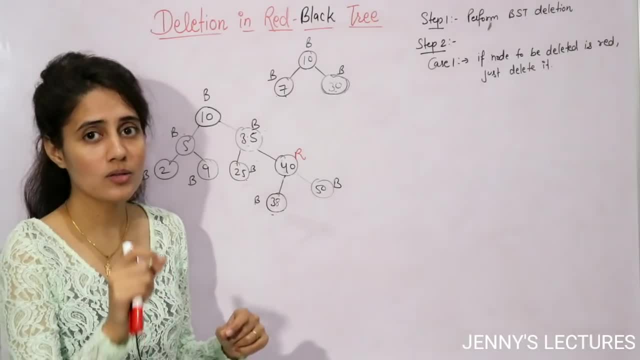 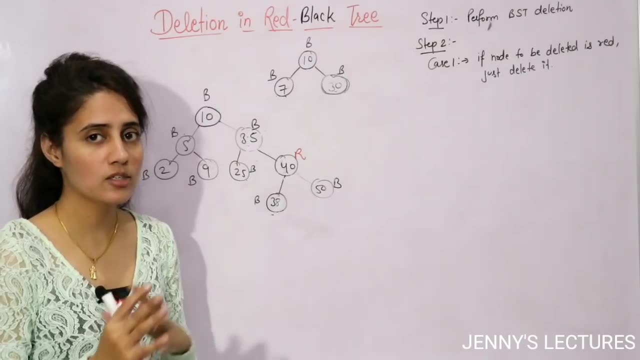 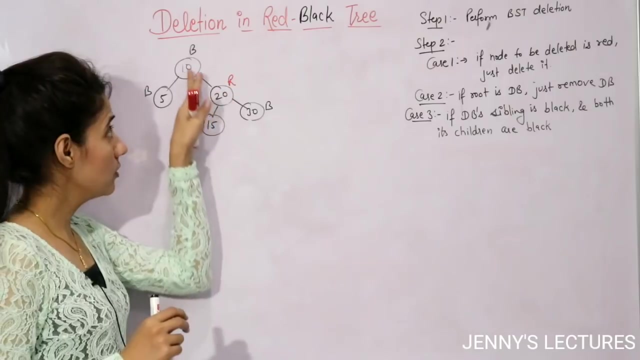 and the main task here is what you need to convert that double black into single black, and for that you need to have some cases. so we'll discuss all the cases with the help of example now. now suppose here i want to delete this 20 right. first of all, search where is 20 to the right of this 10? it is. 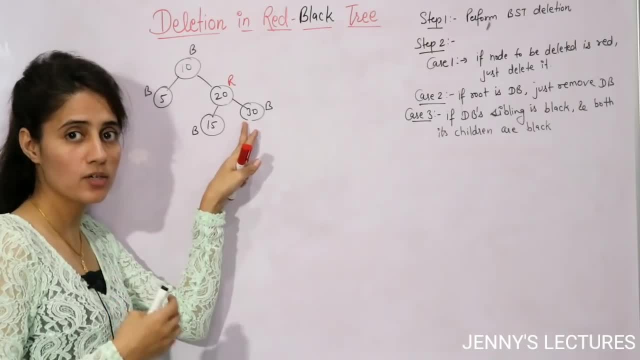 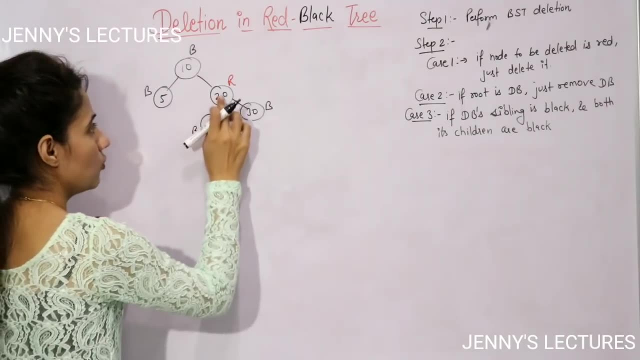 having two children. so which, with which children, you are going to replace it with? in order, successor from the right subtree. find out the minimum element in the right subtree. we have only 30, so we are going to replace it with 30, right, and we are not deleting this one, so we are just replacing. 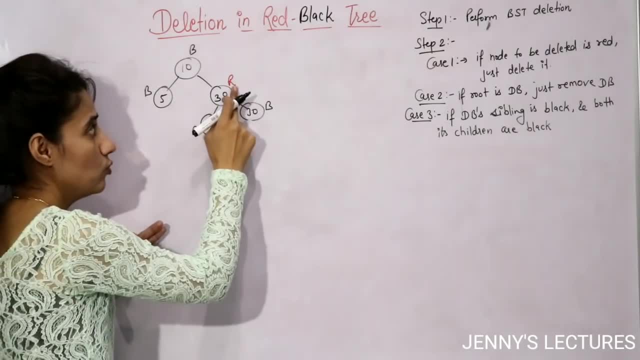 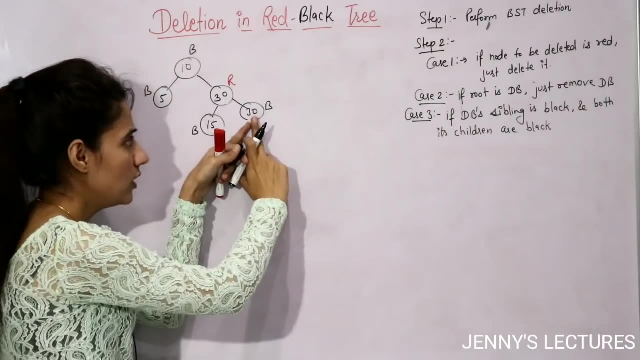 it, so it will contain its own color, right, we are not going to affect this color. now again, call delete function on its in order successor. now, if you delete this 30, obviously this leaf node, so you can delete it. you can delete it. you can delete it. 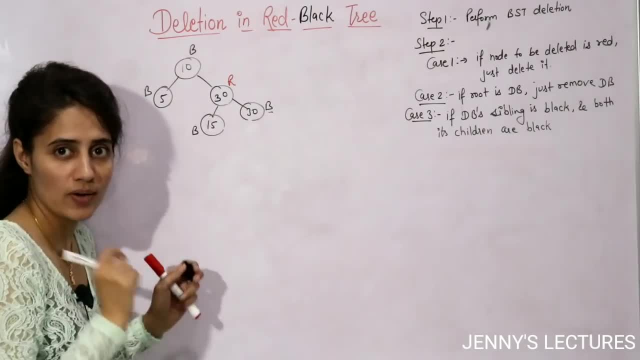 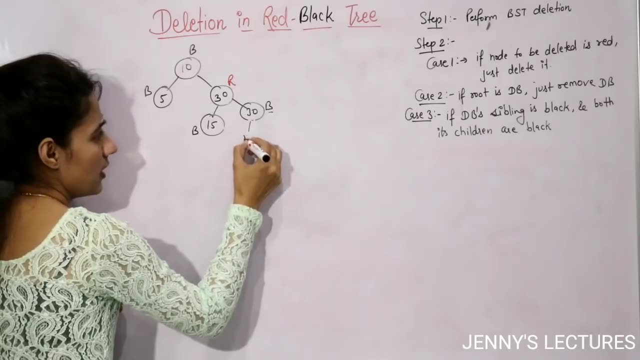 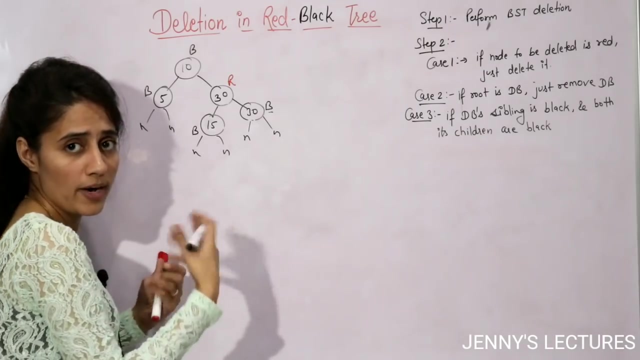 but here the situation is what: it is black, it is not red. so it's not like that. you simply delete it. no, why so? because see, this is having nil nil. all are having its nil children, and these nil are black. so, by default, if this is red, what we have done- we simply replace it with its nil. 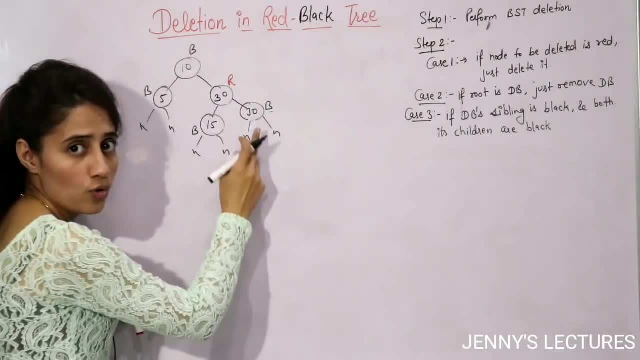 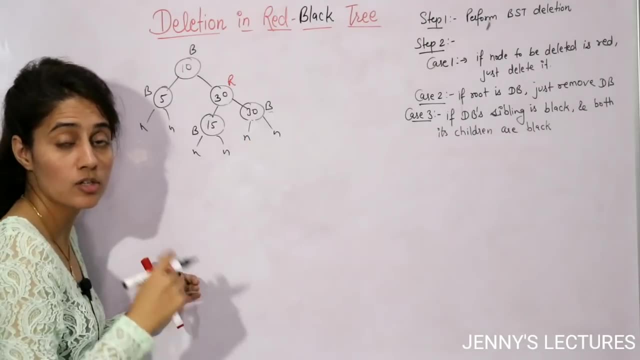 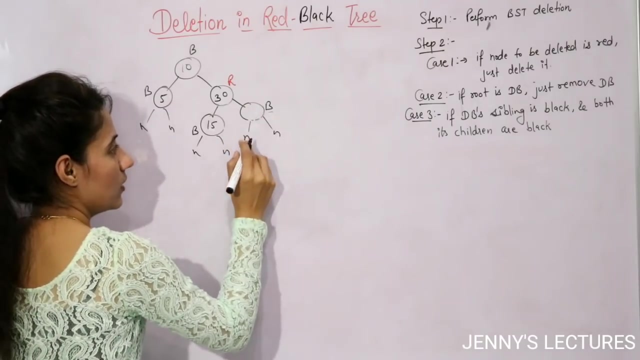 children, but here this is black. you want to delete this node. this is black and you will replace it with its nil children and the nil children is also black. so now this is situation of double black. so if you delete this and you will replace it with its nil, so its own color was black and the children 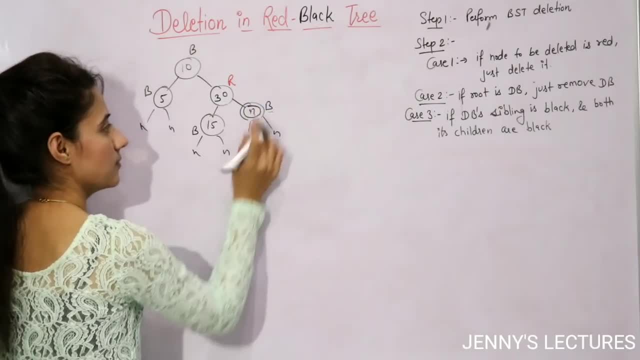 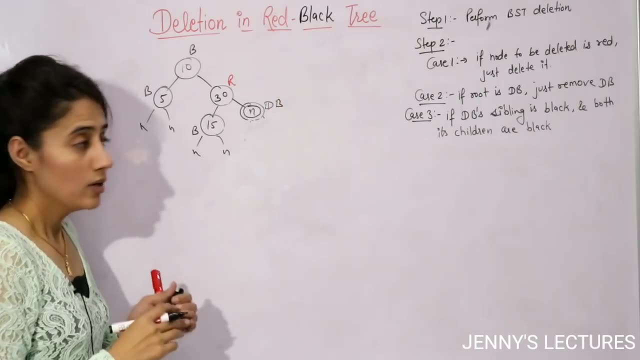 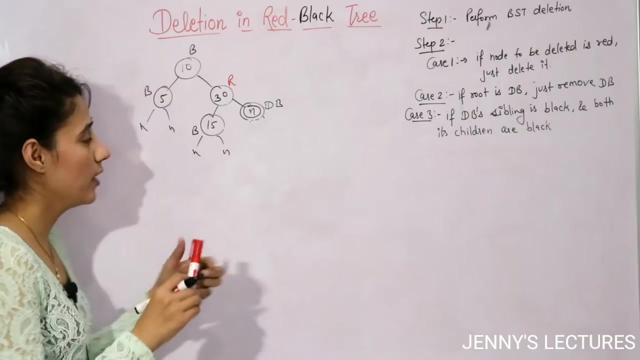 color is also black, so it is now double black. this is the case now, or you can say it is now db double black node. you need to take care of this node now. this is the main problem in deletion in red black train. now you need to convert it into single black. why? so see now check out in each path here. 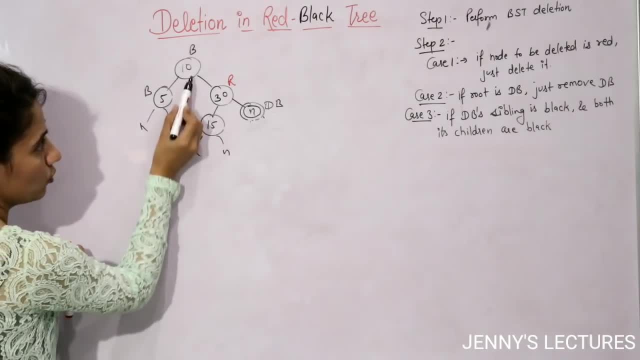 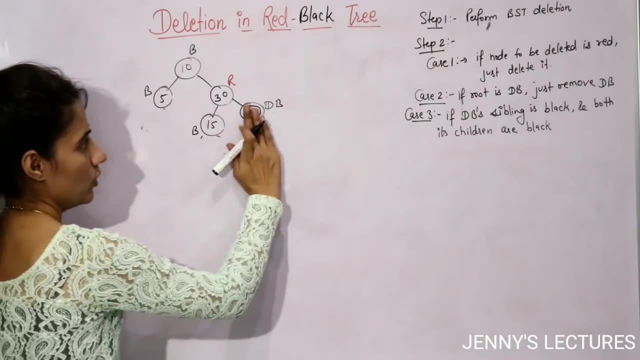 we have two black nodes. here also we have two black nodes, but here we have only one black node because we obviously we are not going to count this nil node, so you will not count this nil node. so in this path from here to this nil node, we have only one black node. 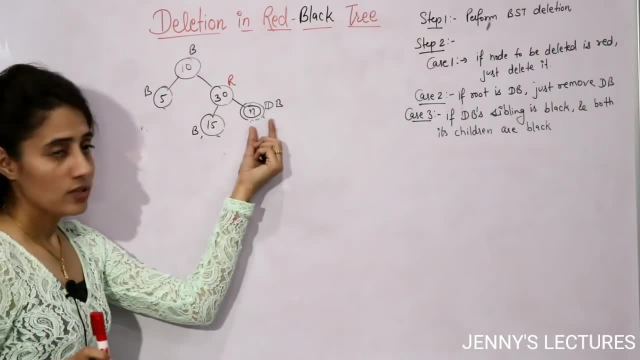 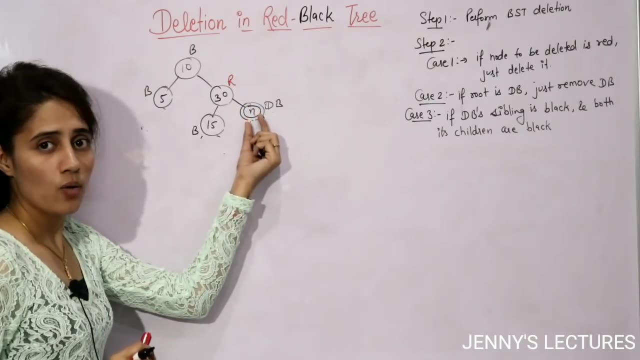 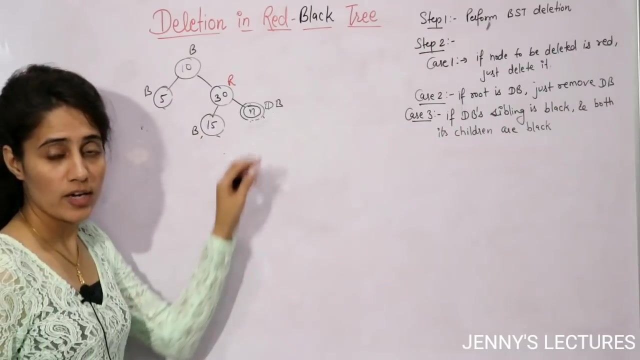 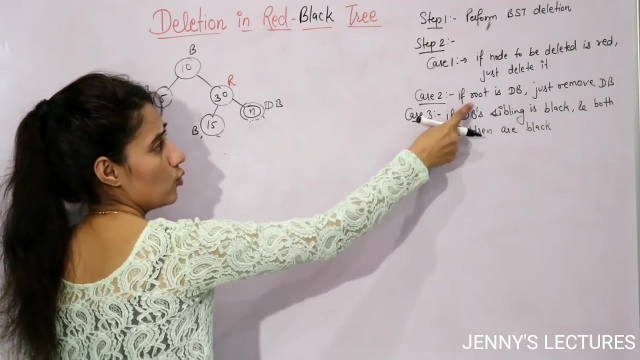 so the main property which is violated here is what? because of deletion of black node in this path, we have one less black node, so it has it has affected the black height. now you need to take care of this thing now. so here we have multiple cases right now. see. first case is simple: if the 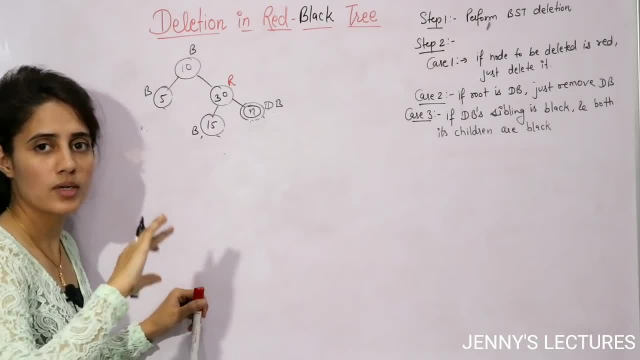 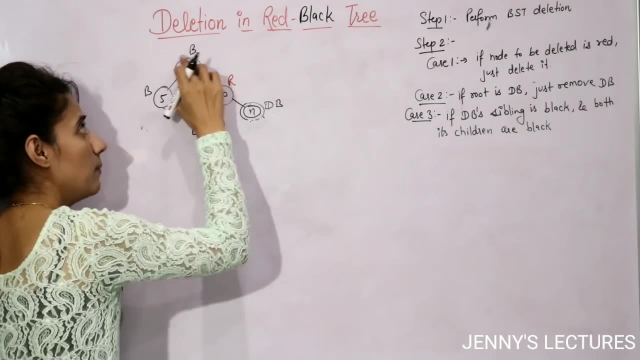 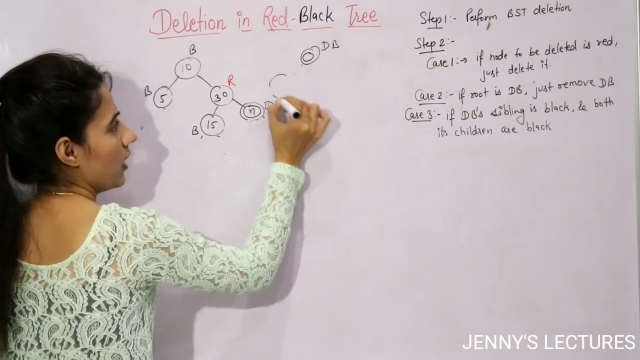 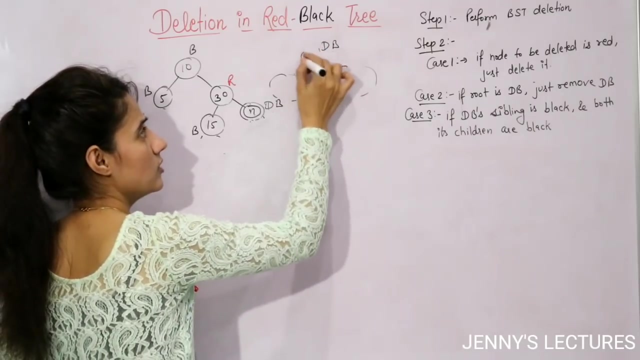 root is double black, so simply remove double black right. suppose because of some situations you got double black at the root, right. this is root, this is double black. and here we have left subtree and here we have right subtree, right. no need to do anything, simply remove this double. 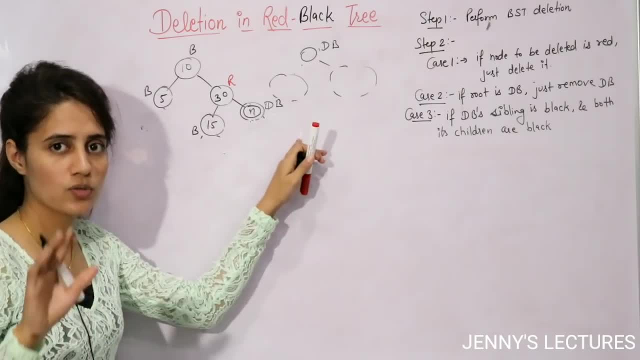 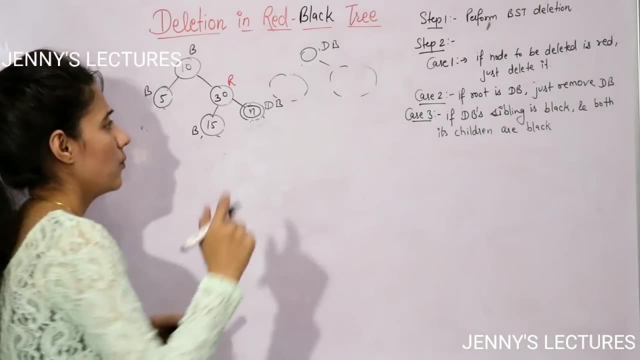 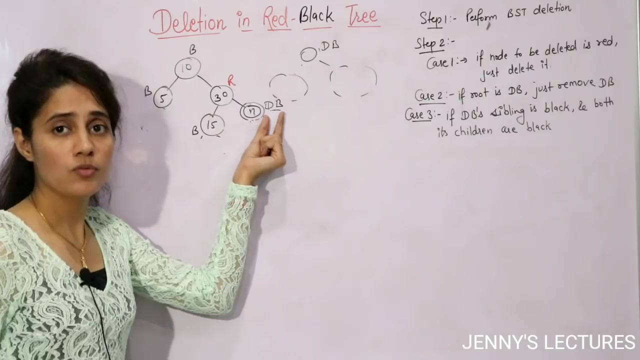 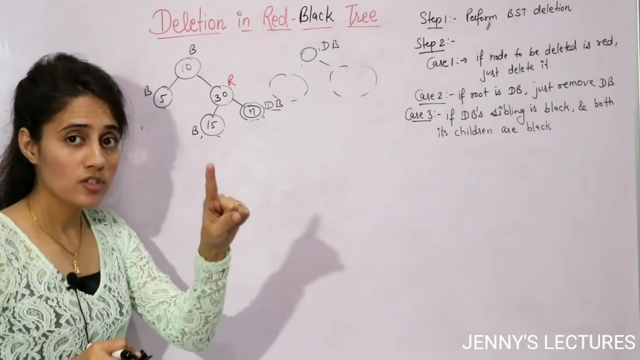 black and make it single black, right. this situation we will discuss with the help of example. this is the simplest way to do it. case in this scenario, right. next situation is what now if the node is double black, right, so to resolve this conflict, we will always check its sibling right. see, in case of insertion we have 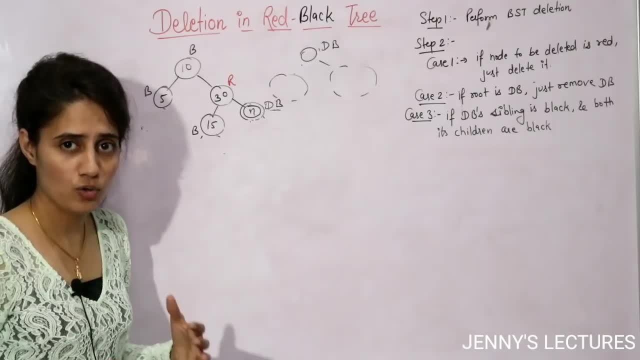 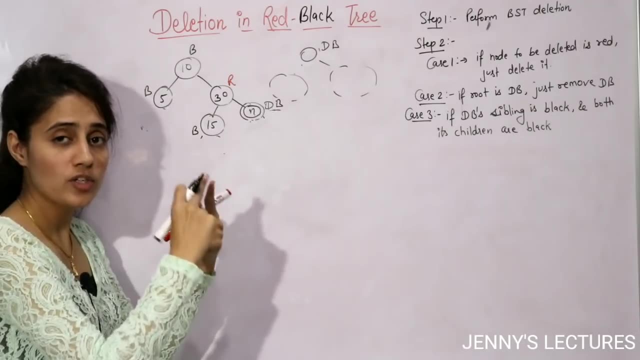 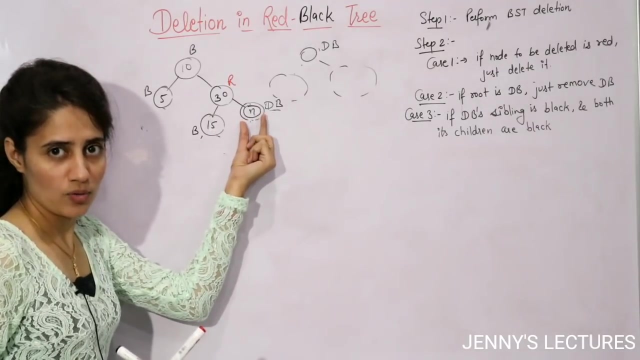 checked the uncle of that node, right, i guess you remember, or you can say that parents sibling. according to that we decided which rotation or which case you need to follow. but here we will check the sibling of that double black node and according to that we will decide which case you are going to apply. 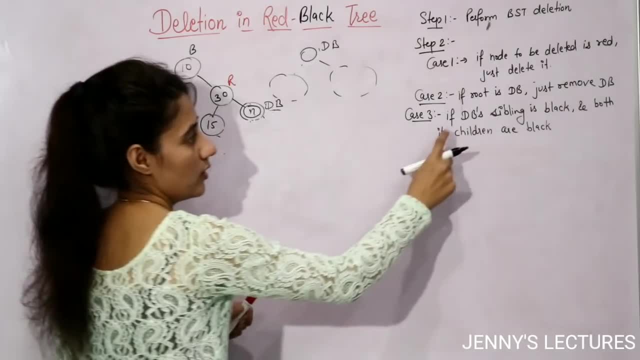 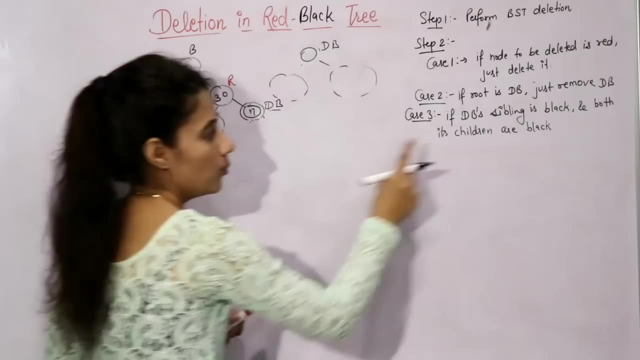 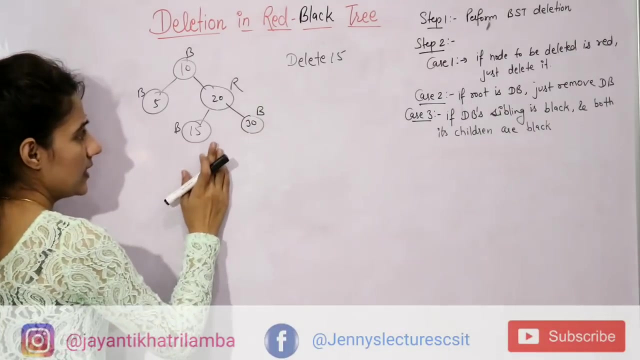 right now. first case in this case in this is: what if the double black nodes sibling is black and both its children are also black? so let us take that example. so now let us take this example. here. in this example, this is a red black tree and here i want to delete this from here. i want 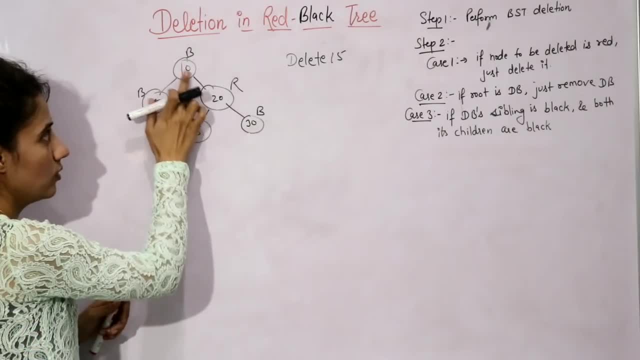 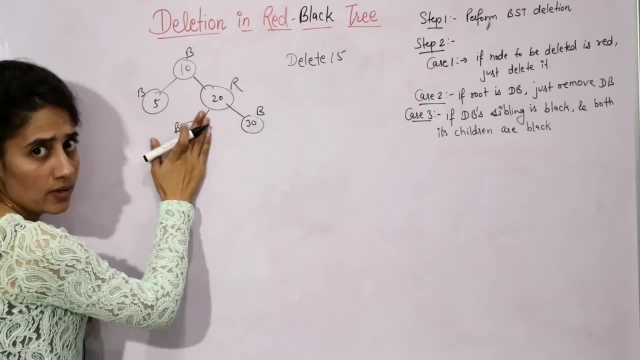 to delete 15, right. so search where is 15? to the right of this 10, to the left of this 20. here we got 15. now see, we cannot simply delete this 15. it is a leaf node and you cannot delete it like this, because 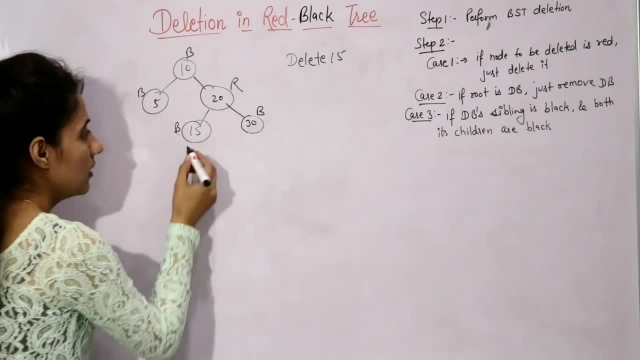 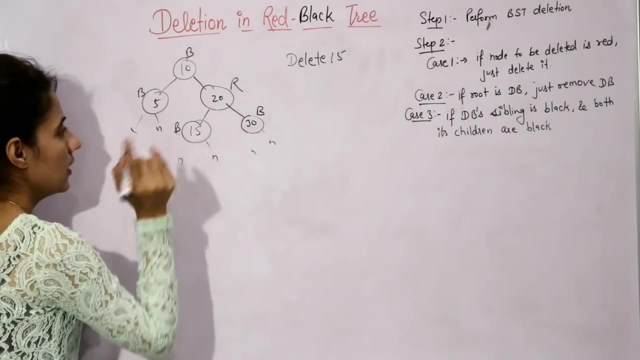 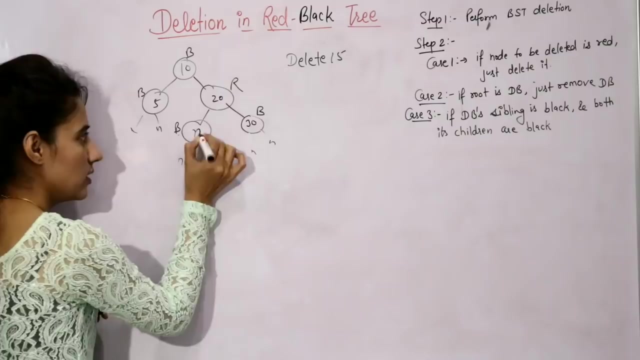 it is having color black. if it is red, then you can delete it. it is having two nil children, which are also black. this is also having nil, nil, nil and nil. uh, so we have different project left and right and if you will delete this one, then you will replace this with its children- one of its children, that is. 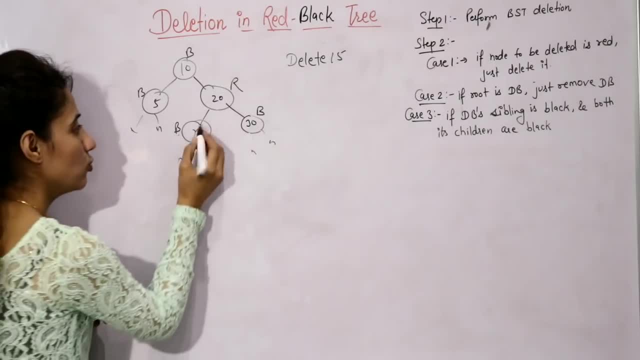 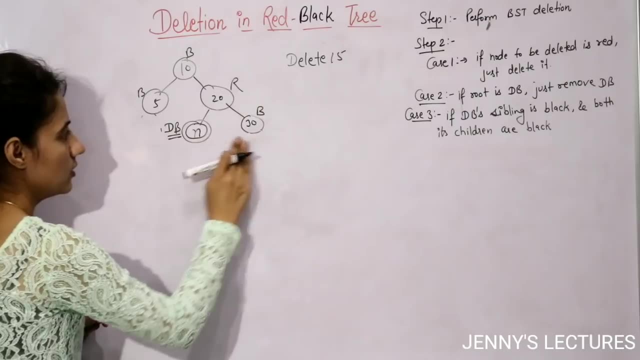 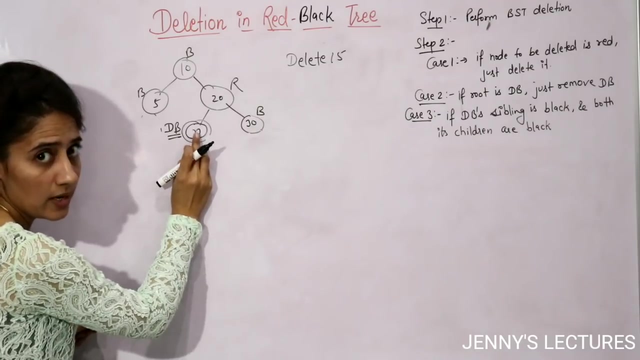 nil and this is black and the children color is also black. so this is now you can say double black, db. right, i'm not showing these nil children, so now in this path from here to here, because obviously we are not going to count this nil while we are counting the black node in the path. so it 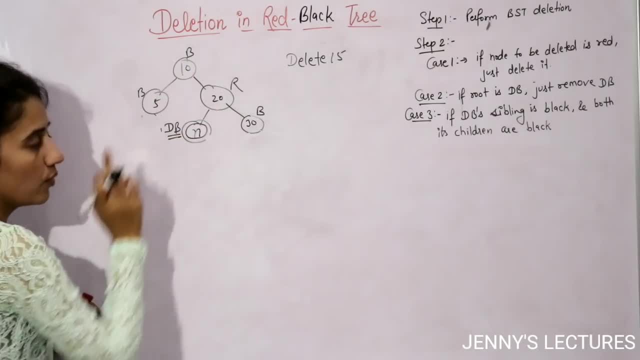 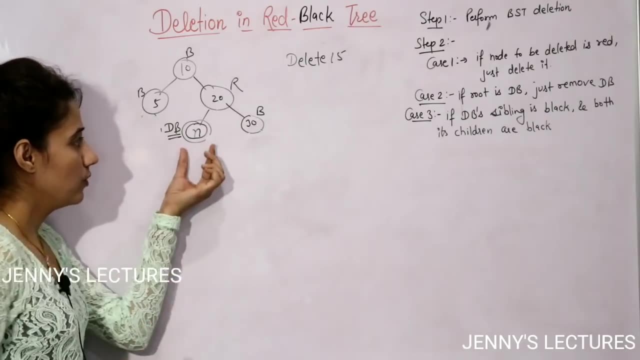 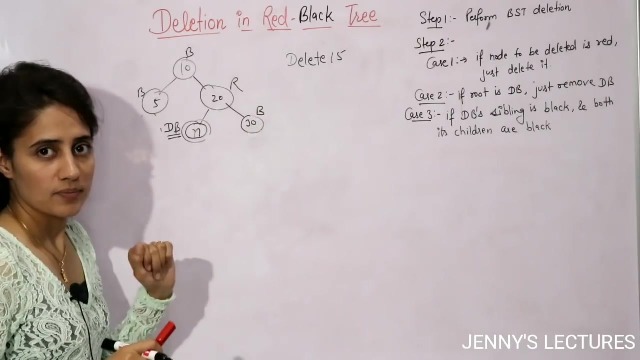 is having only one black node. here we have one and two, here we have one and two. so now we need to solve this problem. now, to solve this problem, this double black node will always check its sibling. sibling is 30. check the color of sibling: it is black right and sibling children are two. 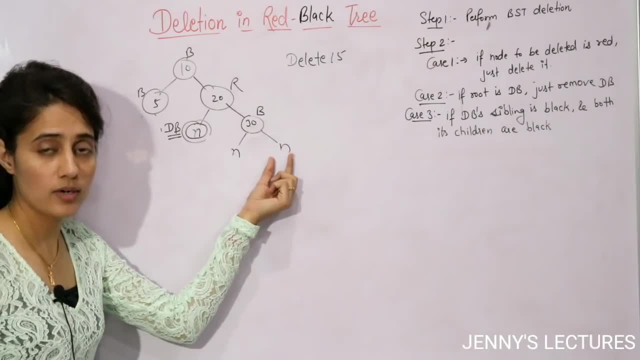 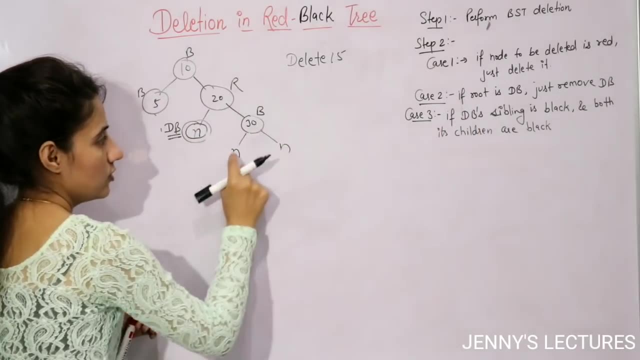 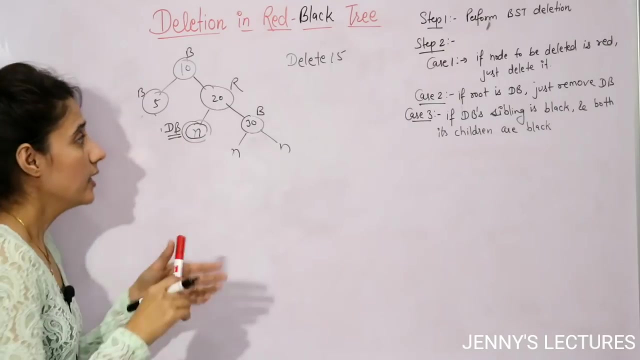 nil and nil, and color of nil, uh children, is also black, as we know right. so now, db's sibling is black and both its children are black. so this is the situation now. now what this db will do see here. you can, uh, relate it with this example: that red means if someone is angry, then 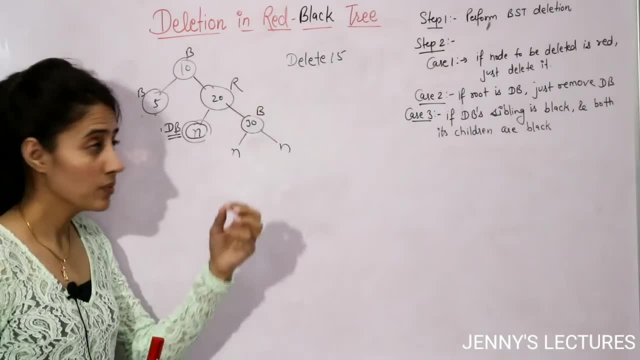 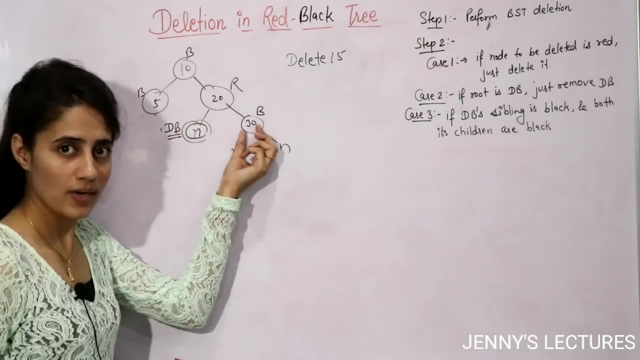 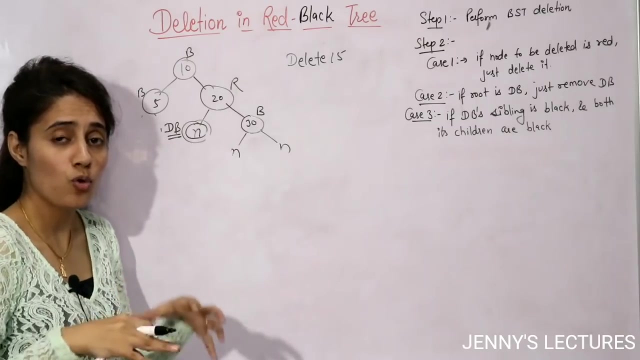 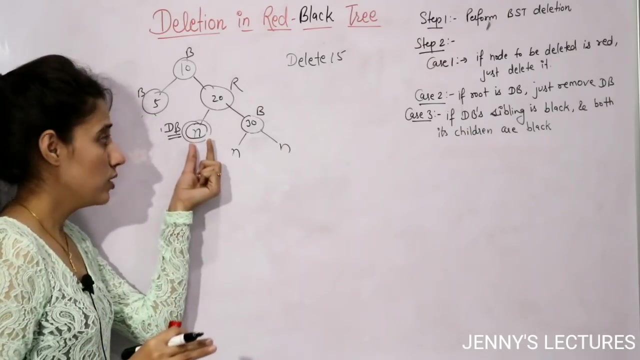 uh, his face becomes, you know, red. so 20 is angry. if someone is cool, then he is black. right now this is double black means this is also a problem. you cannot be so much cool or calm. sometimes you need to be angry, sometimes you need to show your anger, right. so this is a problem. double black situation is also not good. 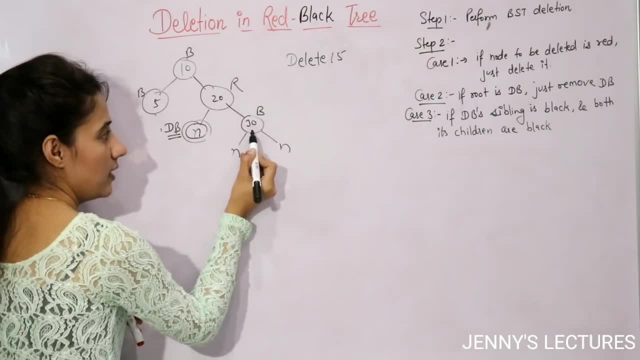 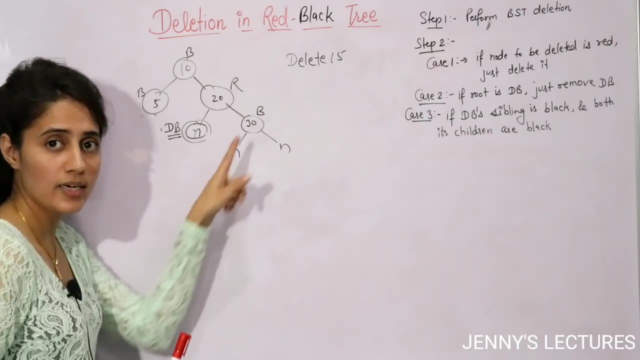 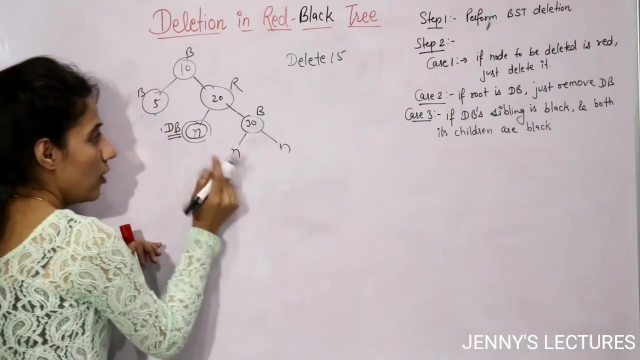 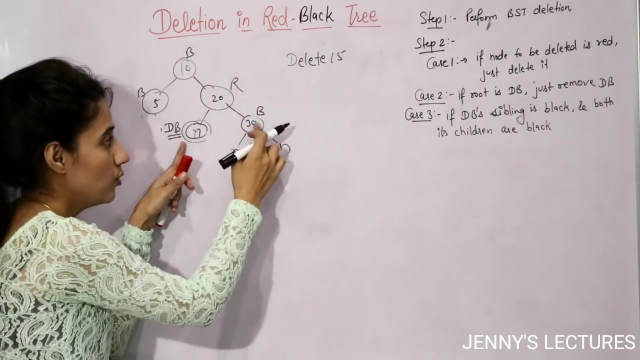 so now it will see. he will see its sibling. it is black, cool, he is cool. so this the sibling doesn't need any black color now because it is already in black. its children is also, so now all the three are black, so he cannot give its extra black to either of these three nodes. 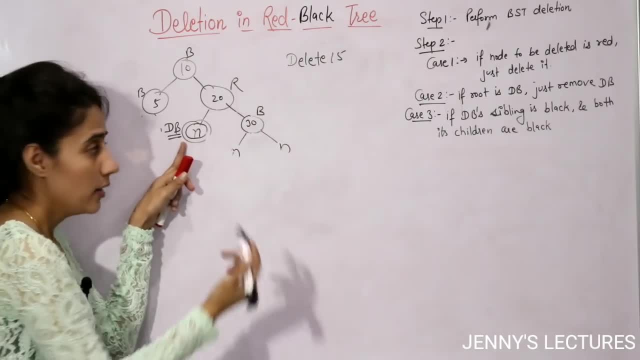 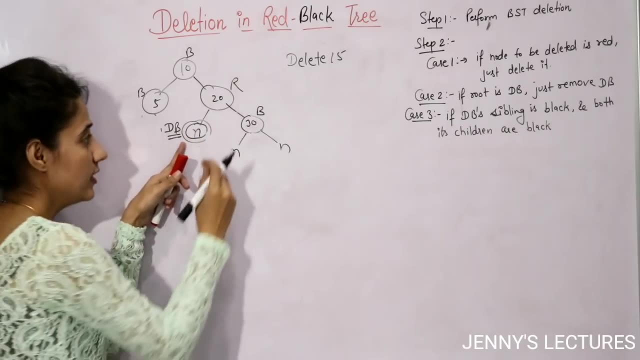 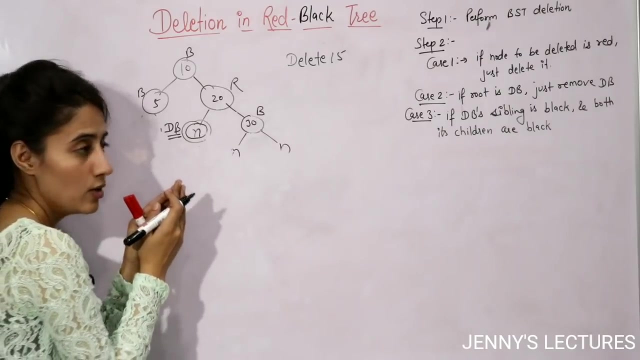 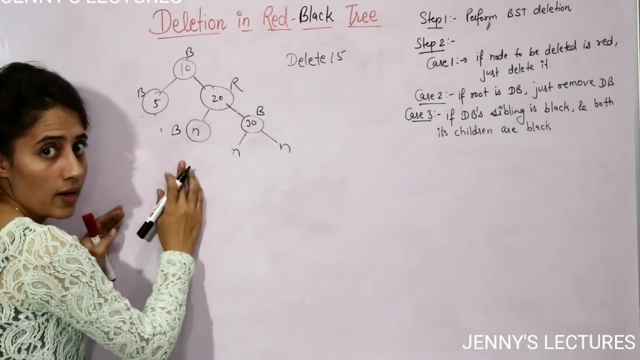 neither to its sibling nor to its children. now what he will do. he will ask to its parent, right, and obviously he will give its extra black, or you can say that its problem to its parent, right. so now here, first of all, remove this DB, so it is simply single black now, and add black to its 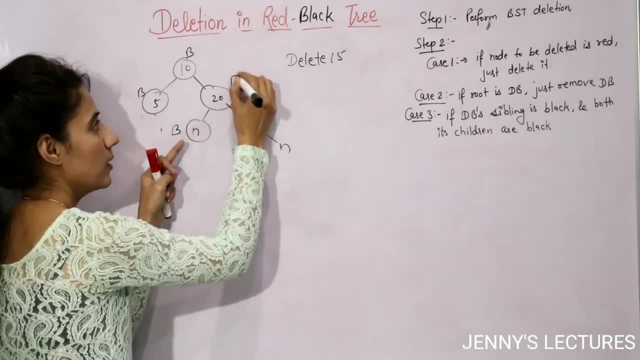 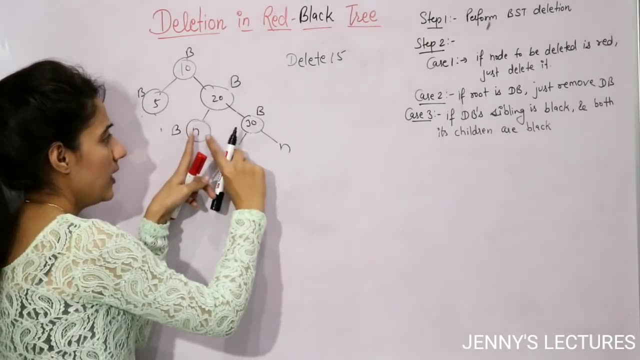 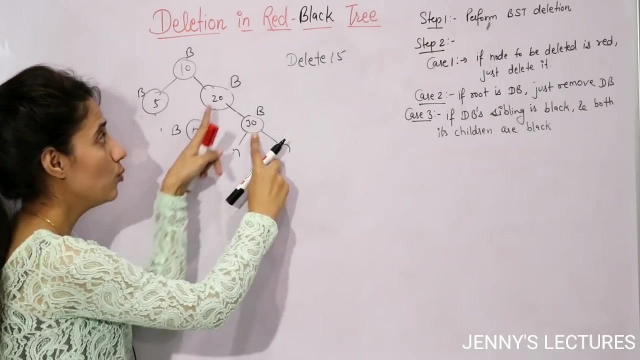 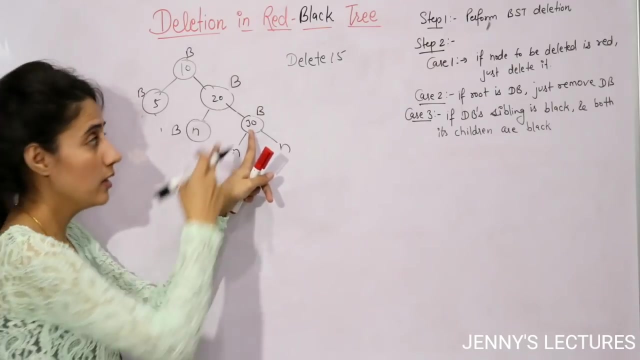 parent. so now parent is red, so parent becomes black. right now what you will do when its sibling come to know that he has given his problem to parent? then what? the sibling becomes angry. right, that why you are giving you, why you are troubling our parent. fine, so now it will. 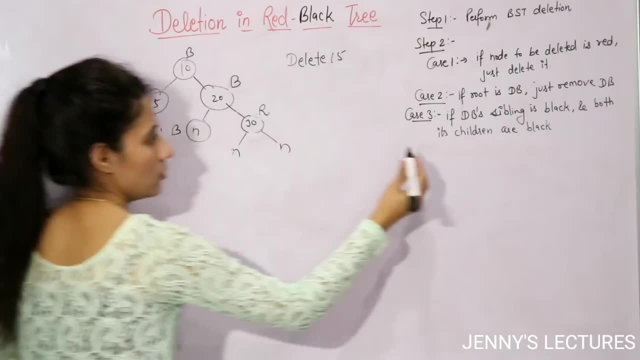 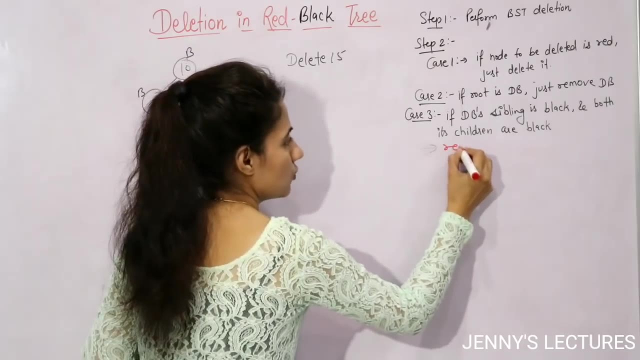 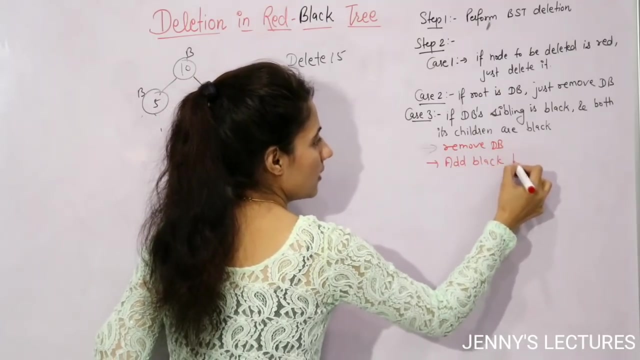 become red. now the steps are what? if this is the situation, then what we have done? simply remove this DB, first of all. and what we have done? then add black to its parent. add black to its parent. and what we have done, then add black to its parent. 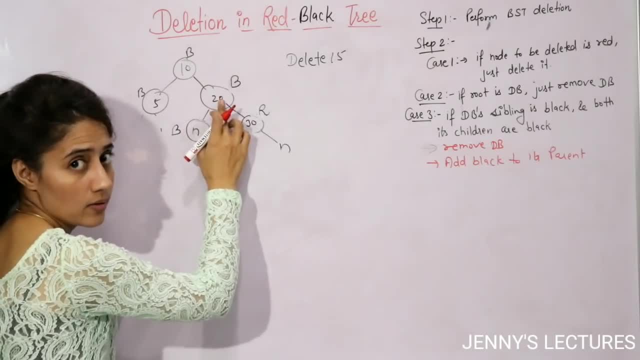 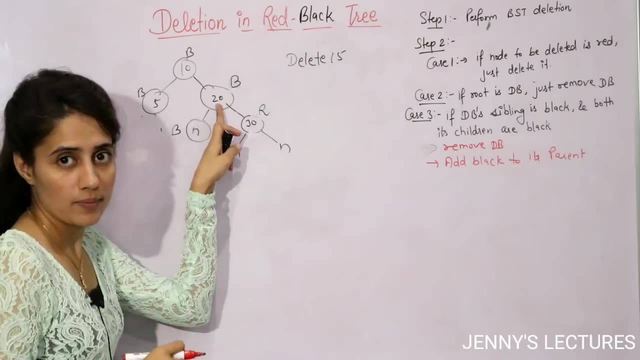 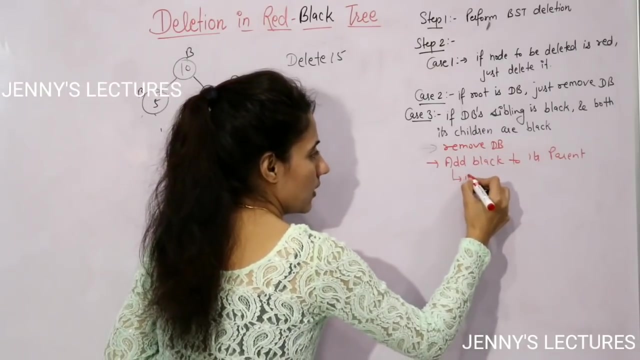 add black to its parent. add black to its parent, black to its. this was double black node to its parent right now. here also two situations can be there. if the parent is already black, then it will become double black, and if the parent is red, then it will become single black. here the parent was red, so here also two situations are there. if 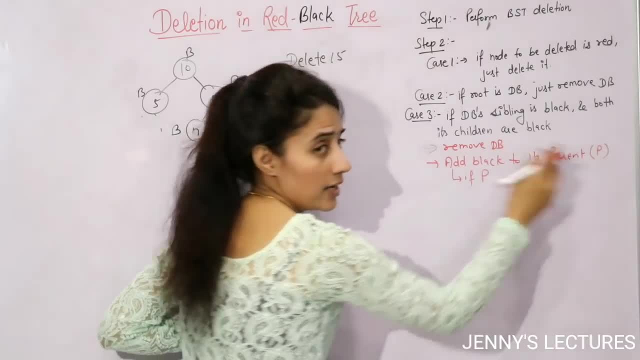 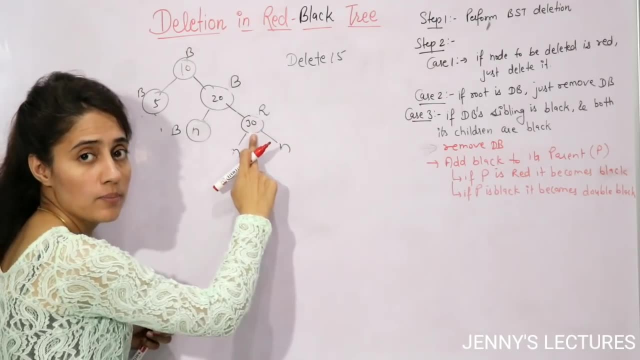 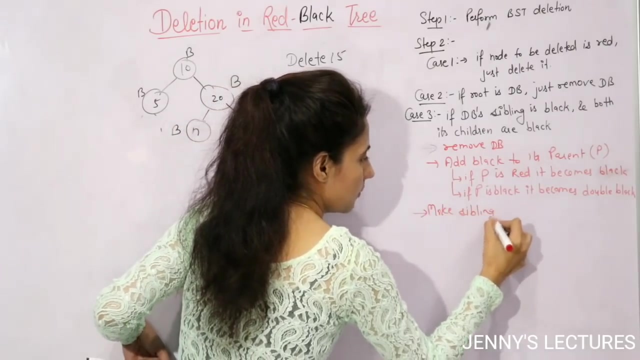 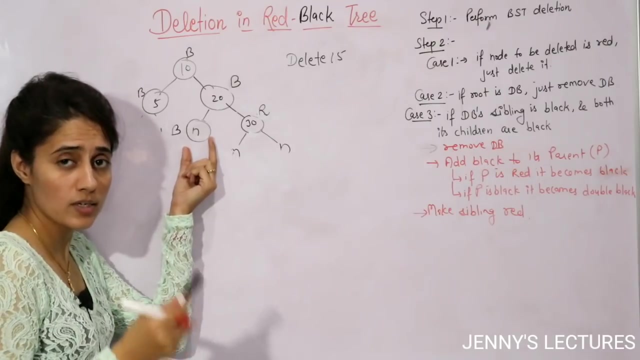 rather than parent. i am writing p. p is red. now next thing, what we have done: the sibling becomes now red. so now next step is: what make sibling red? sibling means sibling of double black node, because double black node is having problem. now we are discussing the cases on this double black. 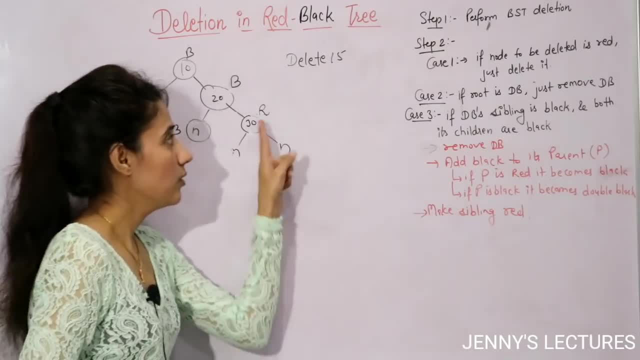 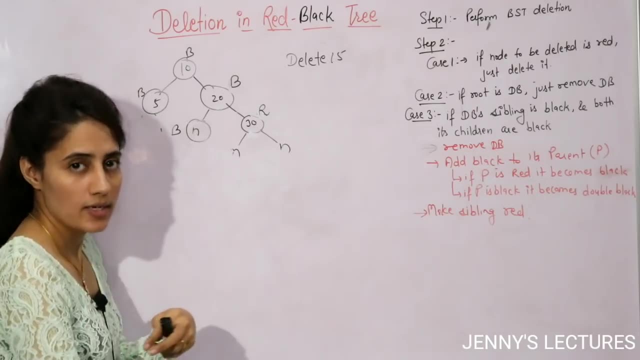 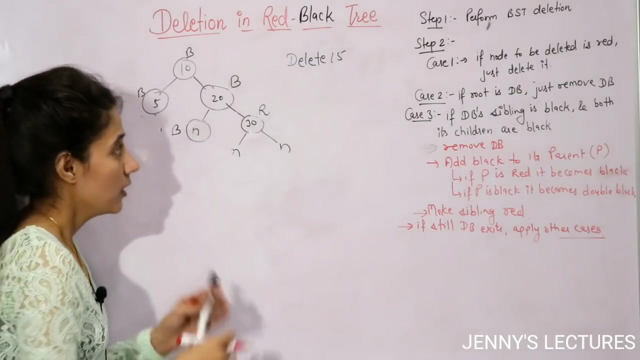 so sibling means double black. sibling becomes now red. right now, if still the problem of double black exist, then we will apply some other cases right so now. and what, what, what, what these other cases, that thing also we will discuss one by one right now. here see, there is no double. 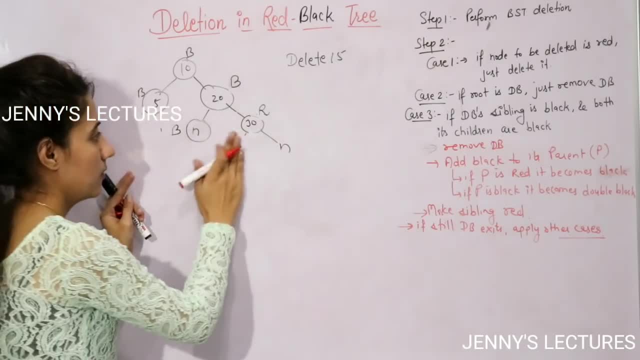 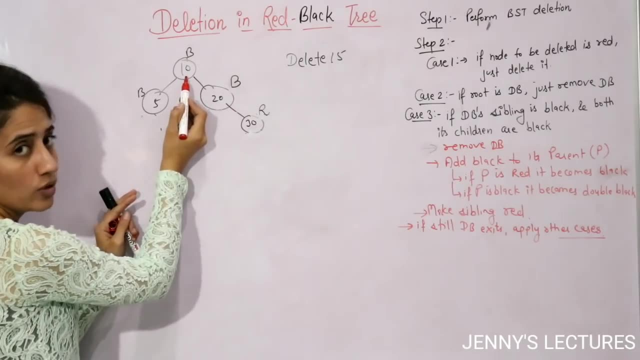 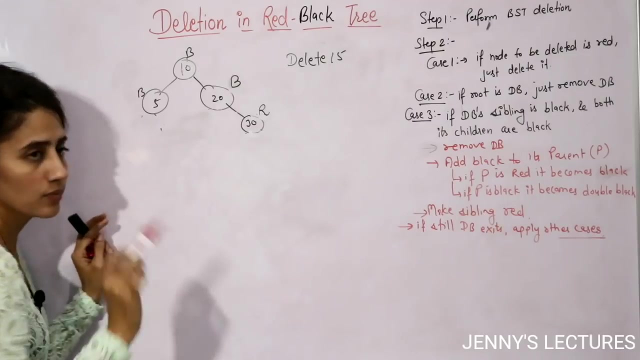 black problem exists now, right, so now it is done, so we can remove this. now. this is also nil, so you can remove it. so now, as you can see, this is a red black. pre root is root is black in this path. one and two blacks, one and two blacks, one and two hair also one and two and one and two. right now, if the 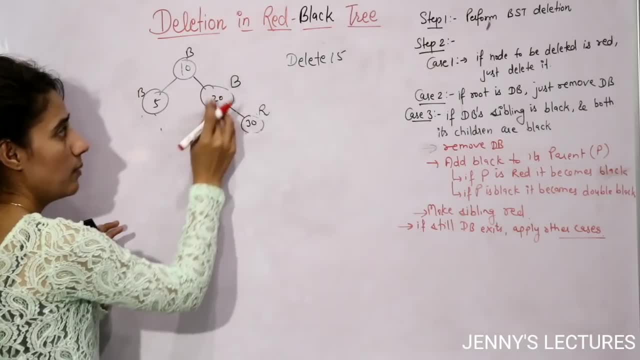 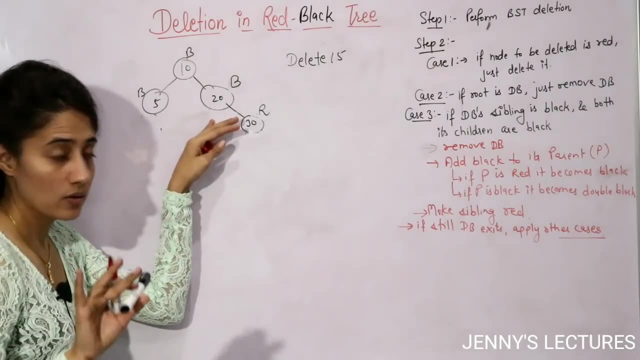 parent was red. sorry, the parent is black, so it would become double black. and here still the double black situation is there. so we will apply some other cases. right, that thing also we will discuss. i hope you got these points. so now here let us discuss this case: that parent is already black. 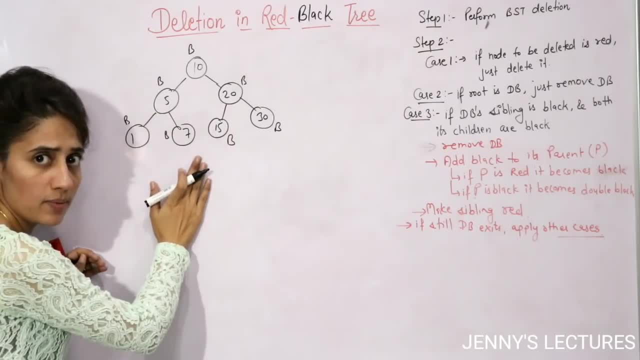 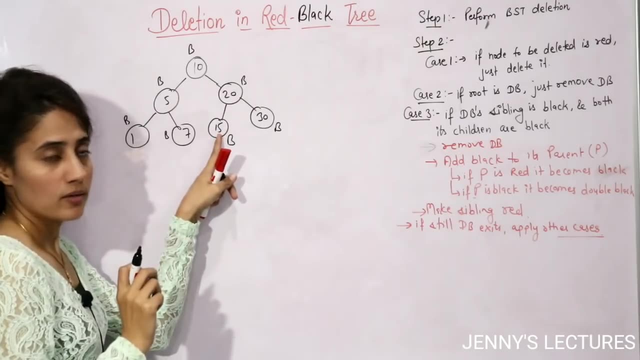 so it will become double black. see, let us take this case. this is a red black tree. perfect binary tree is there and all the nodes are black. so this is a red black tree. now delete here 15. see, 15 is black, so you cannot simply delete. 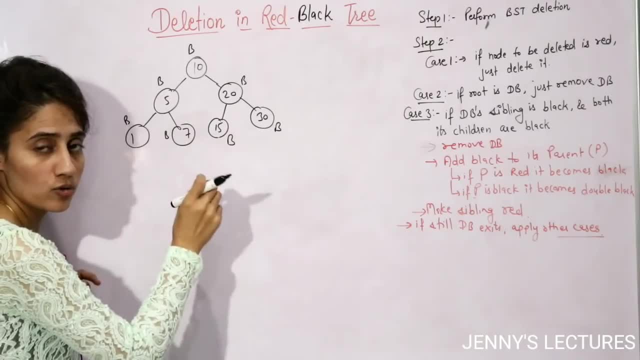 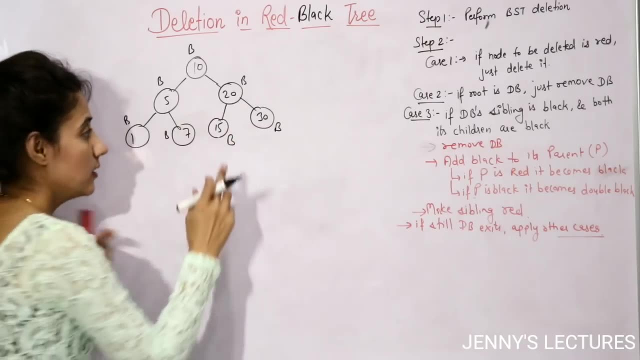 it because it is having two nil children. those are black. so we will replace this 15 with its nil children. so nil is also black and this is already black, so it will become double black. so now, here this is nil and it will become. now you can say, double black. so here the situation is. 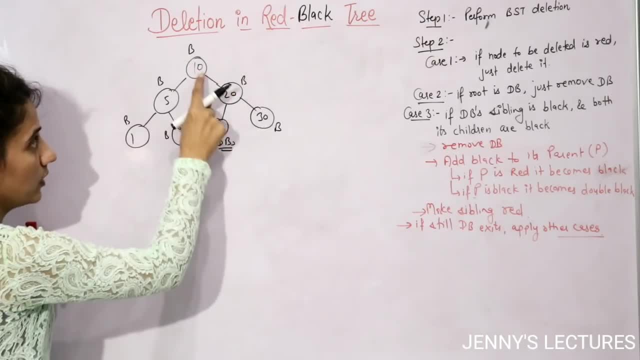 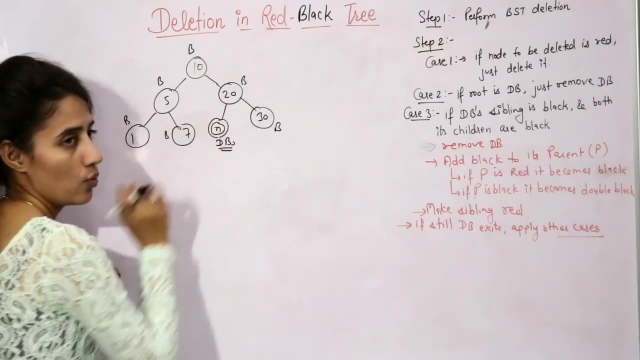 there. the problem is there, because, see, here, in this path we have only one and two black nodes, and all the other paths are having three black nodes. right, because if this is nil, we are not going to count it. so now you need to take care of this thing. 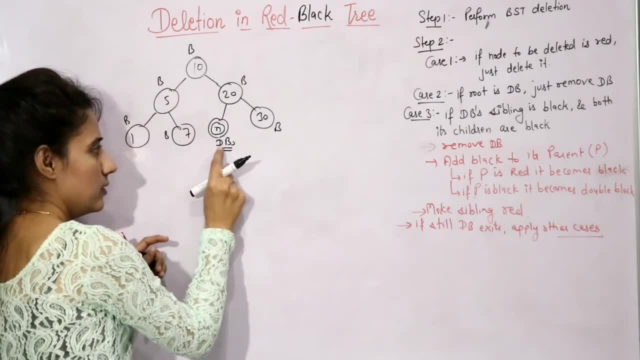 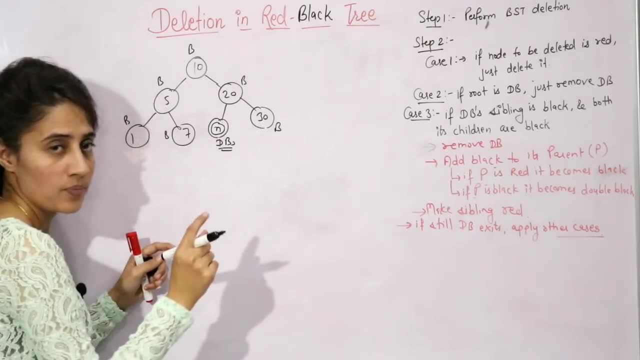 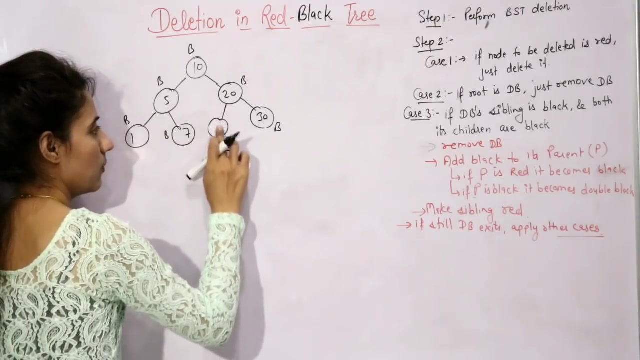 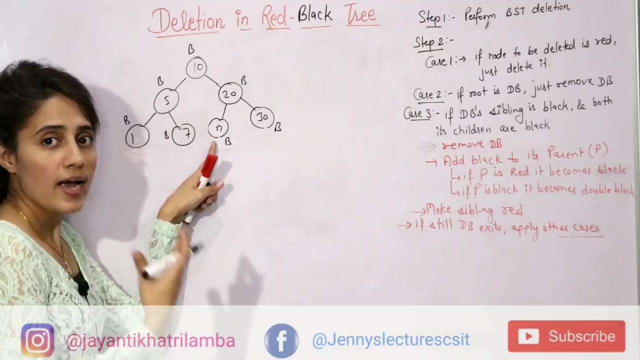 so now apply the cases. check out the: the double black sibling. sibling is black, the two children of sibling is also black. so this is the case right now here. what you will do simple first step is remove db. remove double black. so it is now single black, right, and it is now give its black extra. 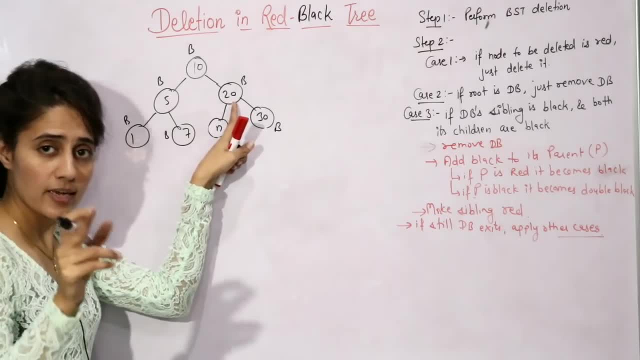 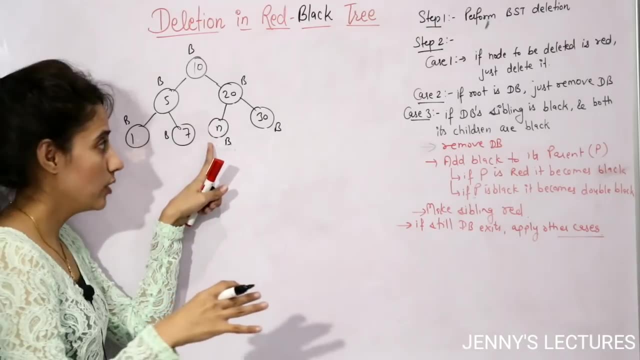 black to its parent right same. you can discuss this case now. so now let us take a look at the case. so we will discuss that. see, this is what black means cool, red means angry. so now this is what double cool. so that is also a problem. he will ask to its sibling, but sibling is. 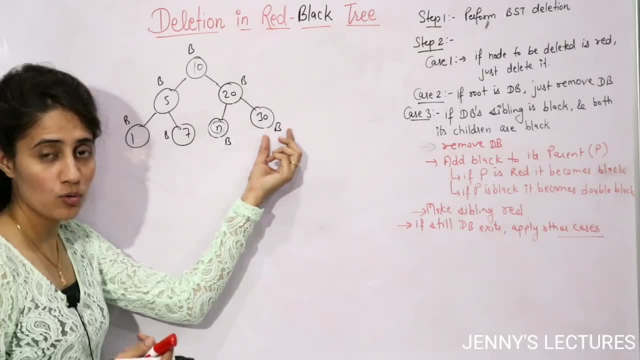 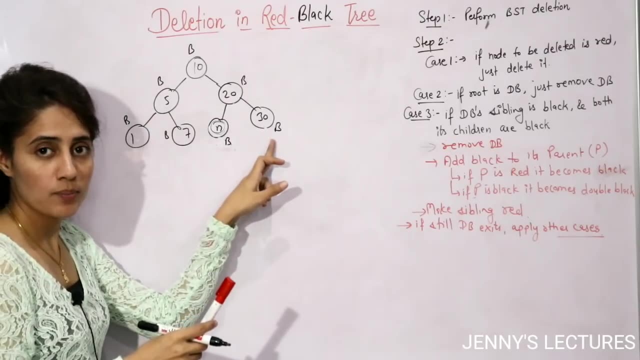 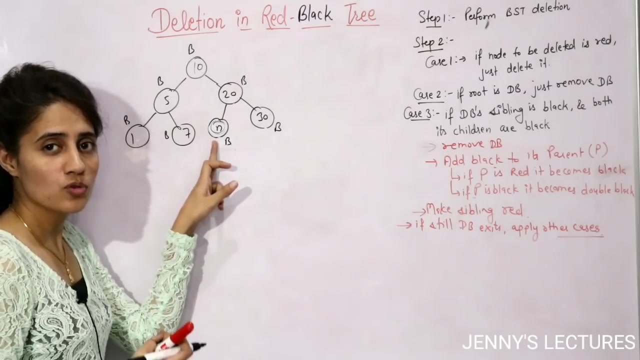 cool, he doesn't know need any black node, or you can say: no more coolness, he needs. children is also black, so they don't need any extra black. so what it will do, it will ask to. its obviously parent right, because if children is in problem, so 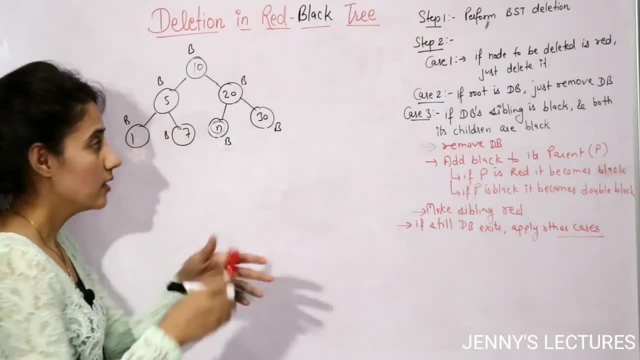 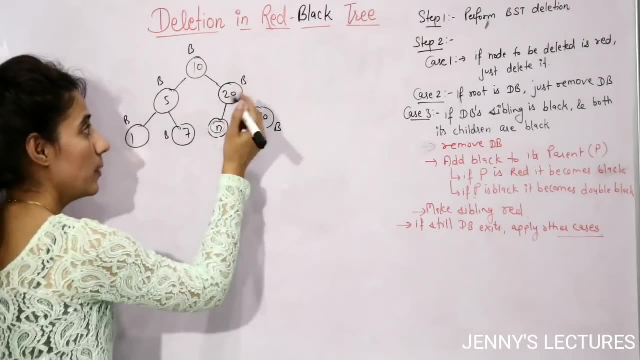 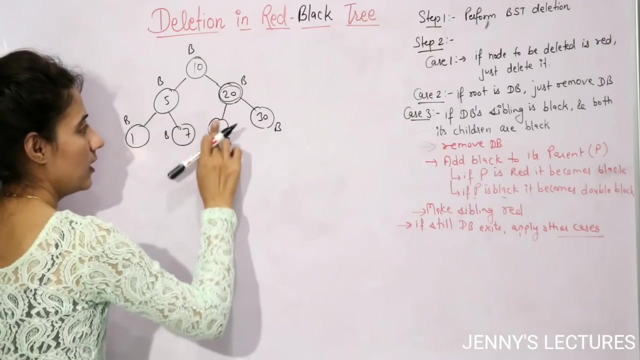 he will go to its, he will go to his parent, right. so now he will go to his parent and give its extra black or give its problem to its parent. so now parent becomes double black. why so? because parent is already black, so it means it become double black and it becomes. 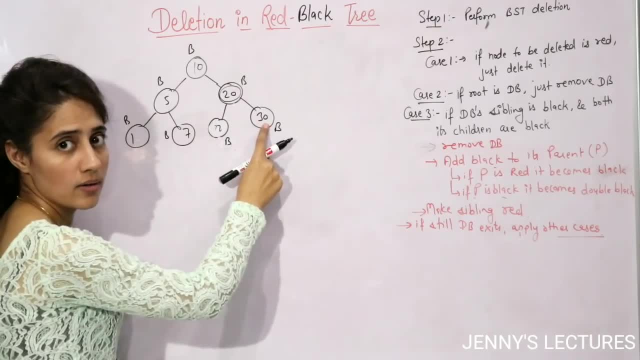 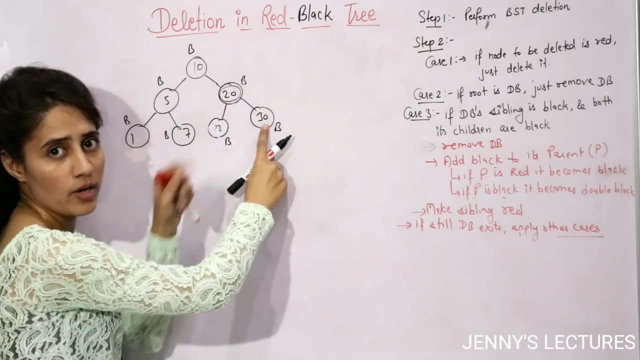 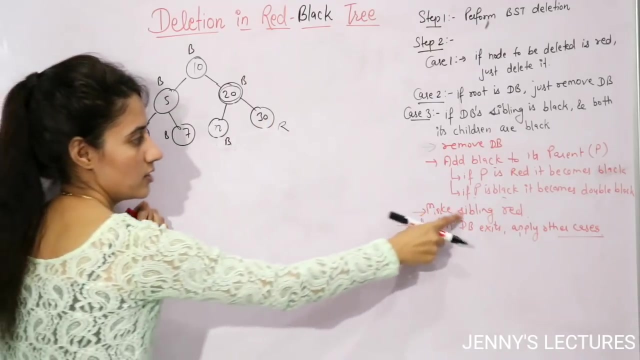 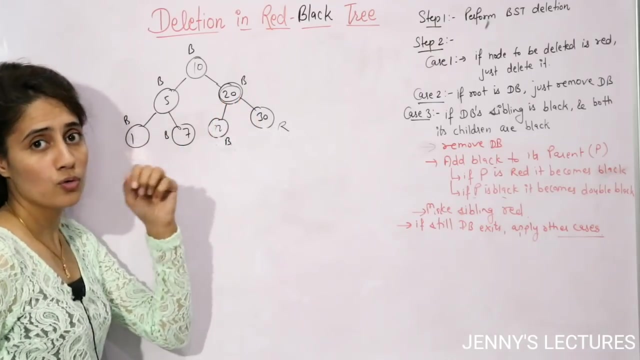 now single black. now sibling becomes red, sibling becomes angry. why so? because he will say why you are giving your own problem to our parent, why you are troubling our parent. so now it becomes red, sibling becomes angry, makes sibling. read now here still, DB exist in this case, right, so you need to follow some other case now. 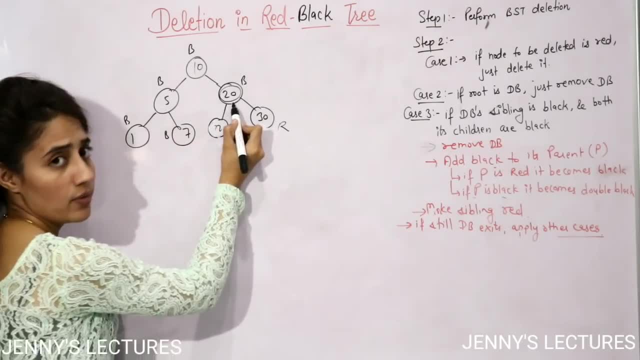 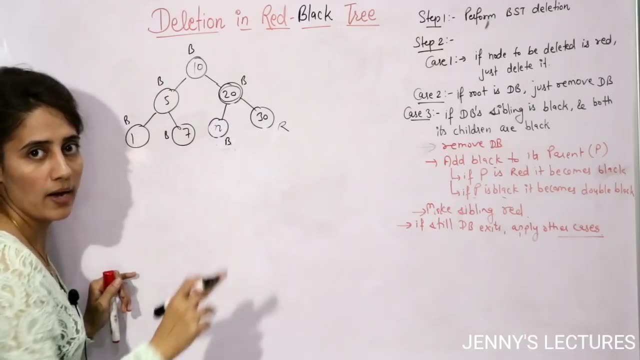 which case you need to apply here. see, this is the node which is having problem. so he'll check at siblings. siblings is black children. both children are black. so Dante Cl round ofnez called it he. they don't need any Wilhelm guilty of black. the white team should buy black faces inside. so this kid, don't buy black. 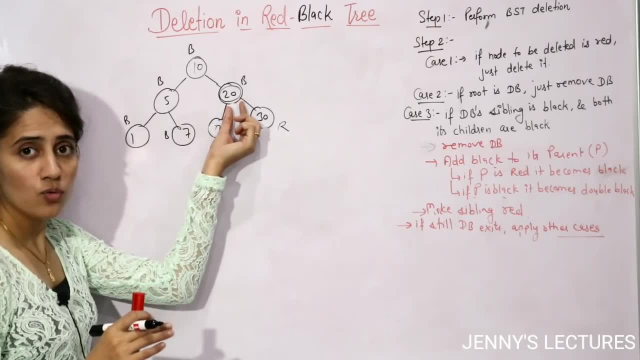 plates and they must get the baby's home name. and then the second child come, black, called clockゃ paul. okay, good question, you have to be sure, but whenever you have something more black already cool. so now what he'll do? he'll ask to its parents means he will give its problem to. 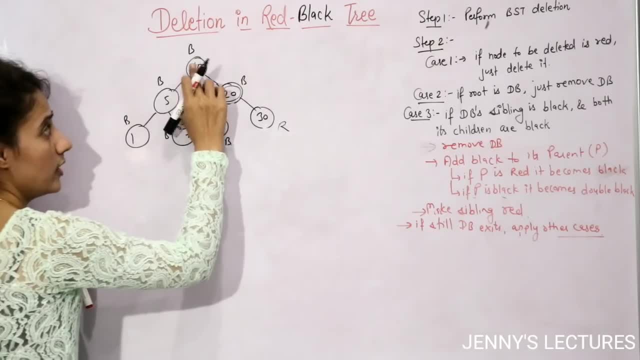 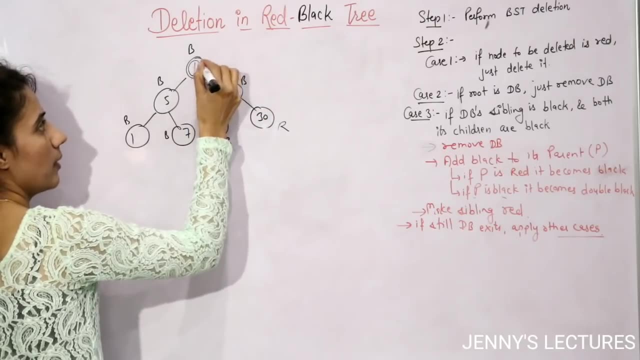 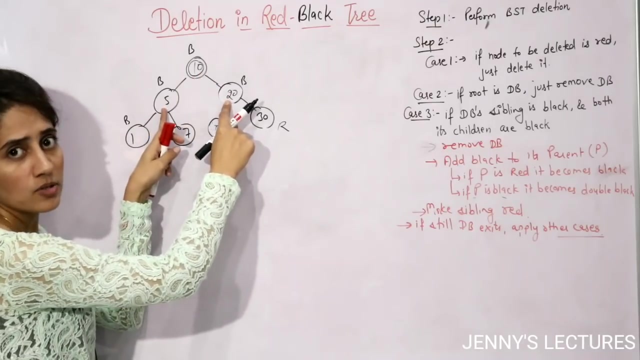 parent right. so parent is already black. so now you can say: first of all, remove this db. it has become now single black and parent becomes now double black because parent is already black now. after doing this, now sibling becomes angry. why so? because he'll say why you are giving your 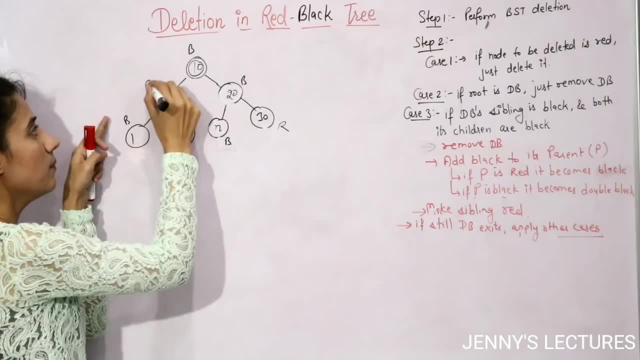 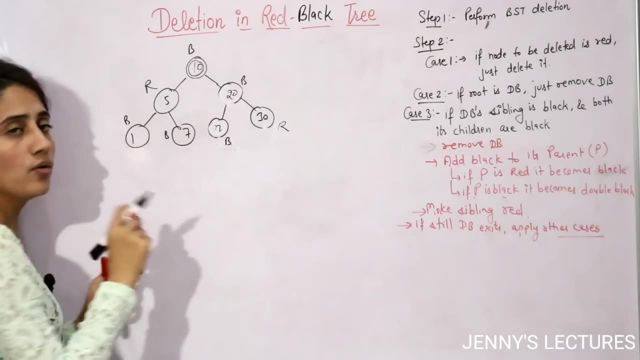 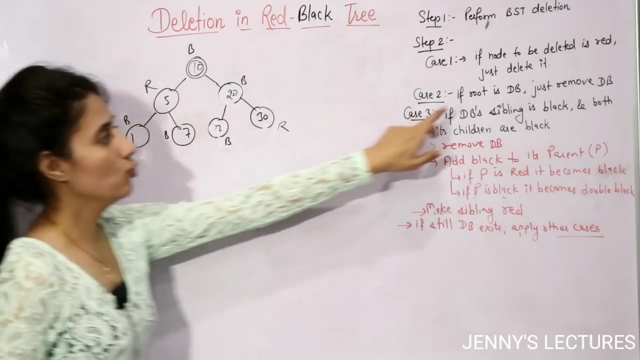 own problem to our parent right. so now it will become red. from black to red. now the situation. see now here, still in our problem, we have double black situation. now which case is there? identify the cases. now see double black is what root. root is double black. this is root, so simply remove. 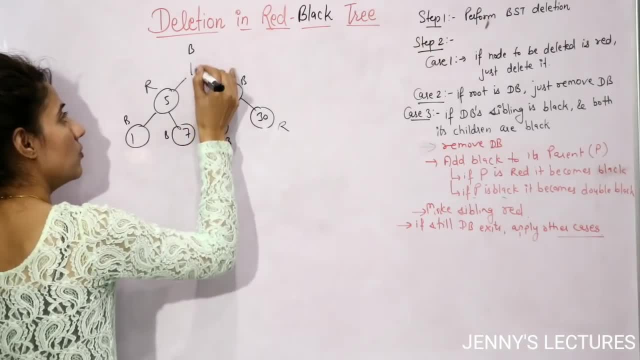 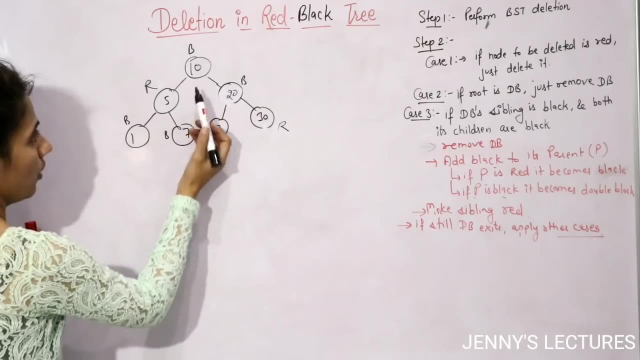 double black. no need to do anything. so simply remove it and it will become single black. right, and that's it. so you can see, this is what a red black tree. you can count the black nodes 1 and 2, 1 and 2, here also 1 and 2, and here also 1. 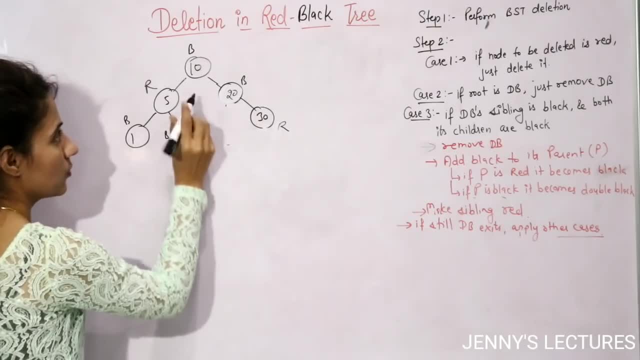 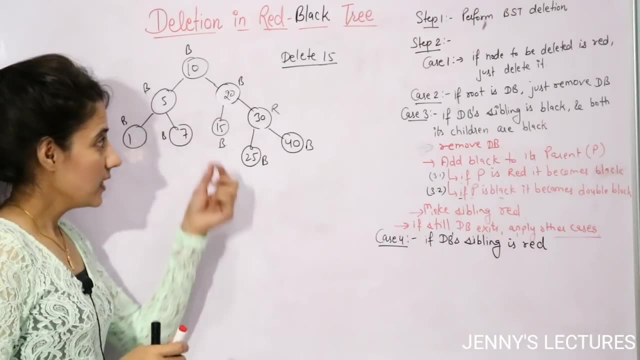 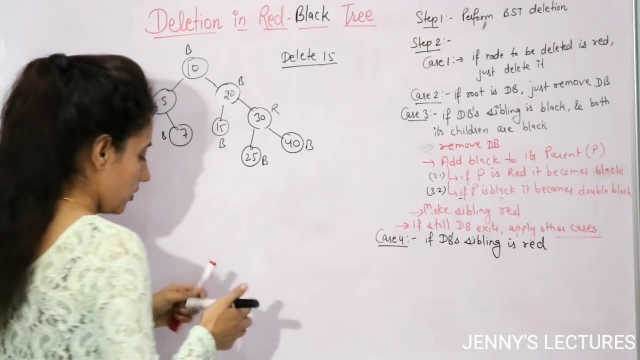 and 2, because this is nil, so we will simply delete it. so here also, 1 and 2 right now. check out the next case. so now let us take this case, and here this is a red black tree, and from here i want to delete this 15 right now. search where is 15. here you got 15, but you cannot simply delete it, because 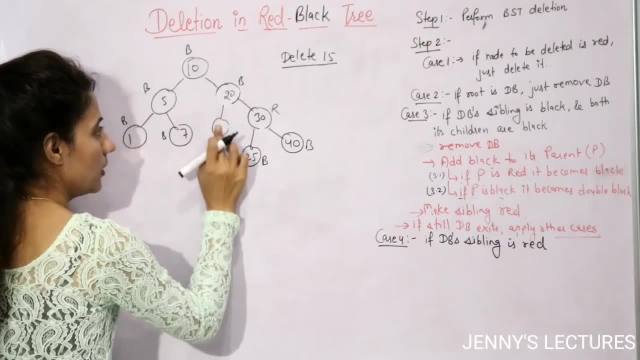 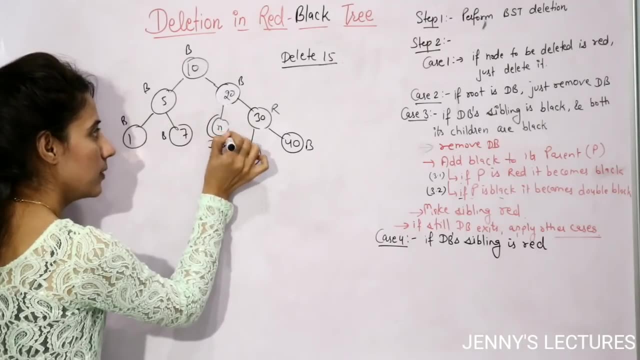 this is black. so now, after deleting this 15, it would become- because obviously it is having nil children. we will replace this with this nil and it will become now double black, because it is already black and its children is also black, with which you are going to replace it, so it will double. 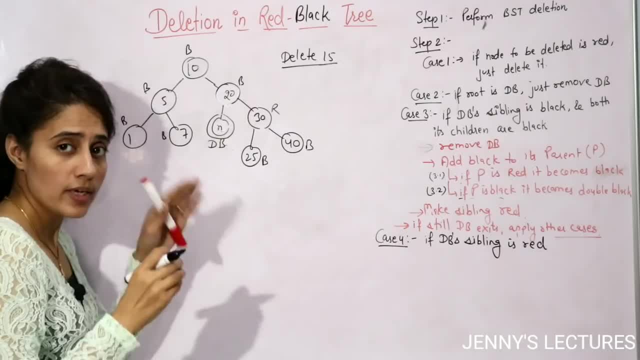 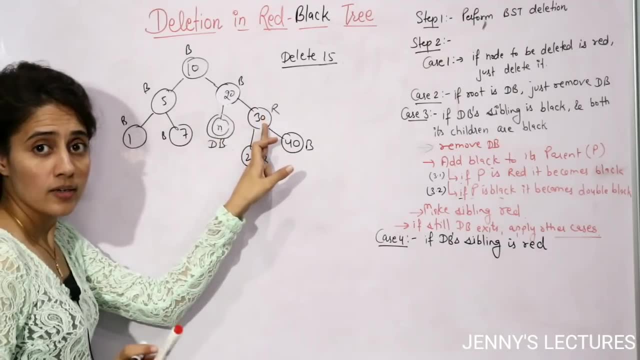 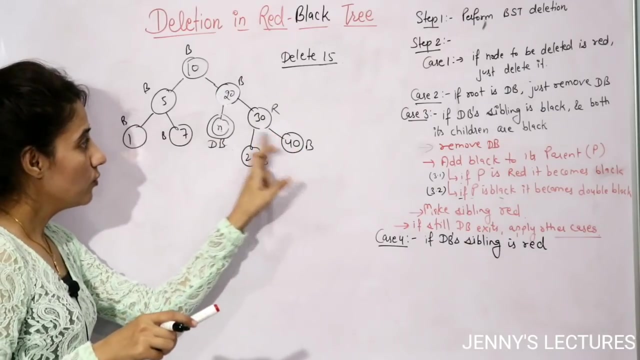 black now. now find out which case you need to apply. to find out the cases, simply check the sibling of double black right. check the sibling of double black after that. after that, you will check the this children of the sibling right, the children which is away from double black, and after that you will check this children. 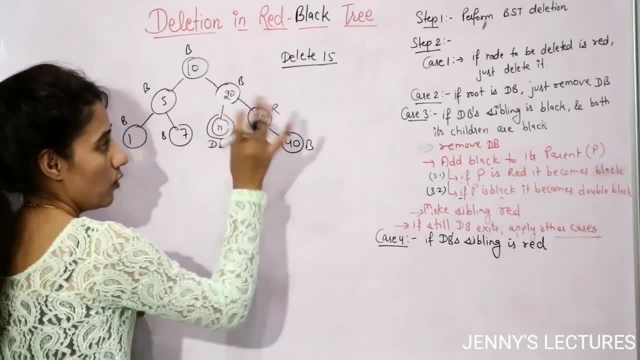 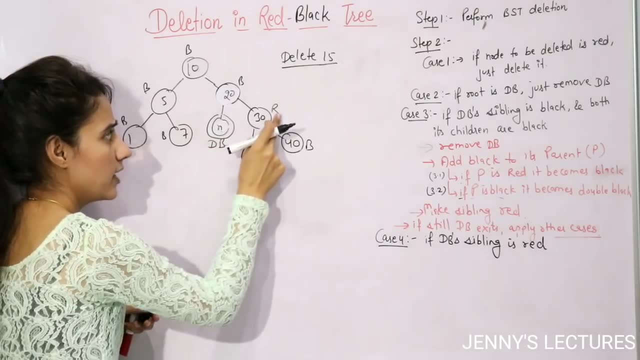 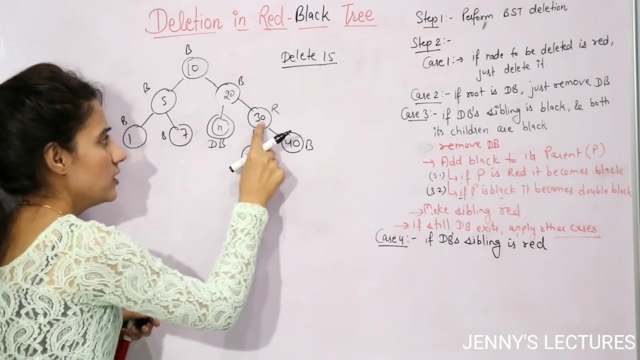 these cases also we will discuss now. we have already discussed this case when sibling and its children were black. now, second case is now here. the sibling of double black is red. so this case is there right here. we have discussed two sub cases right now. this is red. now what you will do. 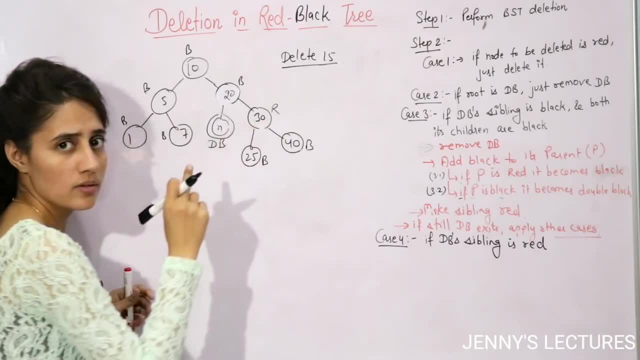 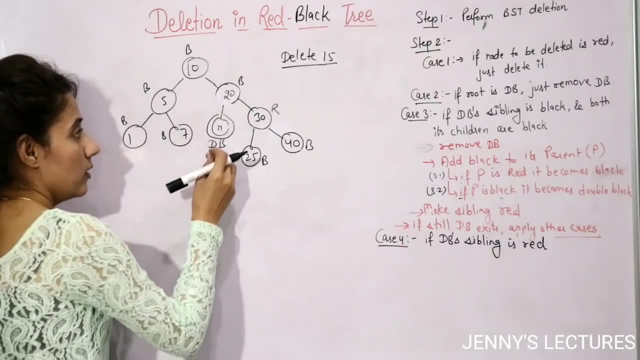 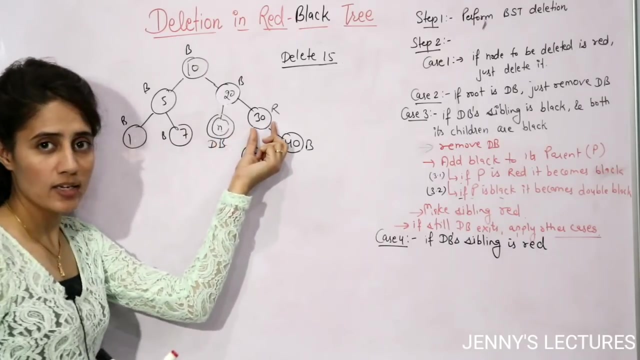 see it means the sibling of double black is angry right because there are friends right here, so you can easily see the life- that have group brother and that your sibling have greenrendo ability right now you know that your sibling is angry right. or, as you can see in the second case, if you have two siblings who are very 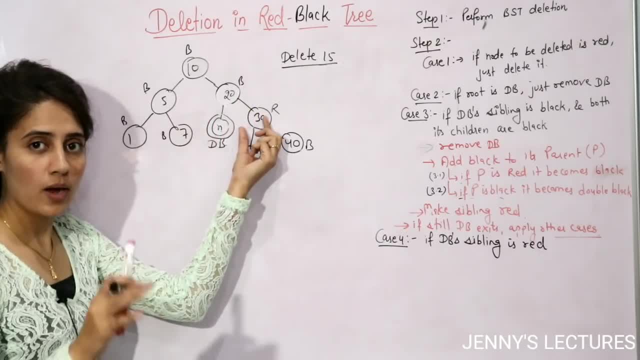 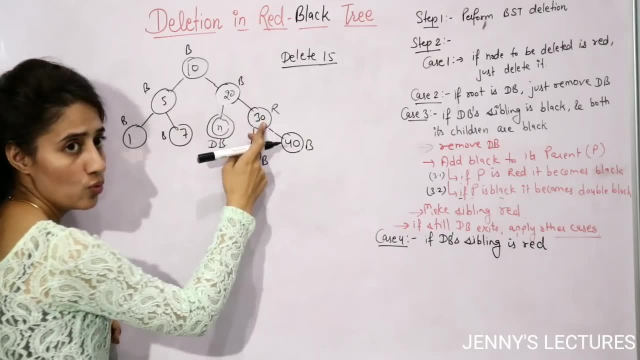 angry and the husband is going to go to any step. you understand now. boring, right? if the house is full of siblings. right, as you go. he is angry, right, depends on how he wants to solve the problem, can't he? I can to nationally go to hisasted sibling friends, right, because 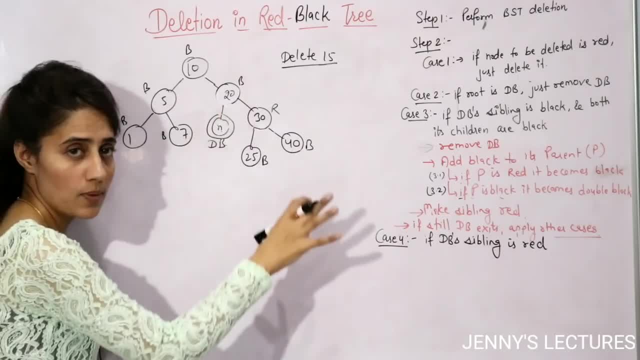 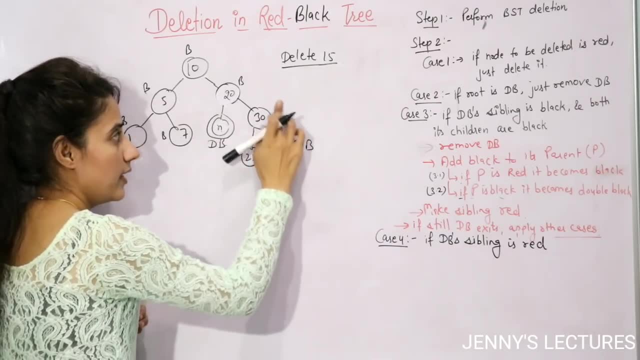 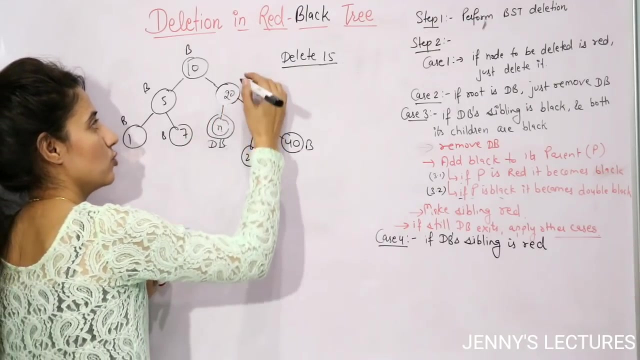 he set the school different from two and ask: our siblings will calm down, low down. his brother, right, or you can say his sibling now. when the parent will go and tell him to calm down, then it will become black, right, but in that process the parent will become angry. so parent 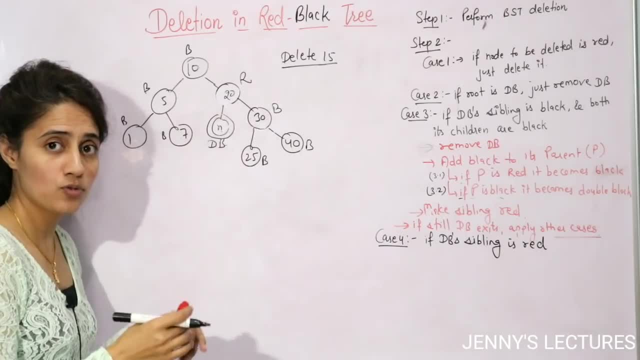 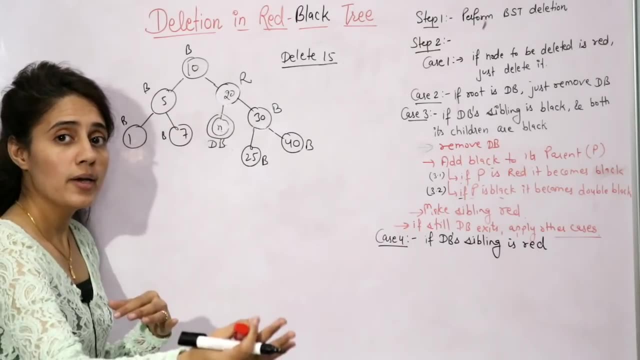 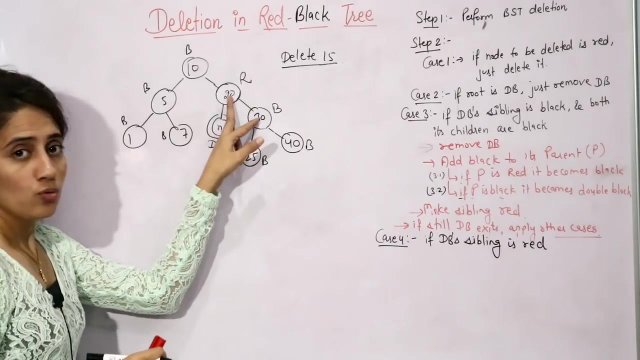 will become red, because generally it happens when you are angry and your parent comes to calm you down, to cool you down, then they will become angry and then after that you will be like silent. so now we are going to swap the colors. now the, the sibling becomes red to black, but parents become 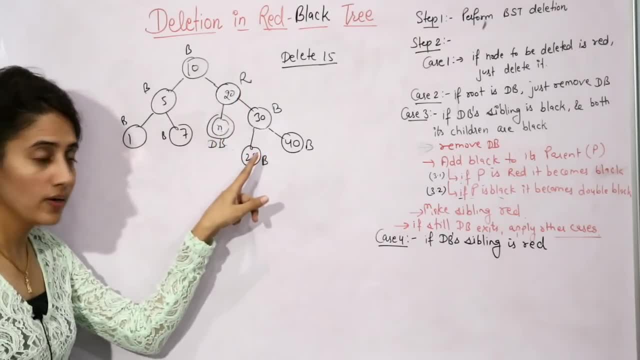 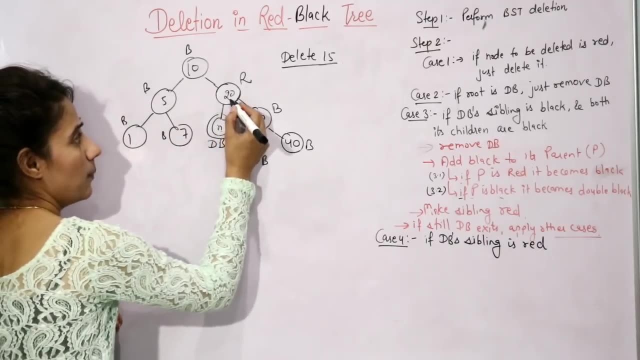 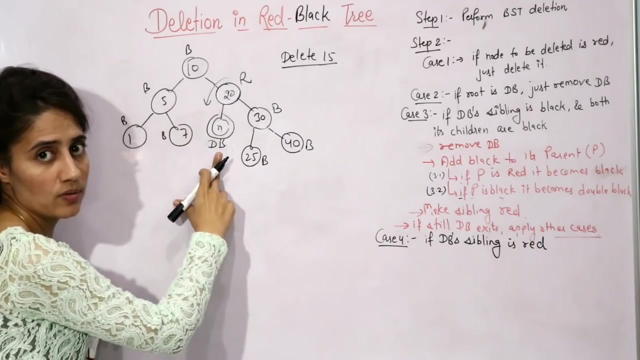 from black to red. first step is this one, right, but still the problems. is there db problem? is there double black problem? is there now? second step is what the parent will rotate in the double black node direction right. second step is this one. so now, after rotation, the parent will rotate towards: 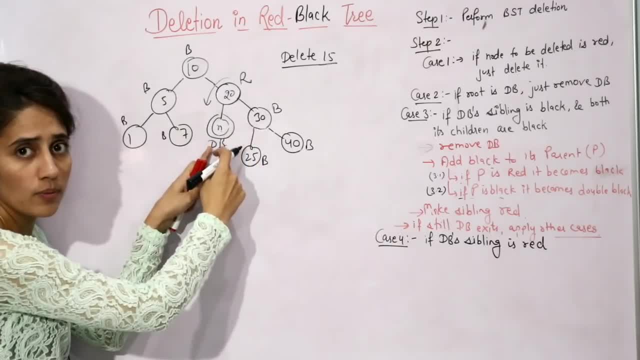 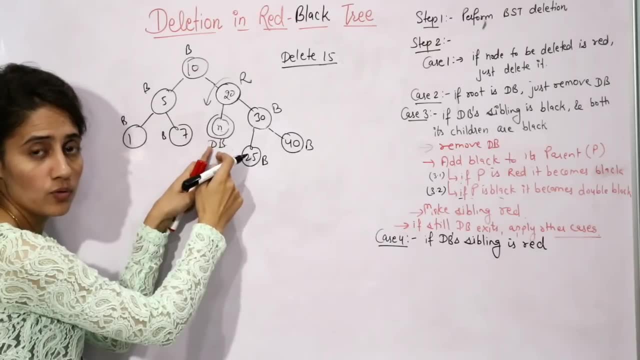 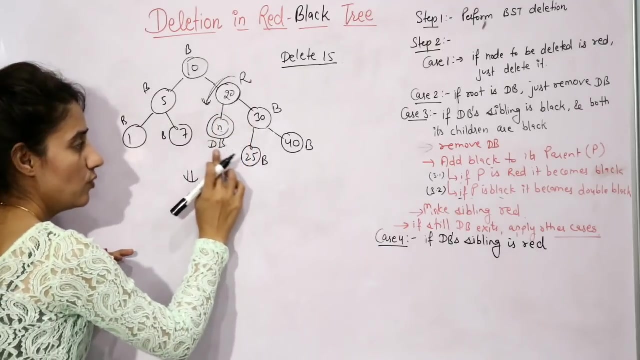 this direction because this children of parent is having problem, this child is having problem, so parent will go, will always rotate towards the, the child who is having problem right. so now this rotation, you can say the left rotation or you can say in the direction of db, the parent. 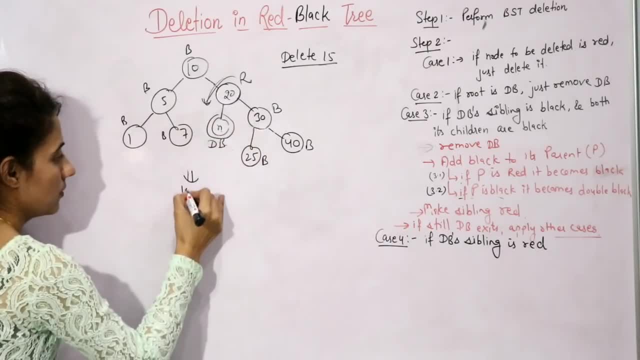 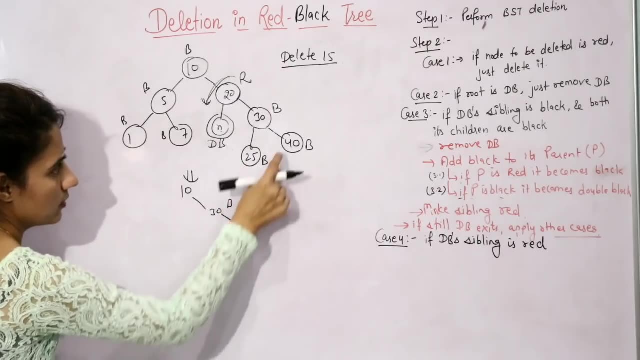 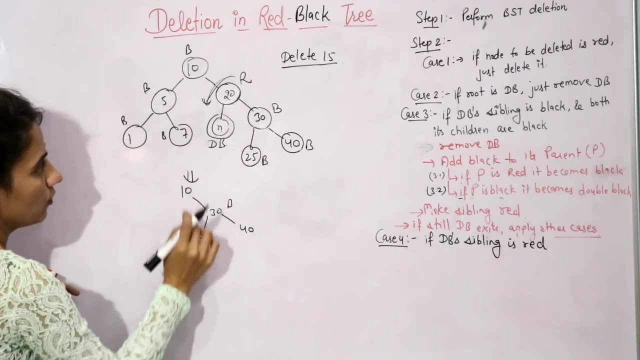 will rotate now after rotation. the tree would become: after rotation, 20 would be down, 30 would go up, 30 is black, 30 is having right child, this 40 and now 30 is up, 20 is down. so 20 is to the left of. 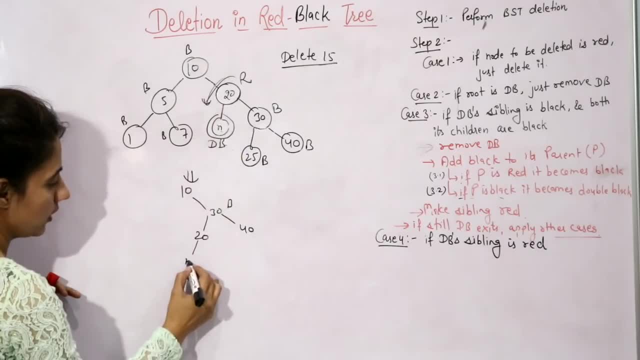 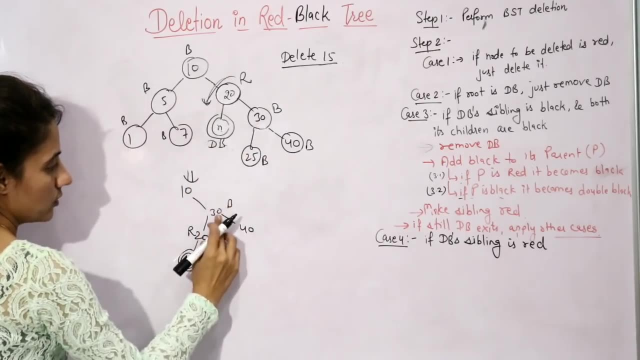 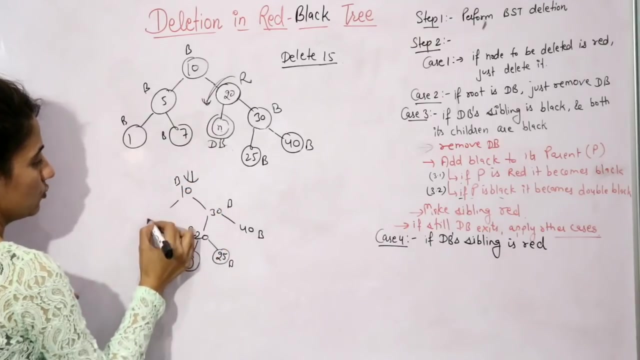 this one. and here we have to the left of 20, we have null. that is double black. 20 is what red now where 25 will go. 25 is to the left of 30 and to the right of 20. right, this is black, this is black and this is black. and this would be same, this side would be same, right now still. 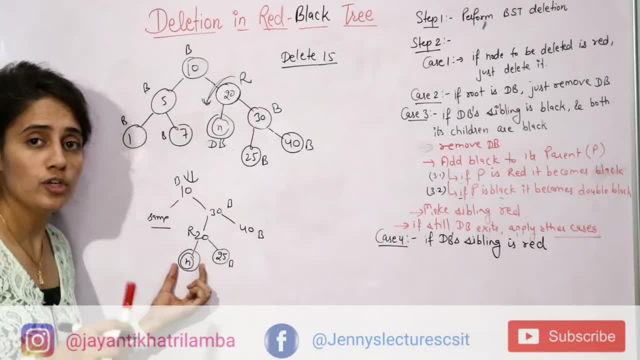 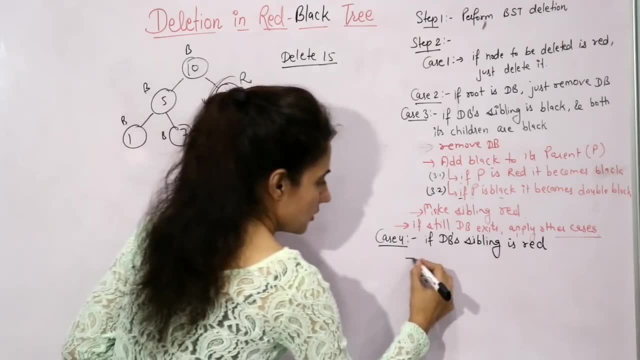 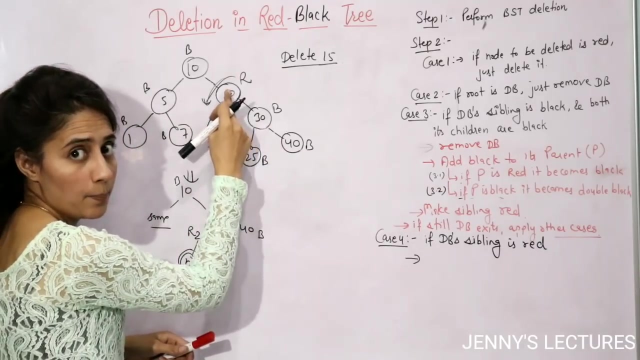 after rotation, still we have double black problem. so now you need to again check which case you need to apply. right so now, this case. in this case, steps would be what? first of all, what we have done? we have swapped color of its sibling and parent right. so now, here you can write. 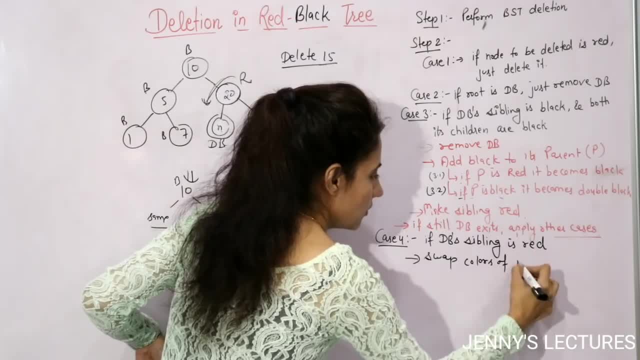 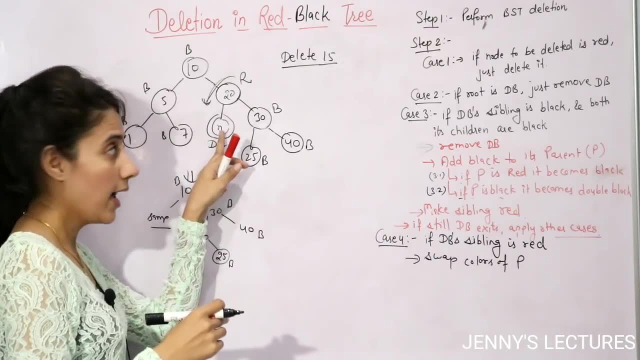 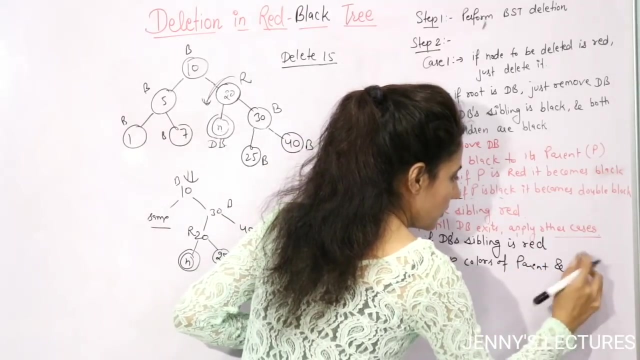 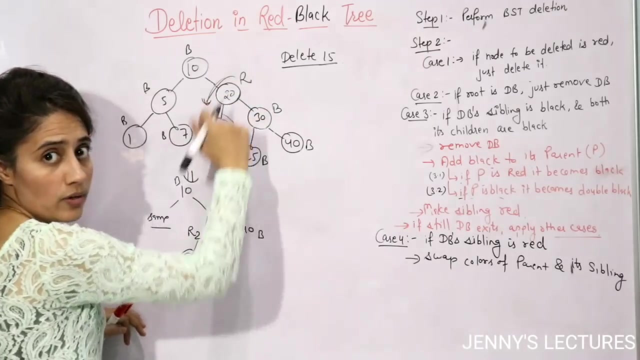 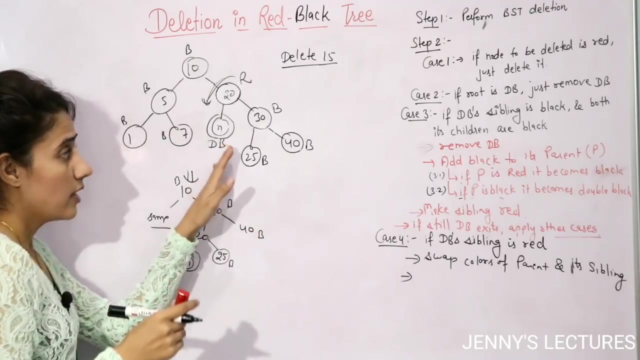 swap colors of parent. or you can say: double black parent of double black right and its sibling properly. you can write this thing so: parent and its sibling right. after swapping the colors, we have done rotations, rotations in this direction, in DB direction, right. see, this case is having its mirror image if DB is. 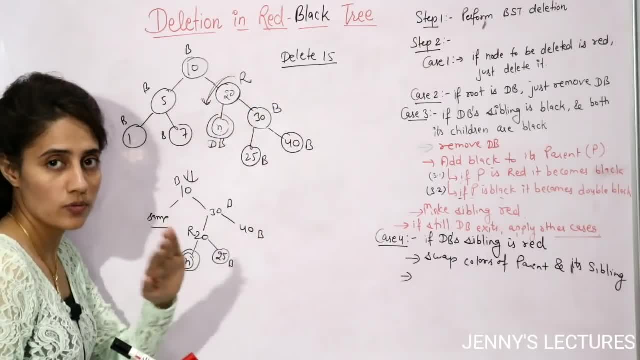 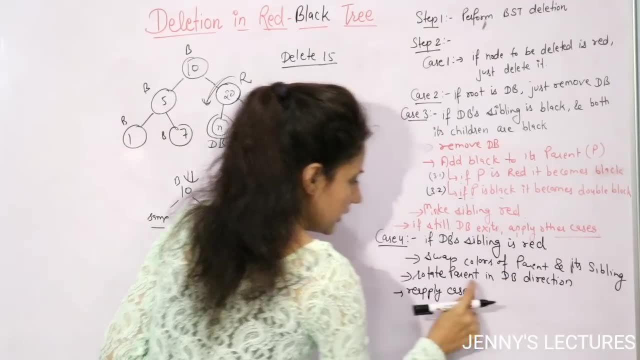 in this direction. in that case this will rotate in this direction. that thing also we will discuss, right, that is why I am saying that: rotate the parent towards DB direction. see here: parent, parent of- you can write down properly: parent of double black node in double black node. 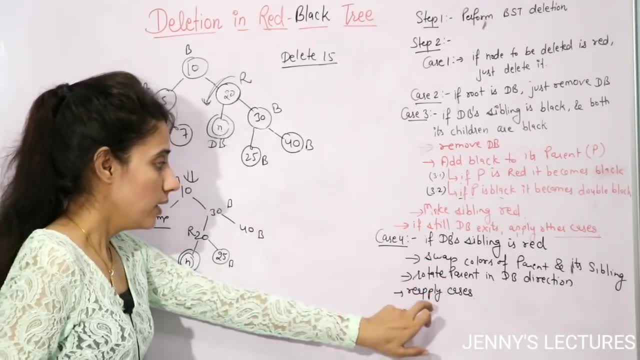 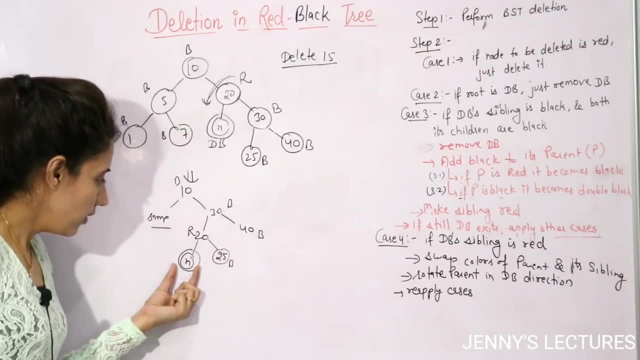 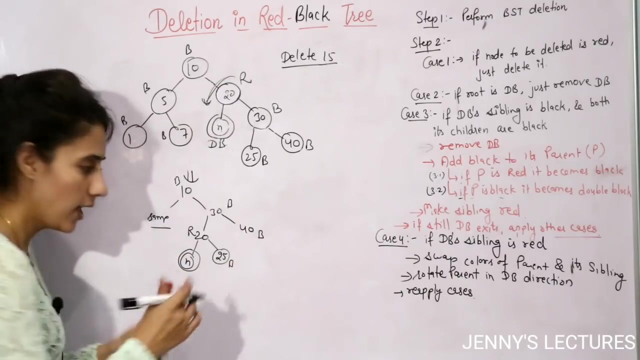 direction. right, I'm writing it in shortcut. and again, we apply cases right now- this is the scenario here- which case you need to apply, check out. still, we have double black situation. now check out the to find out which case you need to apply. check out the sibling of double black. sibling is black. now check out the. 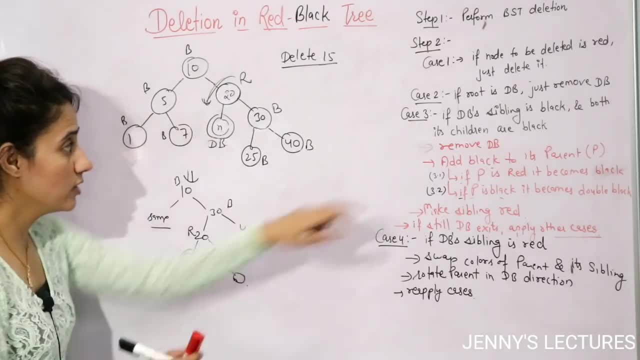 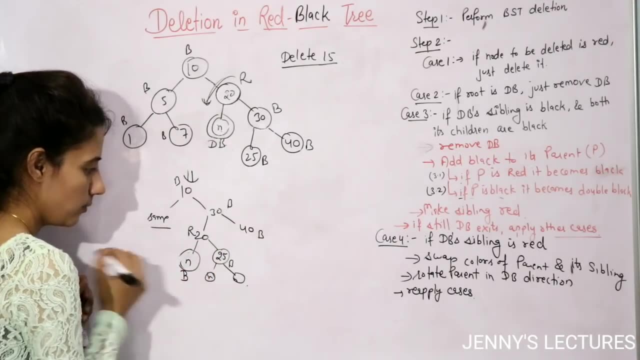 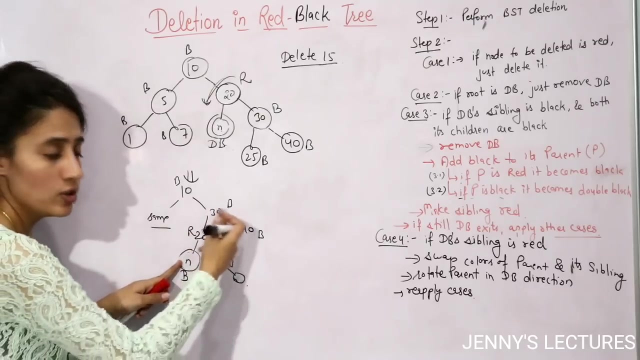 children. children is also nil, and nil, that is black and black. so this case you need to apply now right? what is this case? simply remove DB here we have n means one black on the parent and practically that means that parent is only right and add black to its parent, so he will give its problem to its parent. parent is red, so it. 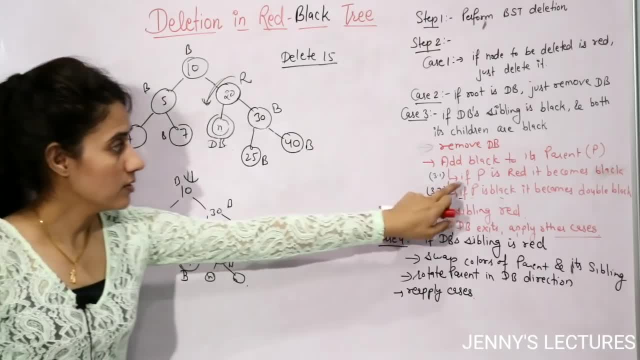 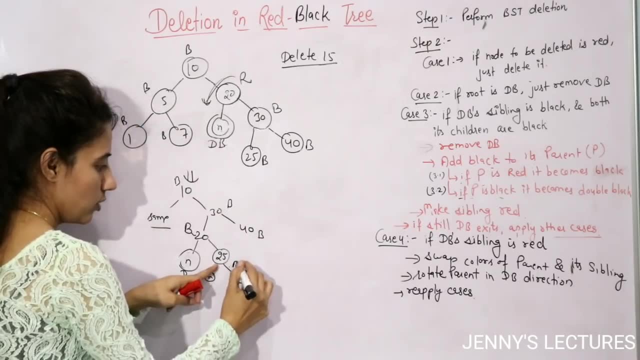 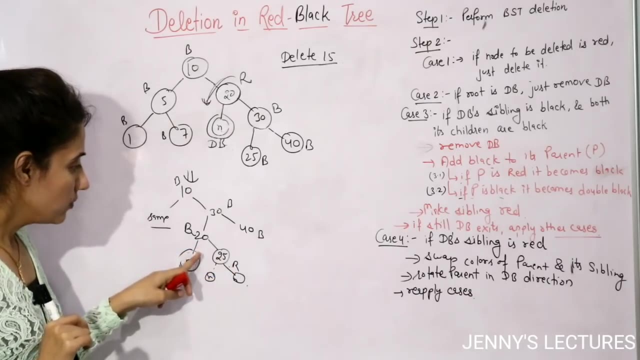 becomes black. right, this is the case. parent is red, it becomes black, and after that sibling make sibling red. so now sibling becomes angry. that why you are giving your problem to a parent. so sibling becomes angry now. now, if still db exists. but in this case there is no db problem exists now this: 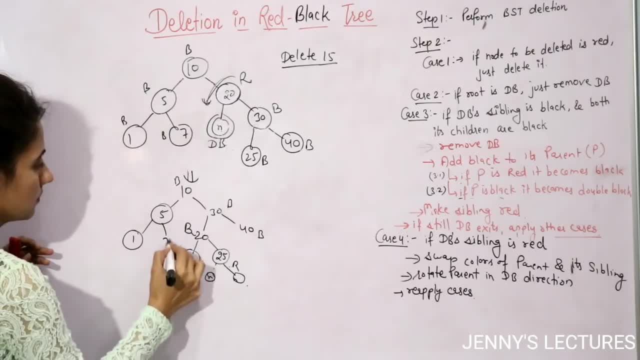 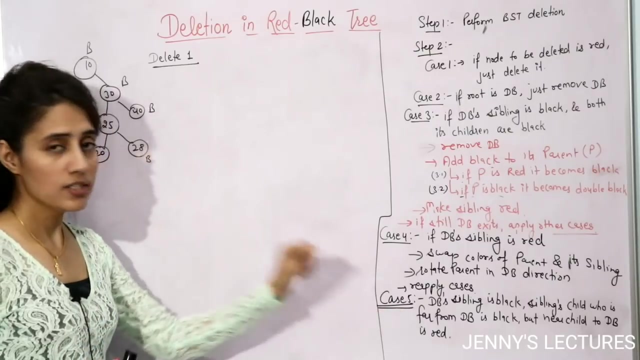 is the final tree after deleting this 15, and, as you can say, this is now a red black tree. from here, this is null, so you can delete it now. what can be the next case? so now we will discuss the case 5. let us take this example: right, this is a red black tree and from here, i want to delete. 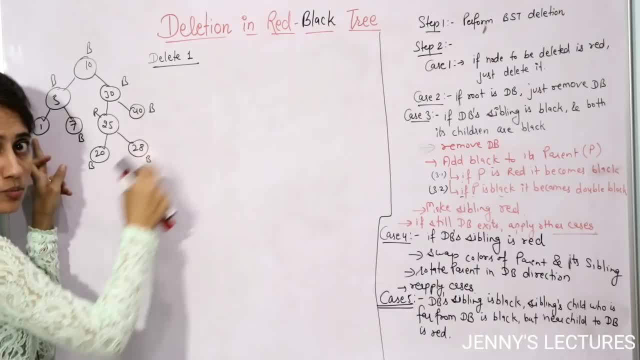 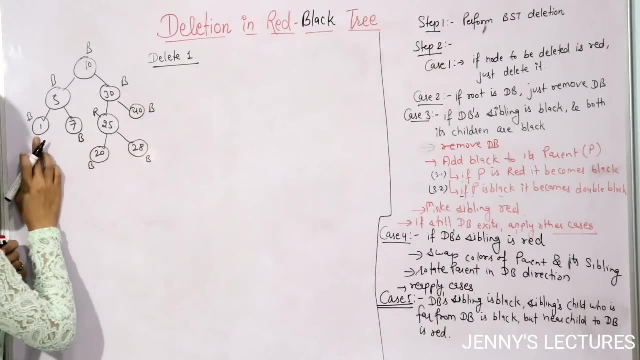 this tree from here. i want to delete this tree from here. i want to delete this tree from here. this one in one example i'm. i want to discuss more than this one case, two or three cases. i'll discuss now. see if you delete this one right. first of all, search where is one. this is black, so we 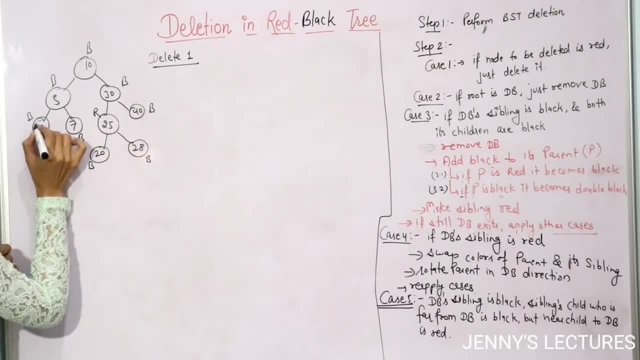 will replace it with its null null node and it will become double black. now, right, so here we have the problem. now find out which case you need to apply to find out this thing. just check the sibling of double black. sibling is what black. now children of the sibling say: this is also black. 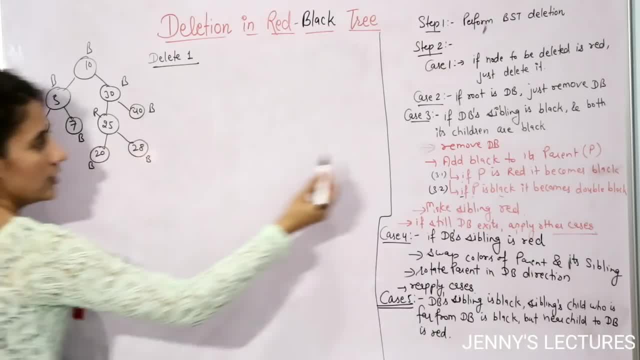 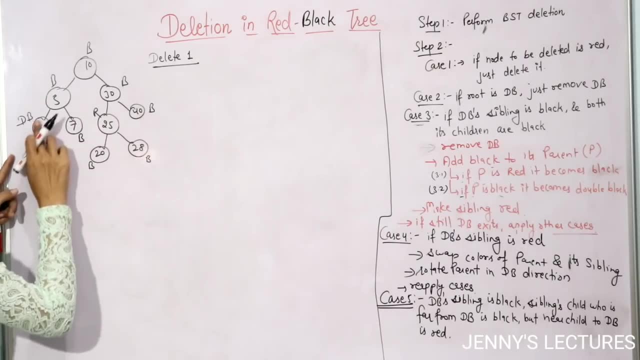 this is also black because these are nil. so now this case you will apply first of all, right, so now he'll give its problem to its parent. so now remove this double black. this would become single black, now null, and a parent is black, already black, so it would become now double black, right now still. 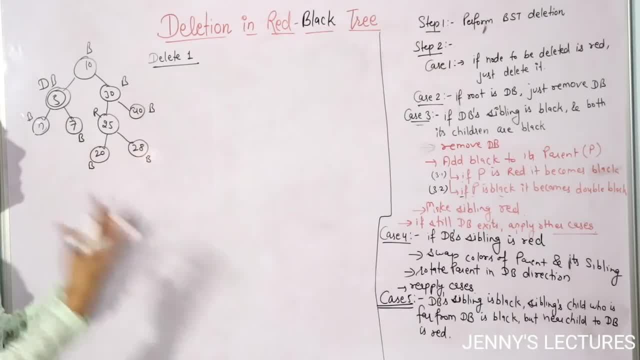 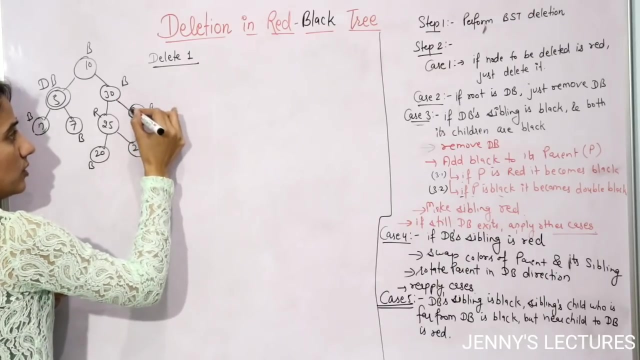 problem of double black exists. now reapply you cases. now find out which case you need to apply now. this is the node which is having problem. now check out the sibling of this node. that is 30, which is black right now. check out this node. sorry, this children of sibling. see it is having two children. which children is near to this double? 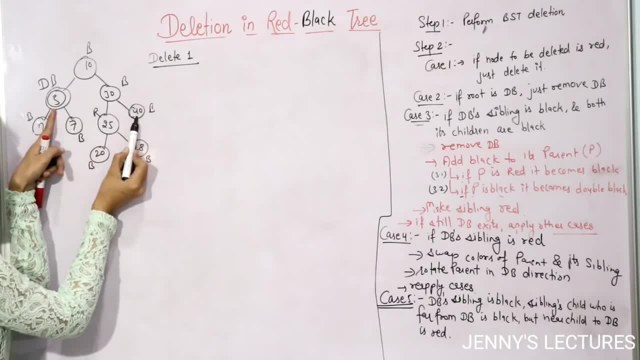 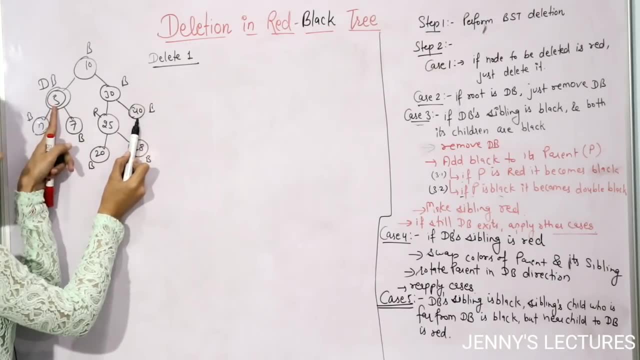 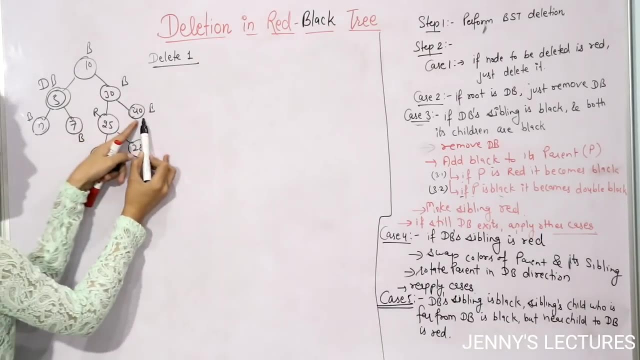 black node, this one and which is far from this, this one. so first you will check: sibling: this is black. now the child who is far from double black. this situation: siblings: child who is far from double black. this child is far from double black, this is near. so this is black, right, and the 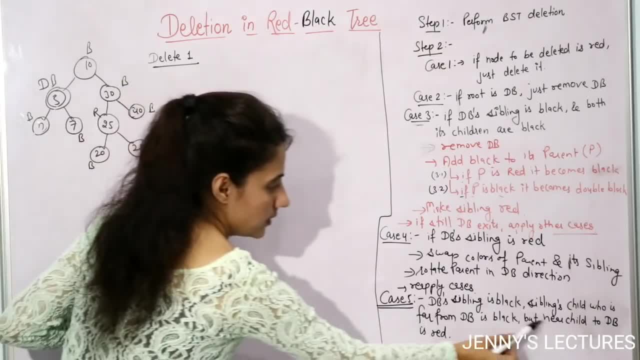 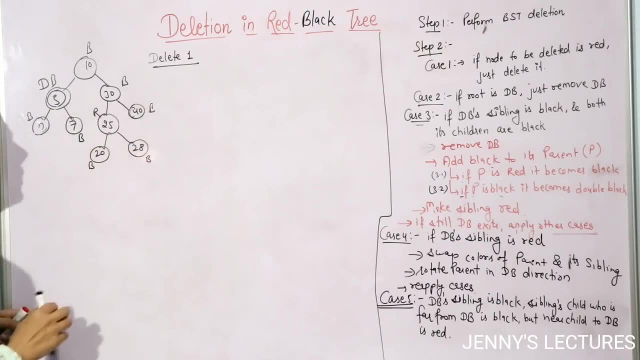 child which is near to double black is red and the but the near child of double black is red. now, this is the case. now, here, what you need to do see here i am not writing left child or right, because all the cases are the same. so i am not writing left child or right child, because all the cases are the same. 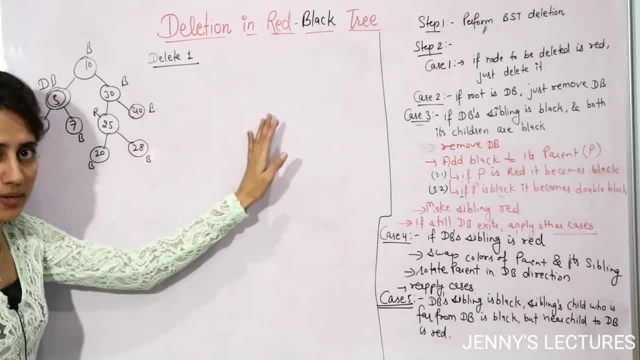 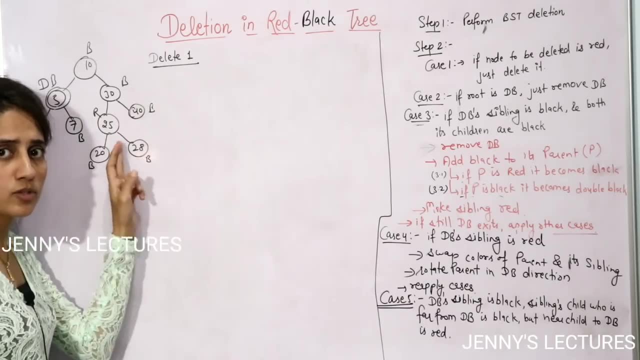 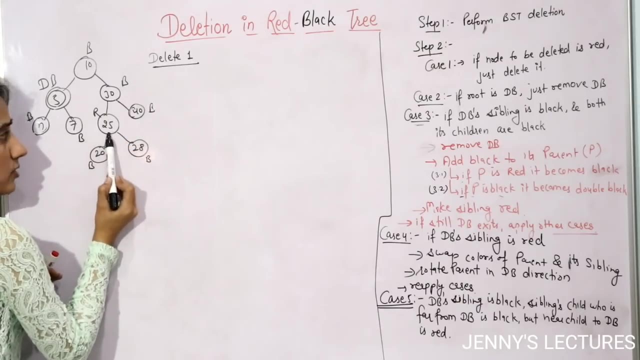 this case, or all the cases, are having its mirror image, right. so if you write down the left and right child, then that would create a problem in mirror image. so that thing also will discuss the mirror image of this thing. fine, now see this siblings child is red means he is angry, right? 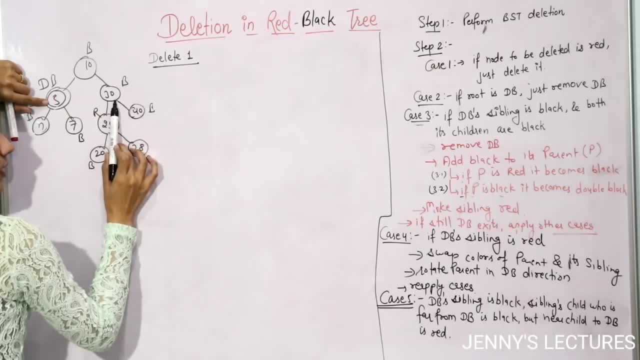 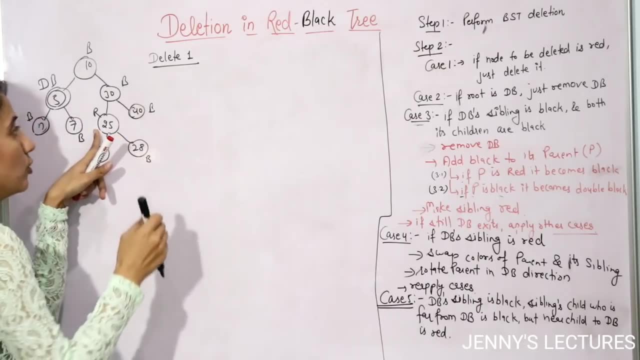 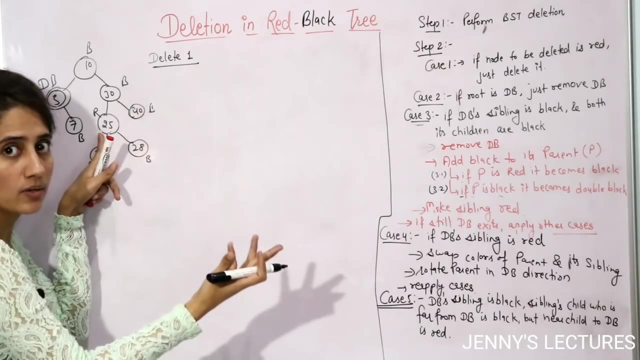 now this double black node will ask to its sibling to go to his child and cool him down. right, so now the parent will go to its child and cool him down, but in this process the parent would become angry. so you can say: you will swap the color of sibling and 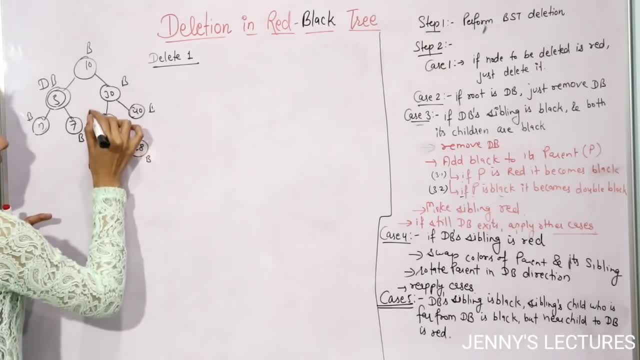 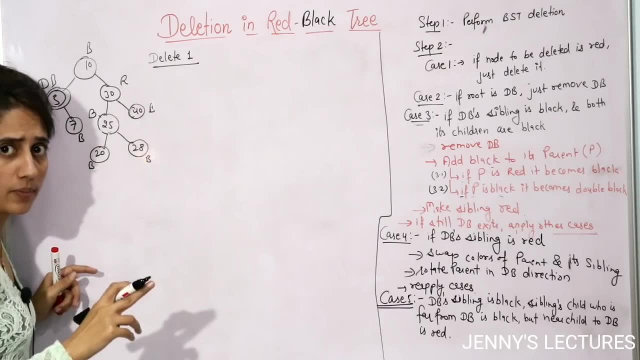 its child. so now this becomes black means cool down and this would become angry, right. this is the first step. now rotation: in this case also, rotation would be required. so now 30 becomes red right. or you can say 30 becomes 20.. so now 30 becomes red right. or you can say 30 becomes 10.. 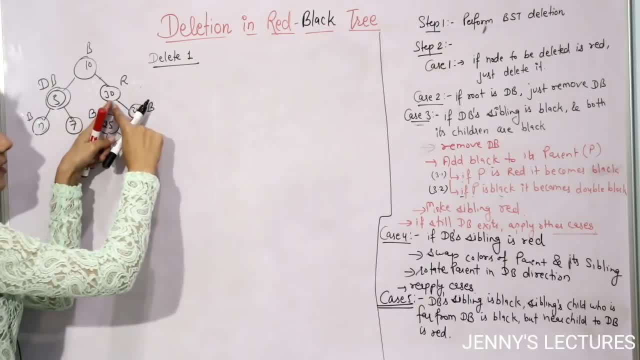 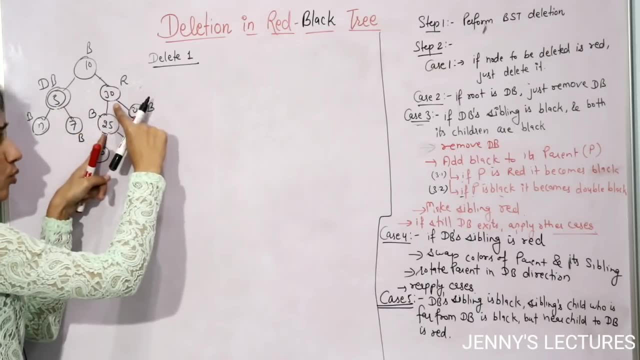 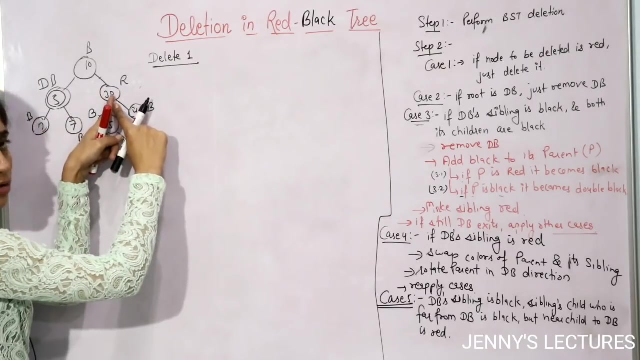 the middle 1?? the middle 1 is your child's own red colour and that is c angry. and why he becomes angry? because of because his sibling- 30 sibling is 5- because his sibling asked him to go to his child, to his child and cool him down. that is why he becomes angry. so 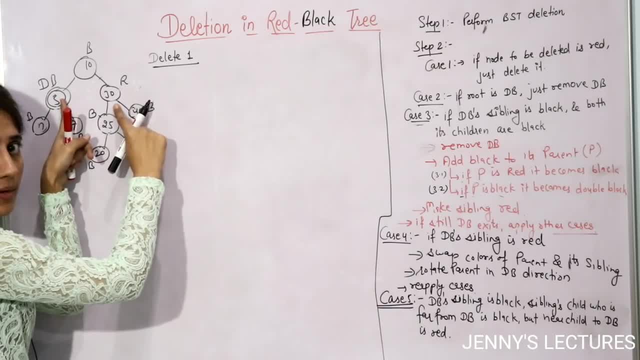 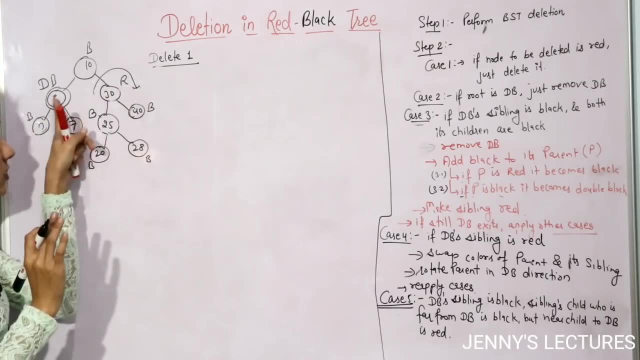 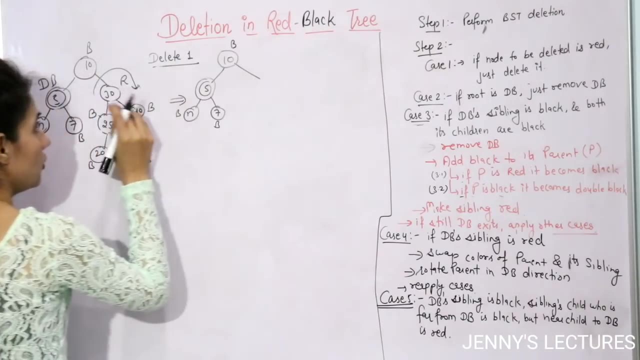 you can say he becomes angry with its sibling. that is why 30 would rotate in opposite direction to its sibling right, not in this direction. opposite direction to its sibling. now, the tree would be something like this: so now, when you will rotate this 30 in this right direction and 30 would be: 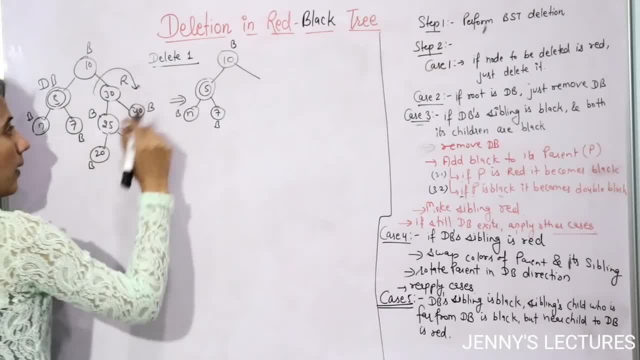 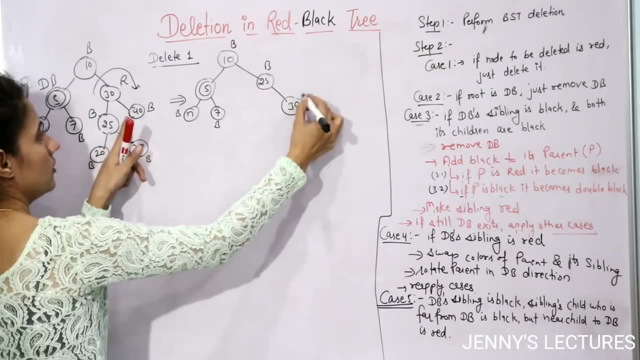 downward and 25 would go up. so 25 is here now having color black, 30 is to the right of 25, that is, 30 is having color red. here we have 40, and to the left of 25 we have 20, 20. 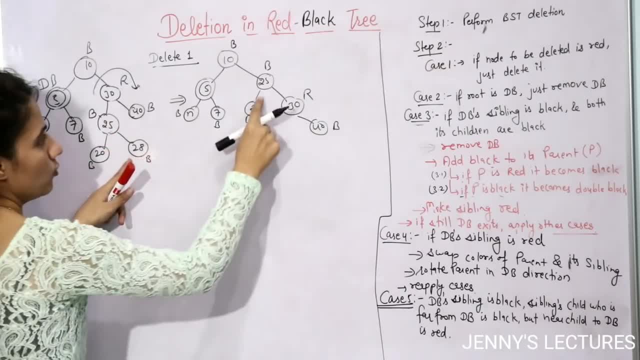 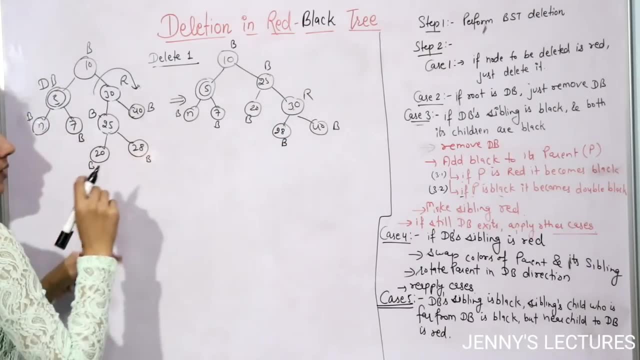 20, 20 with color black and to the right of 25. we have 28, to the right of 25 and to the now to that left of 30. that is here we have 28. that is an black color. now still we have problem of double black. 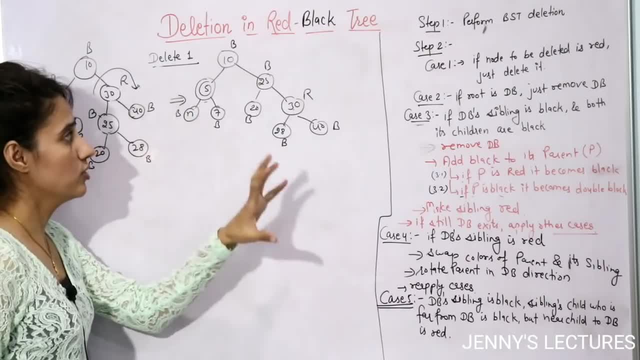 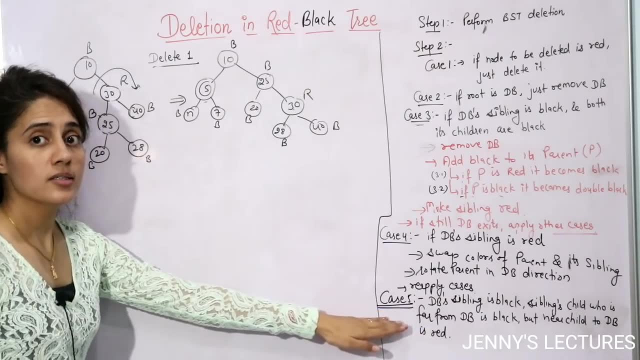 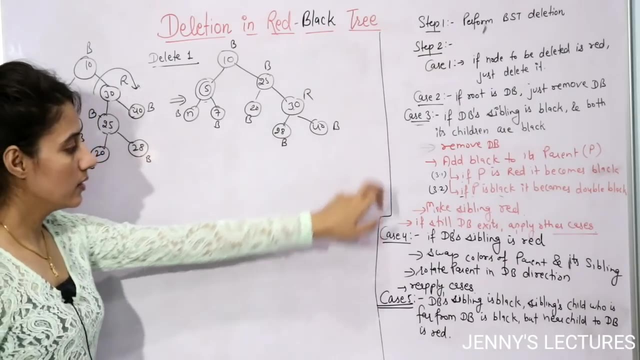 situation. now, again, you need to find out which case you need to apply right. and after case 5, definitely you need to apply case 6, that is for sure right here we have applied case 5. first of all, we applied case 3, then we apply case 5 and now you need to apply case 6. now, what is case 6? 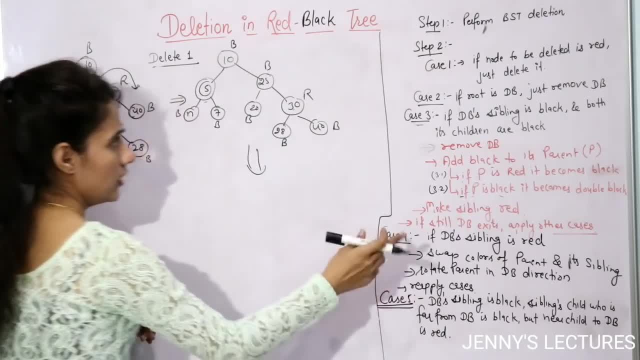 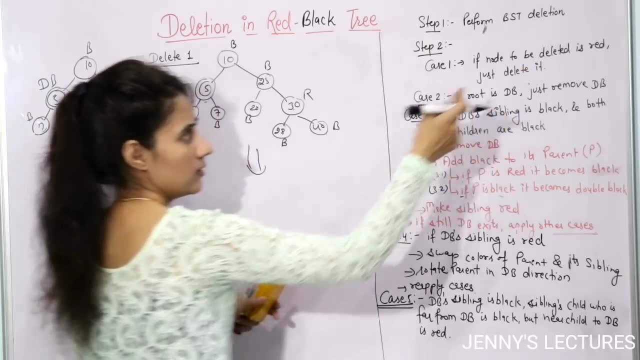 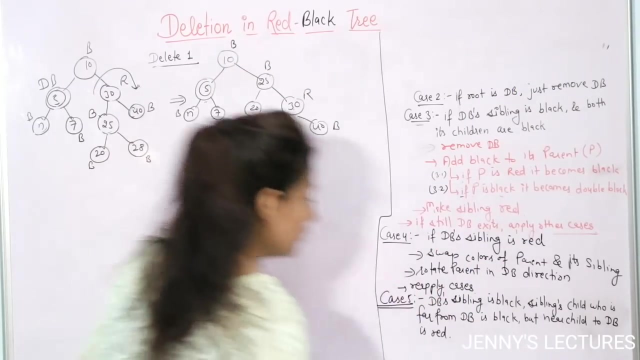 see, first of all, write down the steps of this case. i am writing the steps here because, see, this step is very simple, and this is very simple because if node is deleted you want to delete is red, simply delete it. so i am writing the steps of this case here. first of all, what we have done: we simply swap. 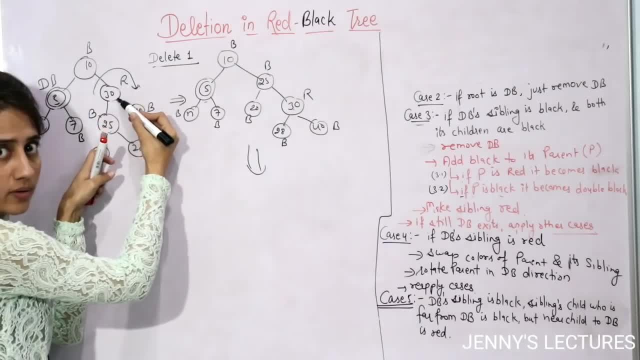 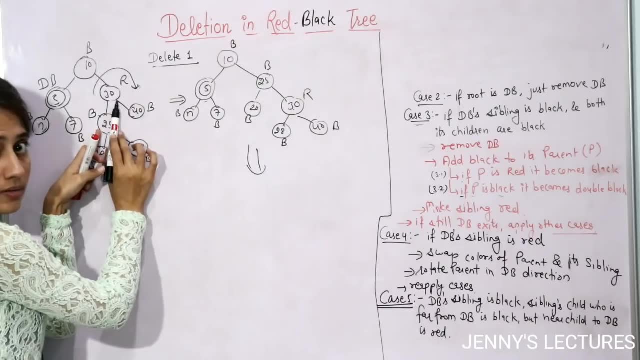 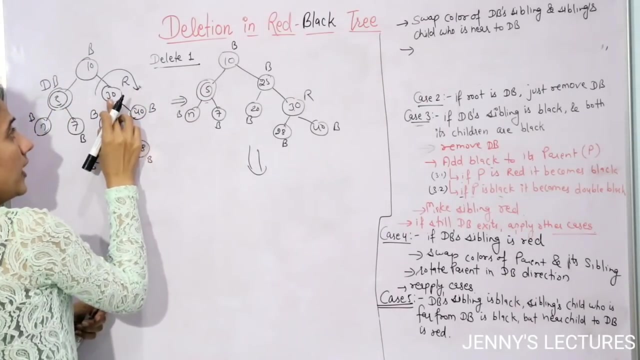 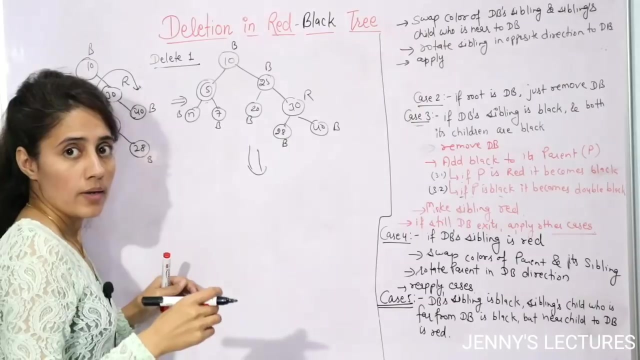 color of see this one and this one right means color of db's sibling with its child who is near to db. now, after swapping the colors, what we have done, we have rotate the sibling of this db in opposite direction to db, not in the direction of db. so now and now still, the double black problem exists. 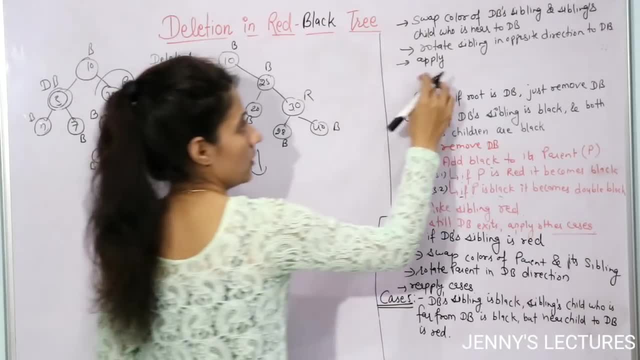 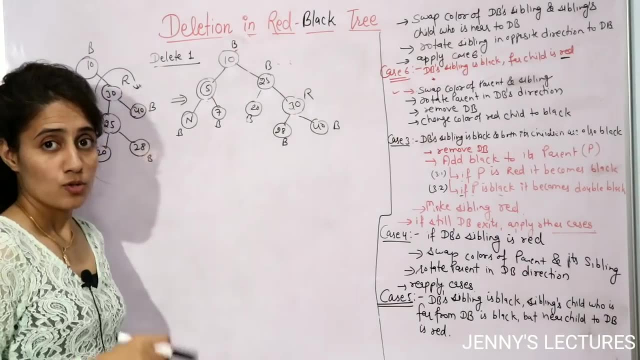 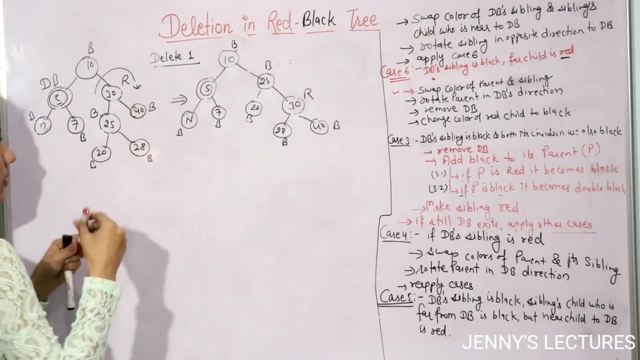 and definitely you need to apply case 6. so here you can write down the steps of this case 6 and down apply case 6 right now. what is case 6? see? so now we will discuss case 6 after applying case 5. this would become this thing: i guess this would be red right, because when you will this double? 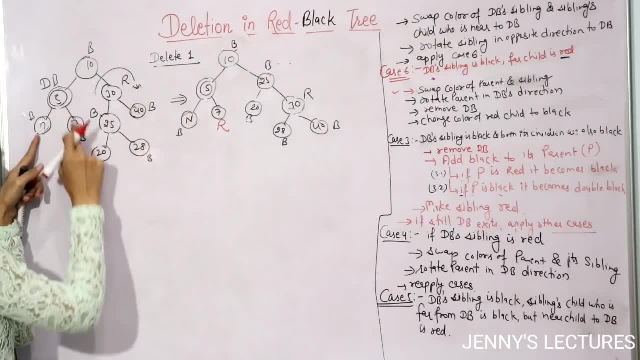 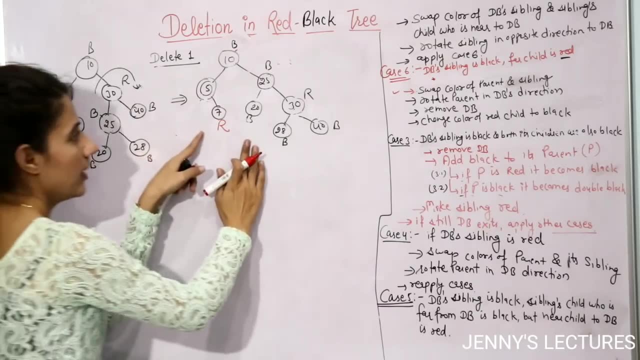 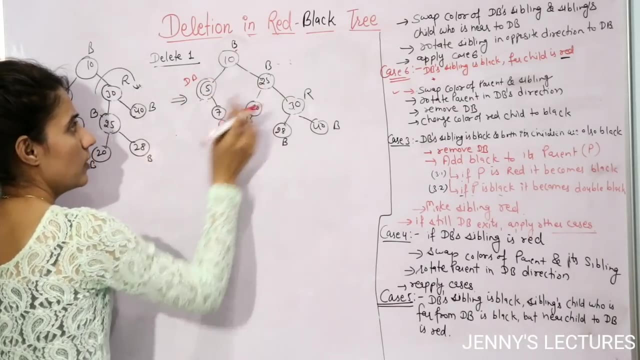 black. this node will give its extra black to parent. then the sibling becomes angry or you can say it becomes red. now this is nil, so you can delete it. so now this is the tree. now here is case 6. now we will discuss. see, this is node having double black situation. now check out the. 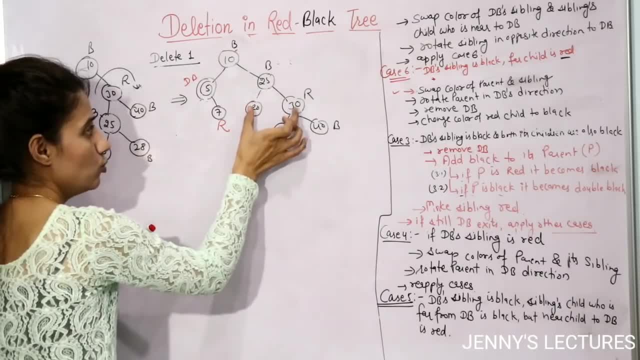 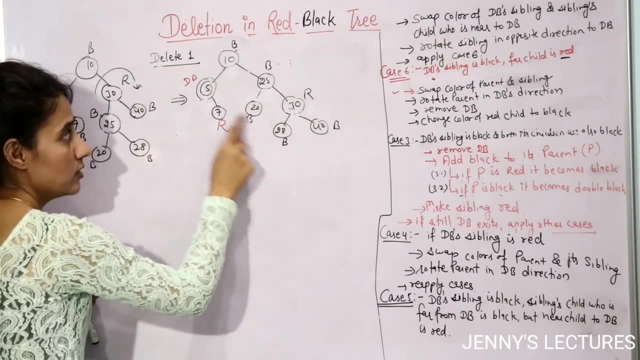 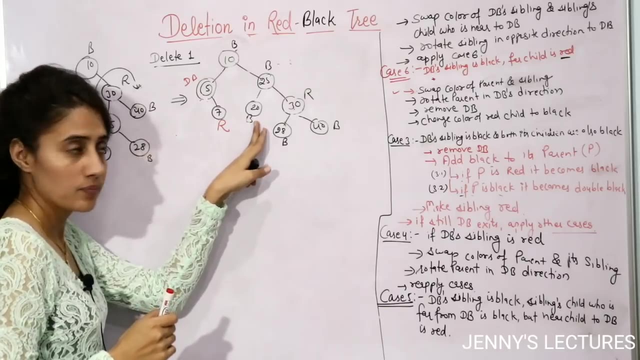 sibling of double black. this is black. now this is having two children. so first of all, you will check the child who is far from double black. say, this is far from double black, this is near to double black. so now, this far child is red now. now no need to check this child, right, if you find this. 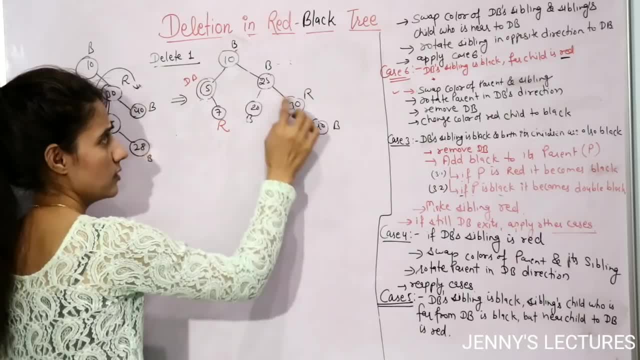 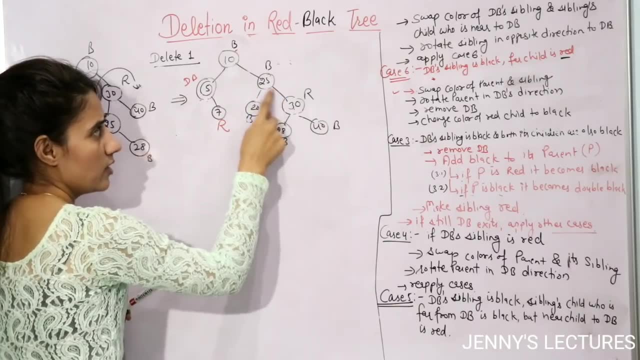 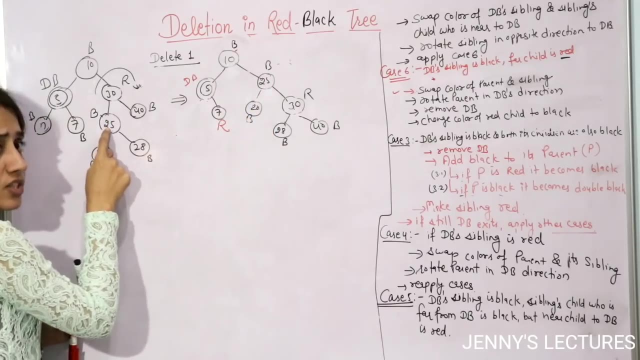 is red. now you have to do something. now you can say this siblings with the far child. or you can say: this child is angry, so now he'll not directly go to his sibling and ask to cool his children down. if the this, this was this case, this was the case, if this child, the near the near children, was red. 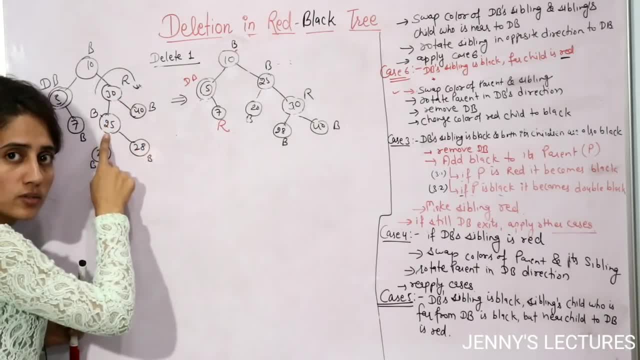 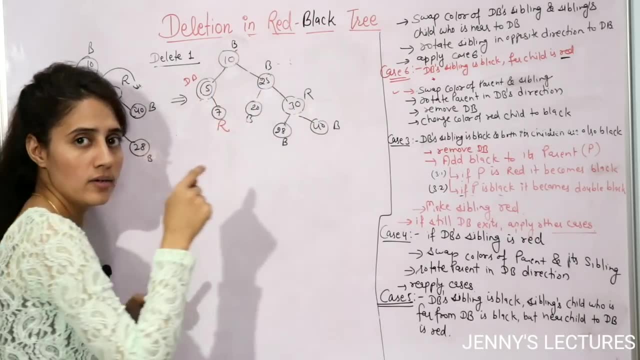 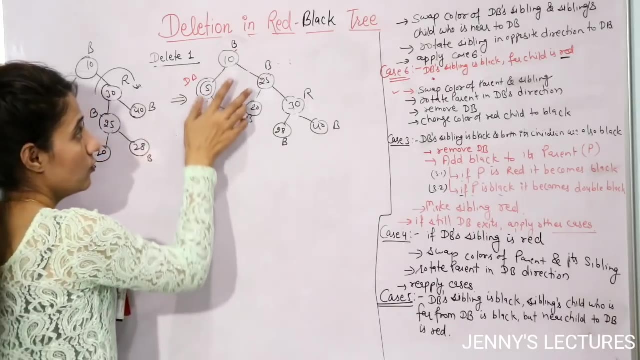 then he will ask to its sibling to go to his child and cool him down right now. this is the far child, so he'll ask to its parent to go and calm down his children right now. if the parent will go, in that case we will swap the parent and siblings color here. both are having black and black, so swapping. 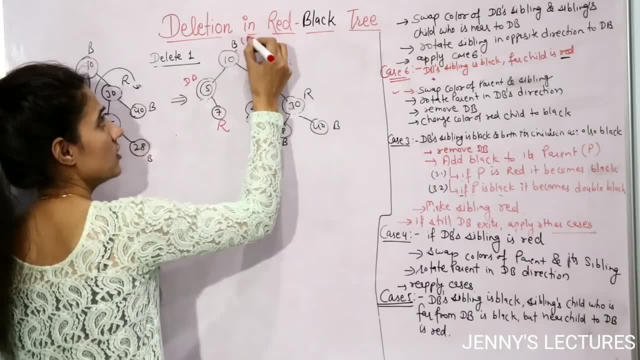 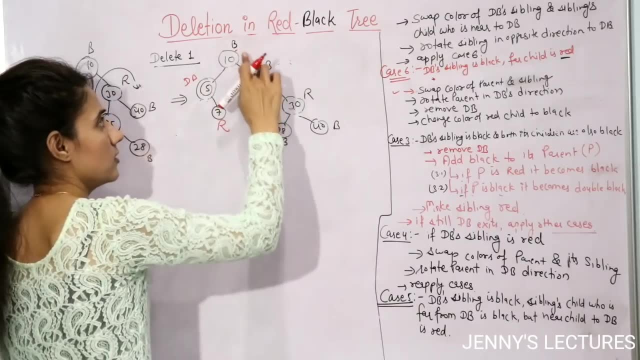 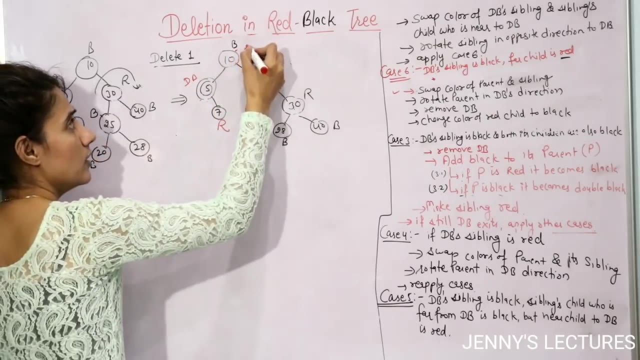 doesn't affect anything now. if situation is something like this: if this is red and this is obviously black, in that case this would become black, this would become red. but here this is not the case. both are black, so no swapping would be there right now again. next step is what? now he'll. 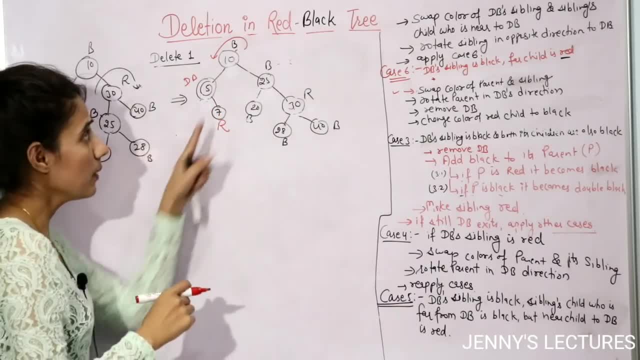 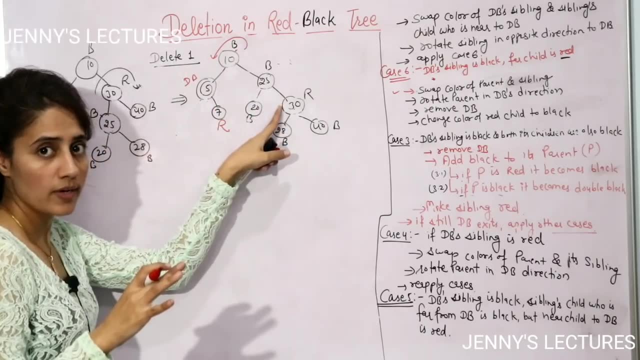 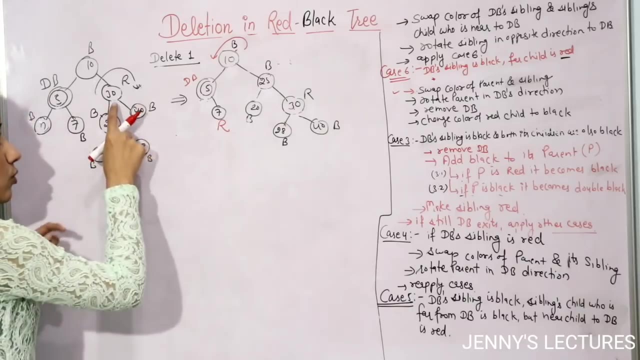 rotate towards DB direction because in this case, 10 then is the one who went to cool him down. right, so this would rotate. in this case, 30 rotated. why so? because 30 went to cool his children down. that is why he will rotate and he was sibling of double. 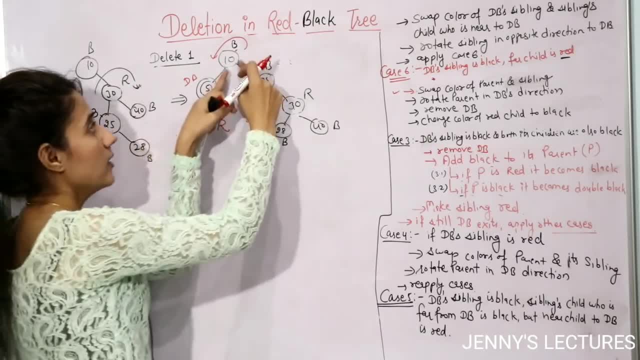 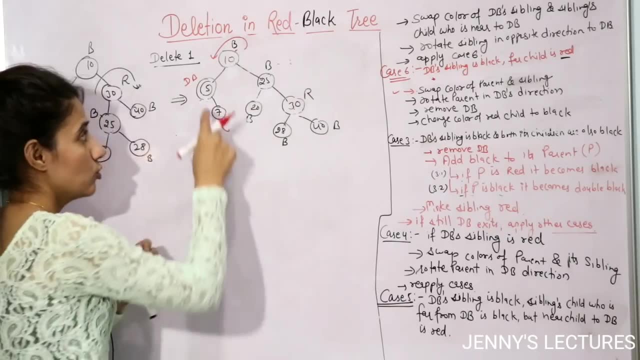 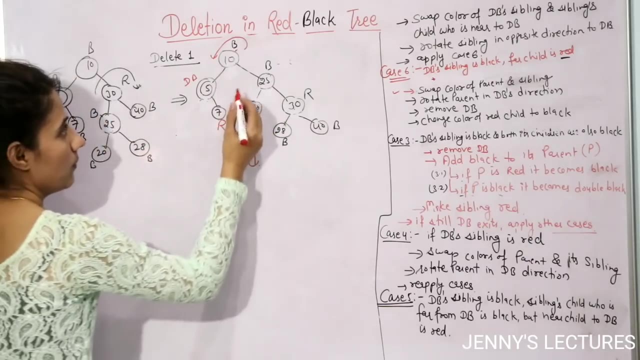 black. that is why rotate in opposite direction right and it is parent of double black. so parent always rotate towards the child which is having problem right. so now this is having problem, so he will rotate towards this direction right now. after rotation the tree would become 10, would rotate it towards this direction. 25 would go upward. 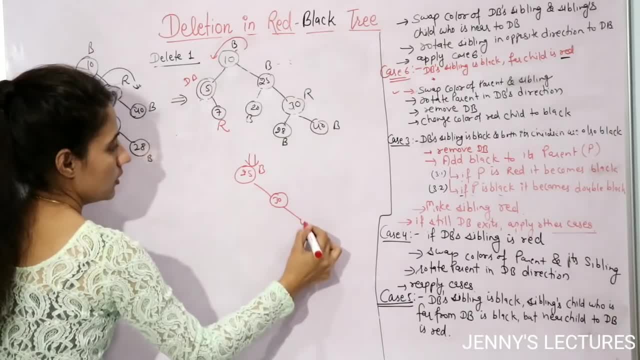 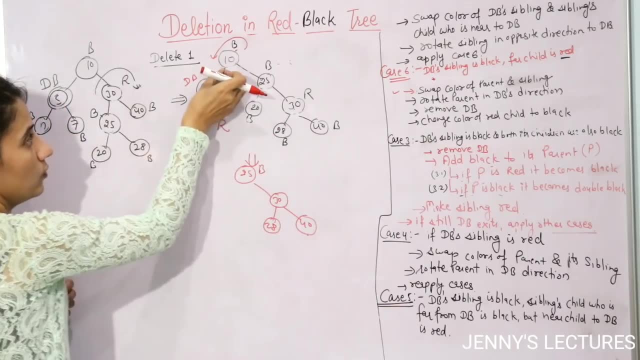 25 is black. now here we have 30, 40, 28, 20 is to the left of 25, but to the left of 25 when you will rotate this tree. so now here we have 10. so now 20 would be to the right of 10. 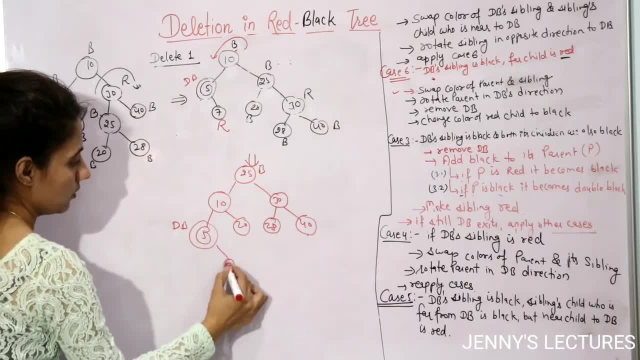 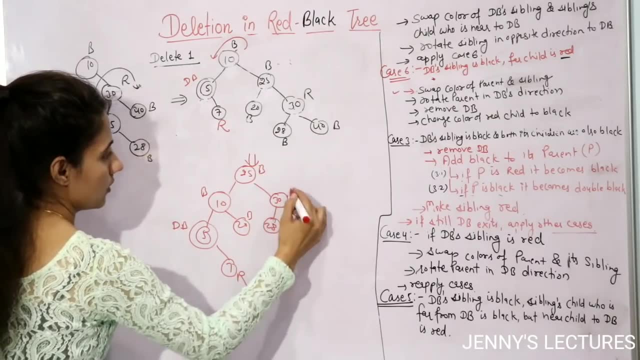 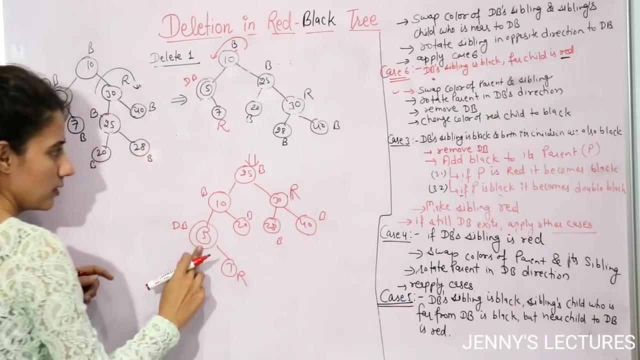 so now 20 is still having the problem of double black. and here we have 7, that is red and this is black. this is black, black. 30s, red, sorry, this is black and this is black. now next step is what this? remove this double black. why so? because see this double black. 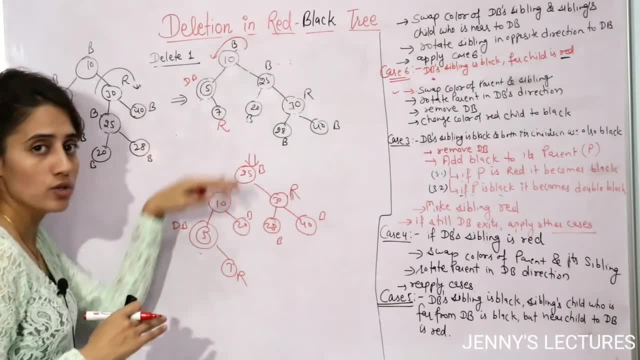 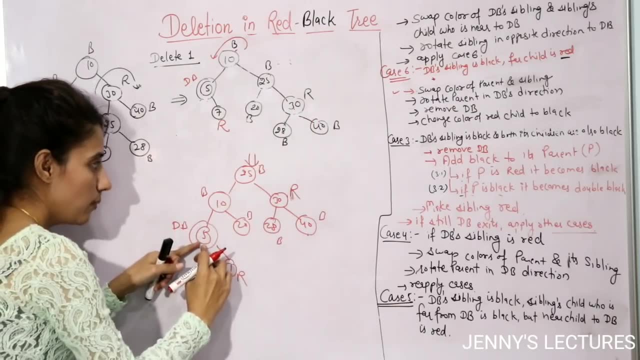 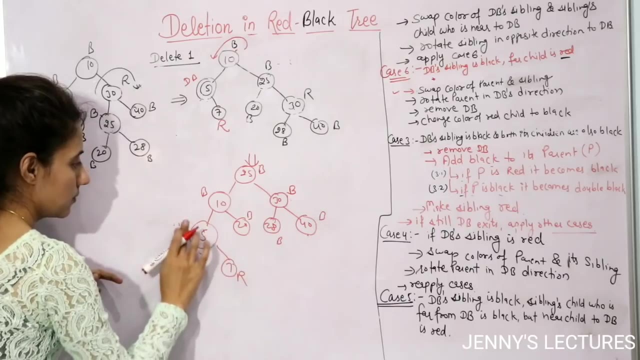 node can push his double black problem upwards, not downwards. now the problem was, the far child was red. he will give its extra black to 30. So the 30 would become now black and this would become single black. and that's it. Now you can see this is a red black tree right after applying case 6.. 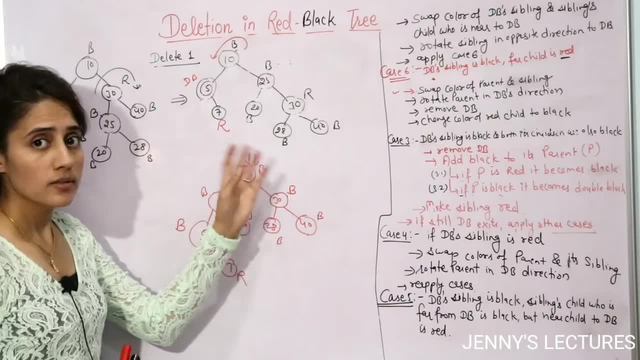 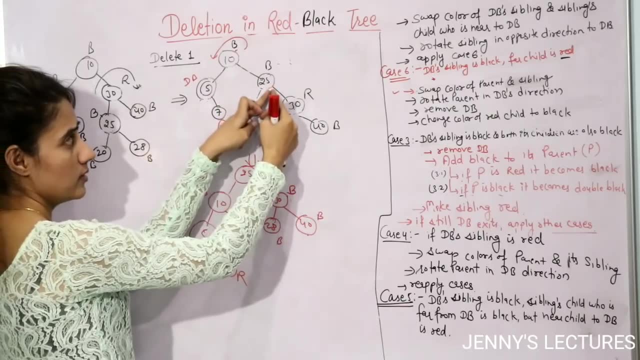 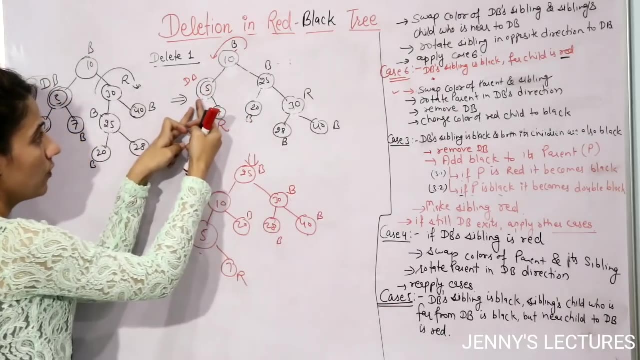 So now these are all the cases, and these cases are having its mirror image, also like this: Here the db is in this direction, but suppose db is in this direction and this direction we have sibling of this db, right. So now the far child of db would be this one and the near child would be 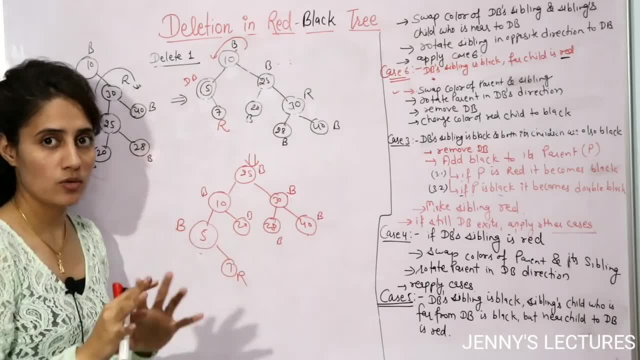 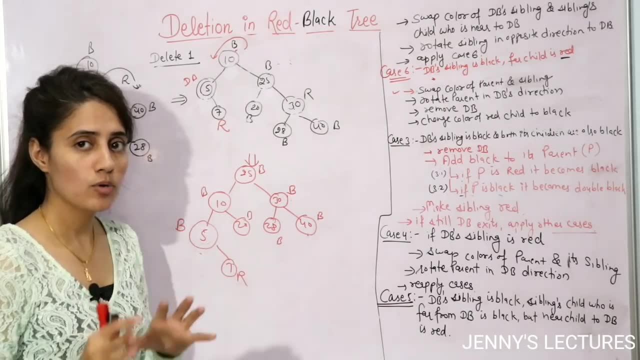 this one, right? So you need to take care of this thing also. but apply the same rules in mirror image also, right? So now we will take one example and we will discuss the deletion process in red black tree. Now let us take this example and, one by one, we are going to delete these numbers, So 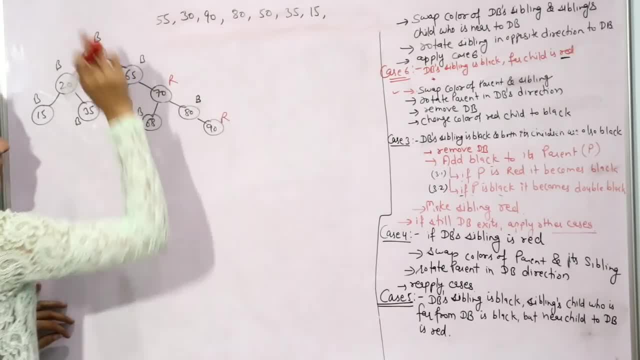 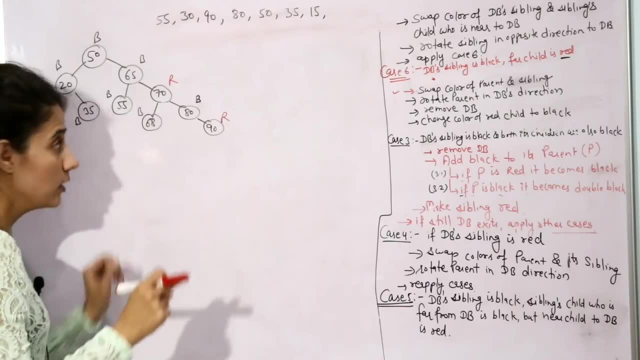 this is a red black tree, as you can see. Now, first of all, delete 55.. Search where is 55 from the root. 55 is greater than this, one less than So. here we got 55 right. You cannot directly delete it because this is black node, right? and 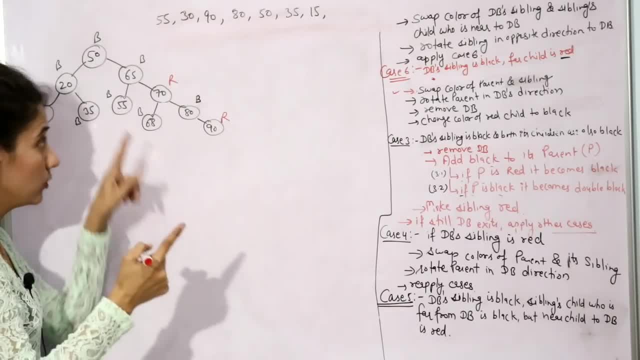 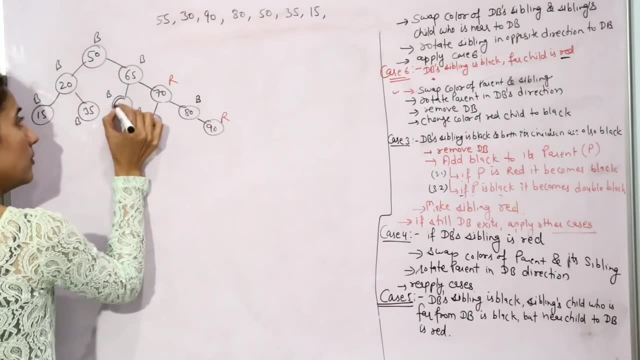 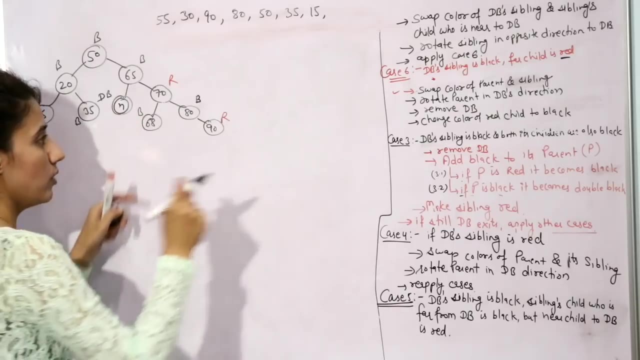 children, obviously nil and nil. those are also black. So if you will delete this thing, so we will replace this with nil, and nil is black. so that is why it will become double black, because this was already black. Now the problem is there. Now you have to convert it into single black. Now apply. 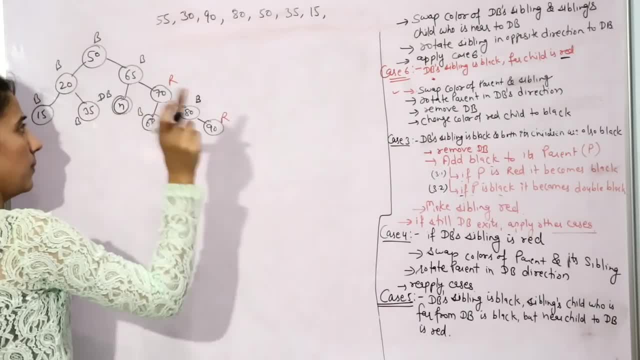 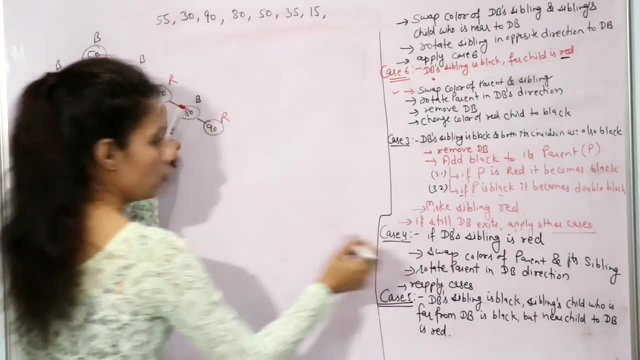 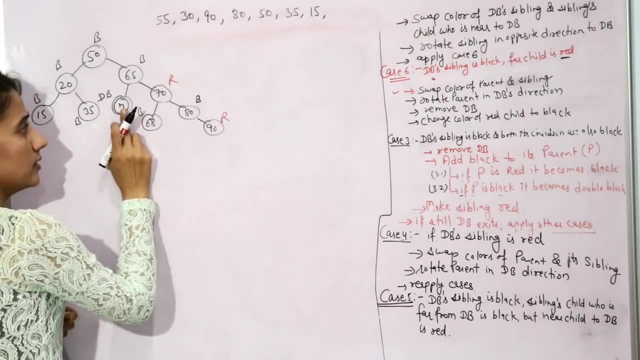 find out which case you need to apply. To find out this thing, simply you need to do, you need to check sibling of double black. Sibling is red. It means this case four you need to apply. It means sibling is angry, right, So now he can see, he can give its extra black to its sibling. but right now, 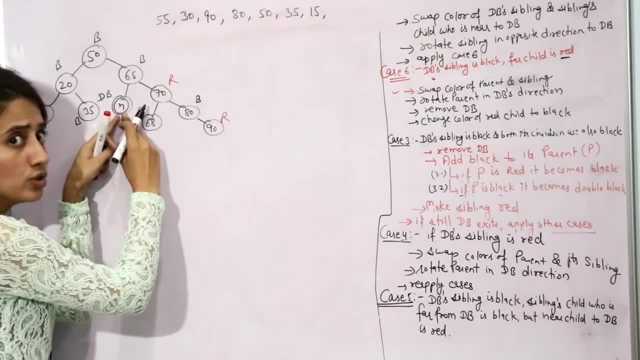 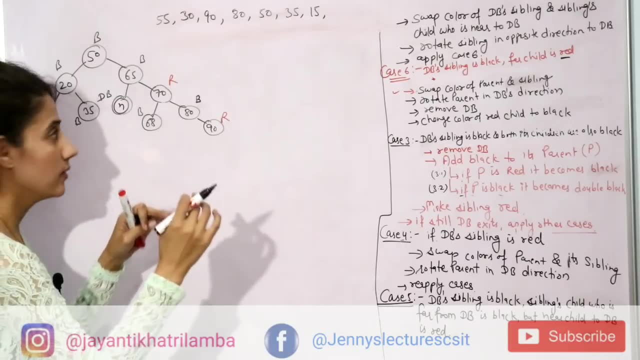 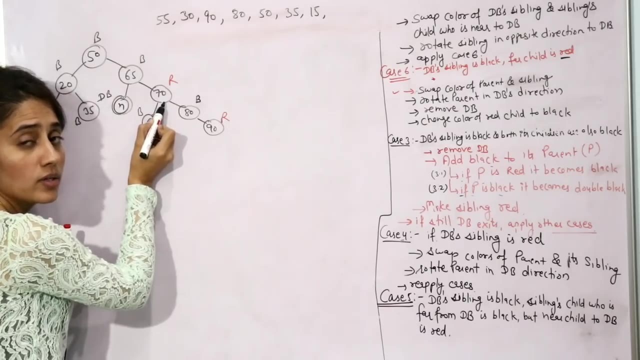 cannot give, because these are at same level and it can push its problem to upwards only right, not downwards and not at the same level. right, So now he will ask to its parent to go and cool his brother or its, his sibling down, right, So now parent will go. so that is why the 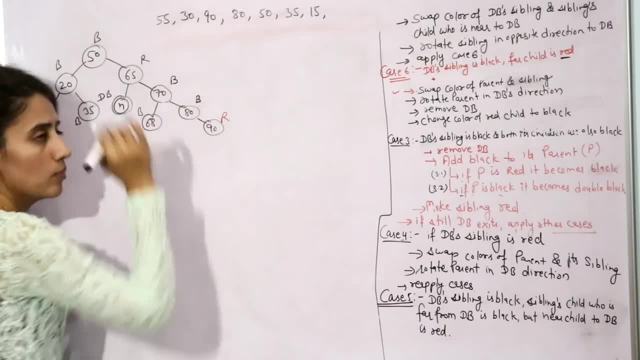 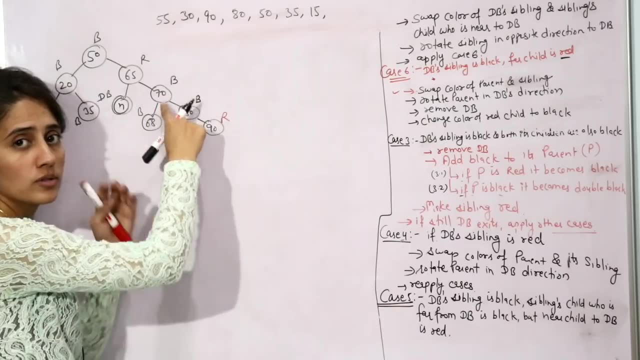 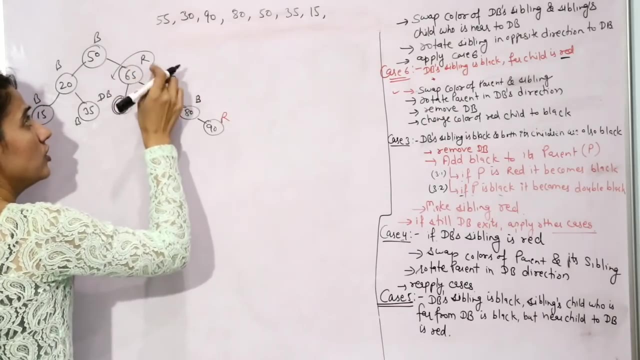 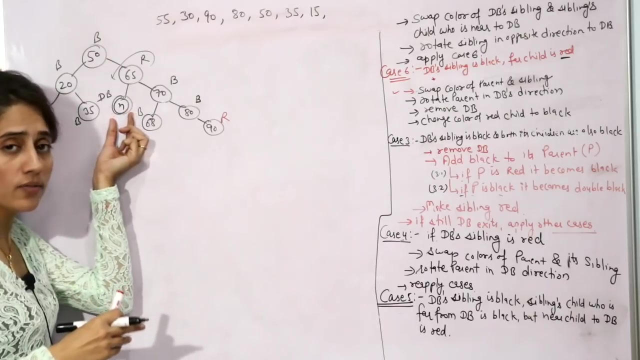 parent now become red and now it becomes black, because during this process parent become angry and that child who was angry becomes cool down now. Now parent is angry, So now parent will rotate. in which direction? Parent will always rotate? in the direction the child, in the direction of the child who is having problem, and now this child is having problem. 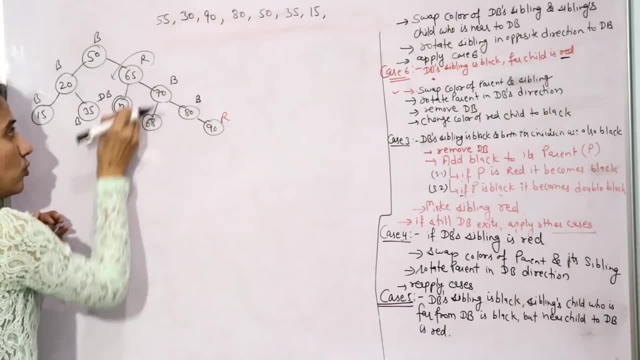 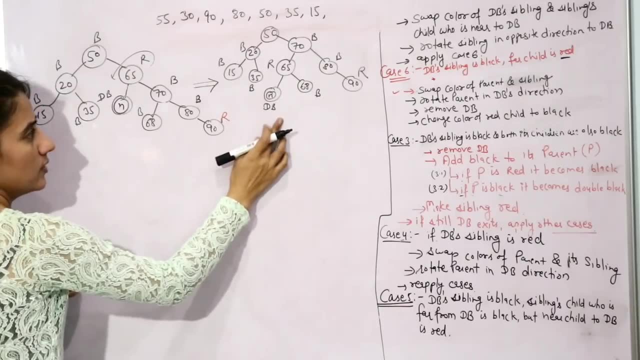 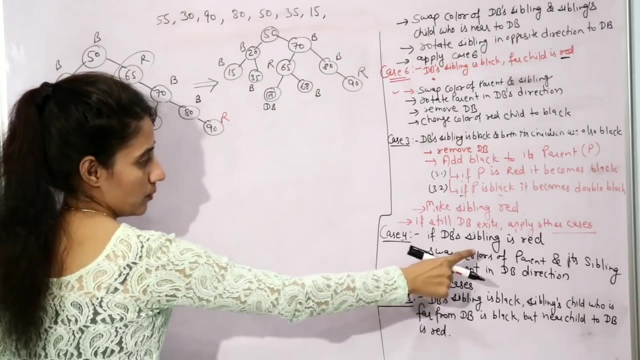 right, So parent will rotate in this direction. So 65 would go downwards, 70 would go upward- right, So now the tree would be something like this: So now this is the tree after applying case four. Still we have DB problem. See, we have done swapping of parent, color of that parent. 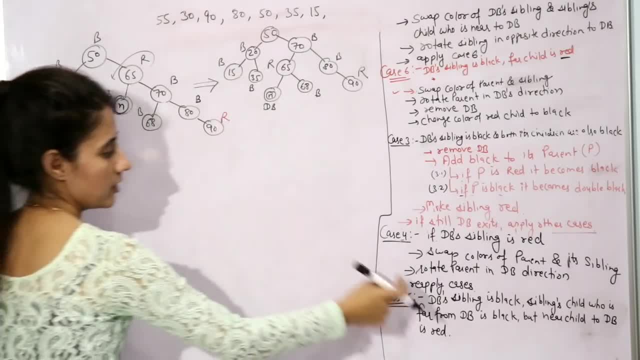 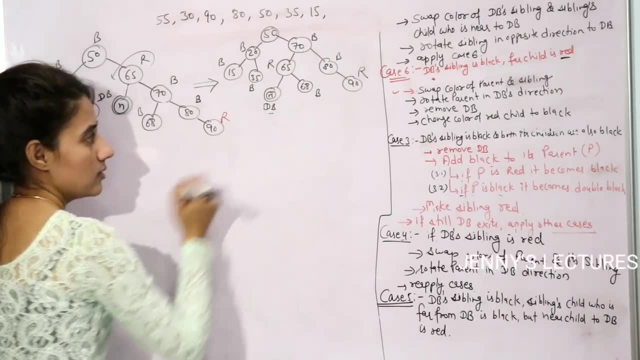 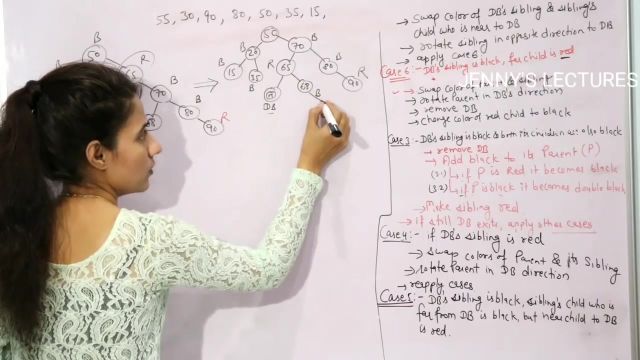 and its sibling Rotate. parent in DB's direction. Now you have to reapply cases. Now again check which case you can apply. So now in this case, Now DB is this one, this node is having DB problem. So first of all check the sibling. Sibling is black. Now check the, the child. 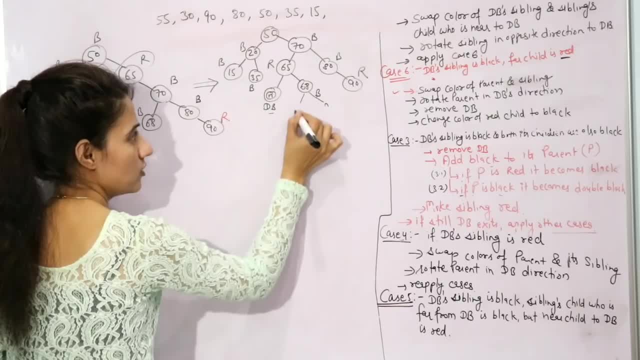 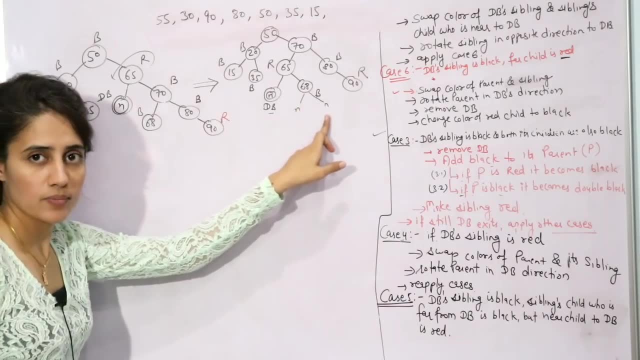 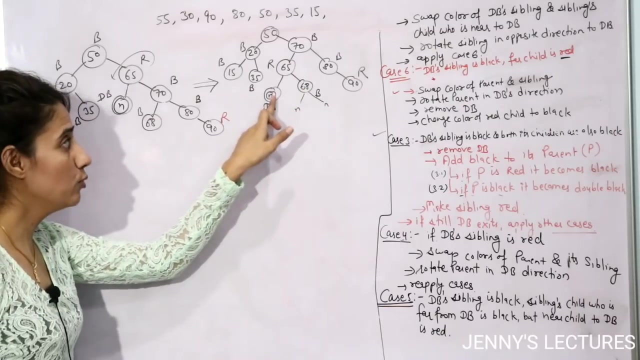 who is far from this DB. that is nil, that is black. and this is also nil, that is black. So now you will apply case three: This is black, this is black, this is black, right. So now he cannot give its extra black to any of these. So now what he will do? He will push his problem. 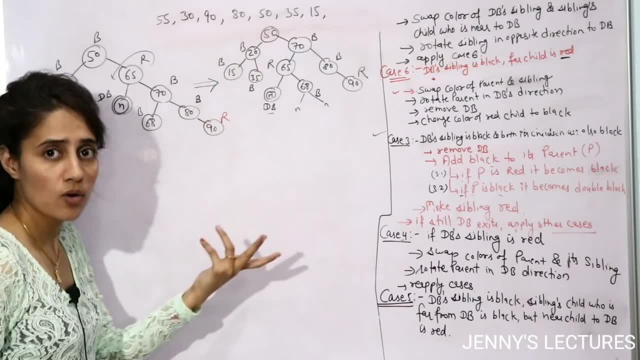 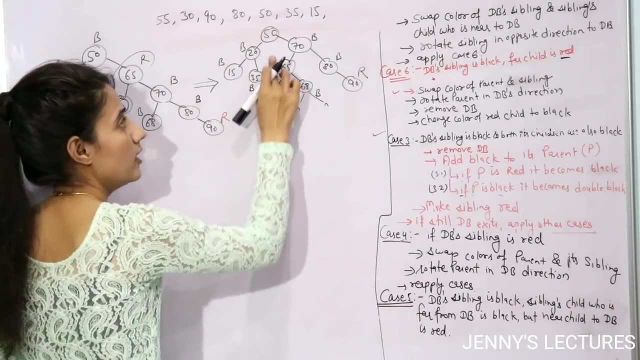 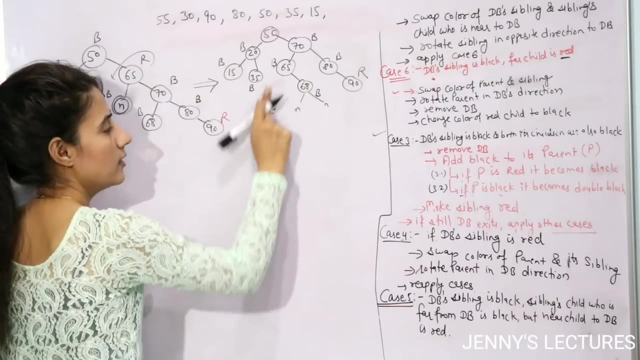 upwards, he will push the extra black to its parent, obviously right. So now the parent is red, See 65 is red. So now this parent becomes black and this will become single black and this is null. That is why you can delete it. Means, we will not write this thing. 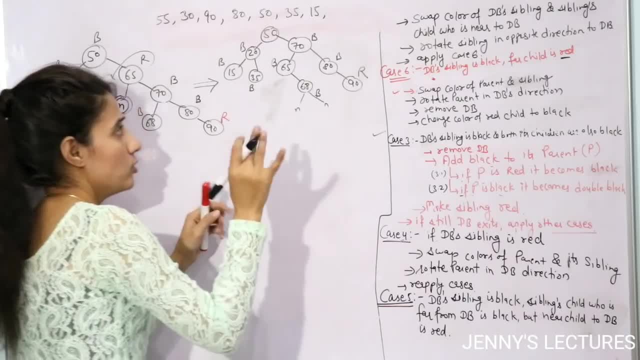 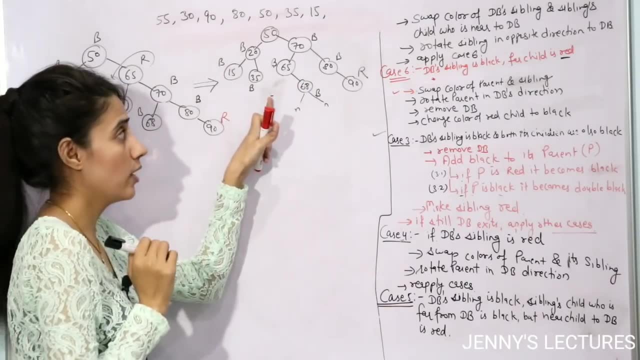 right, We have solved the problem. Now one more step. one more step is what now? this children has given its problem to parent. Now, after looking at it, That is right, this one, the sibling, becomes angry. he will say: why you are giving your problem to our parent. 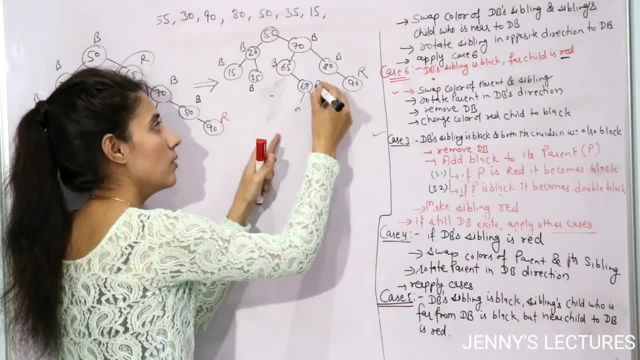 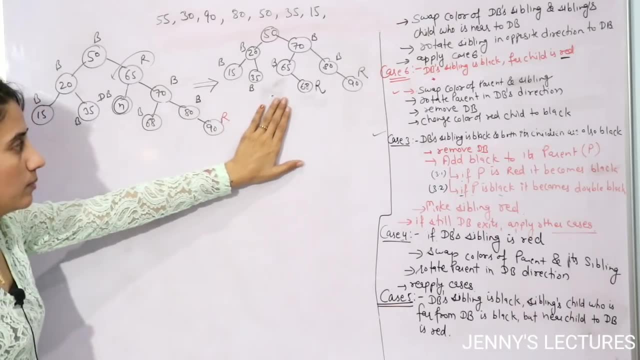 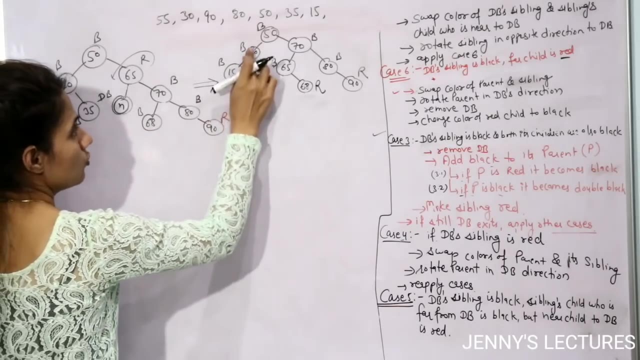 right. so now this was black, so it would become now red right. so now this is the tree, because here now we don't have any double black problem. so after deleting this 55, this is the final red black tree. so now, next you delete 30. so suppose this is not 20, this is 30. so now we 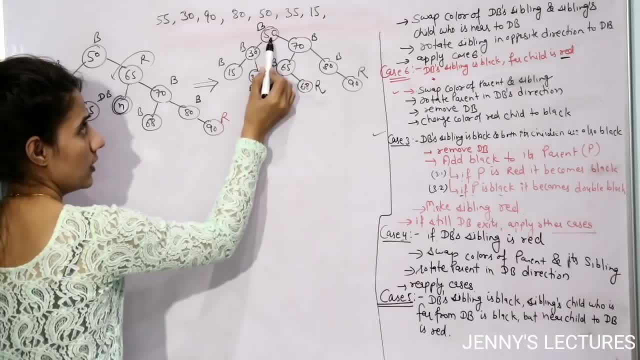 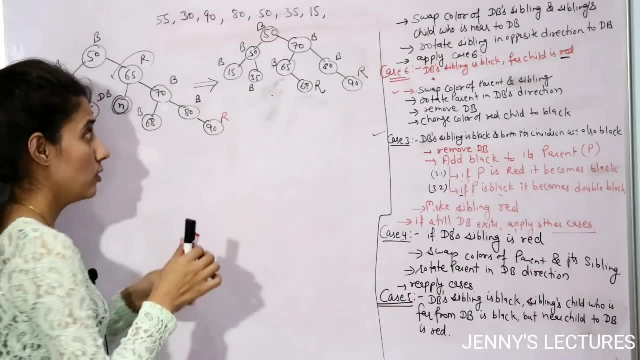 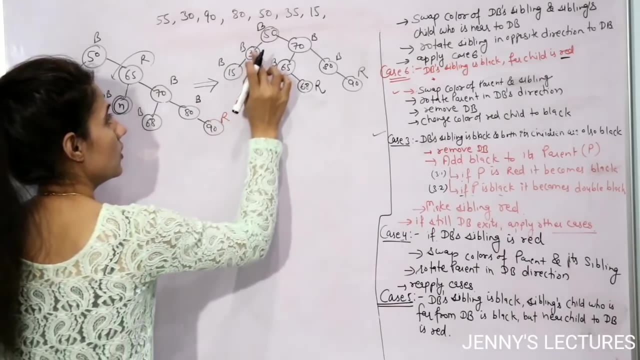 need to delete this one. first of all, find out where is 30 less than 50. so here we got 30. now 30 is having two children, so we will replace it with in order successor. in order successor is 35, because in the right sub tree only one node is there that is 35. so we will replace this 30 with. 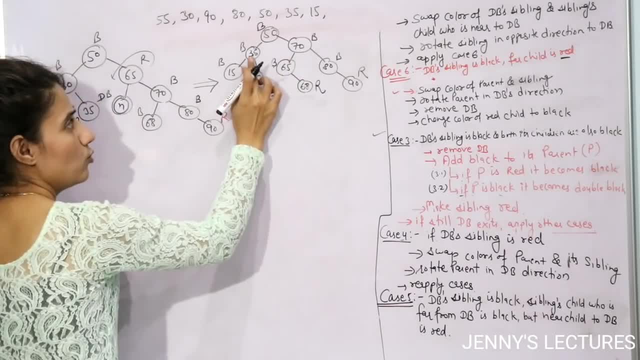 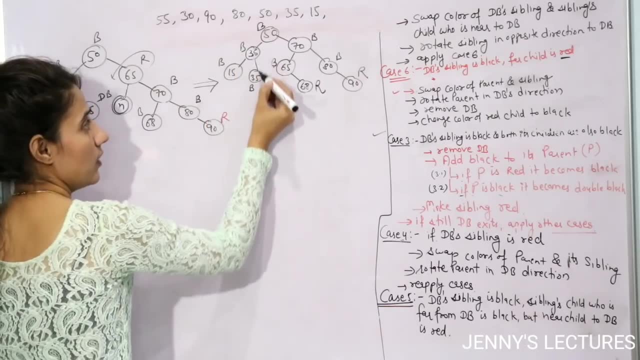 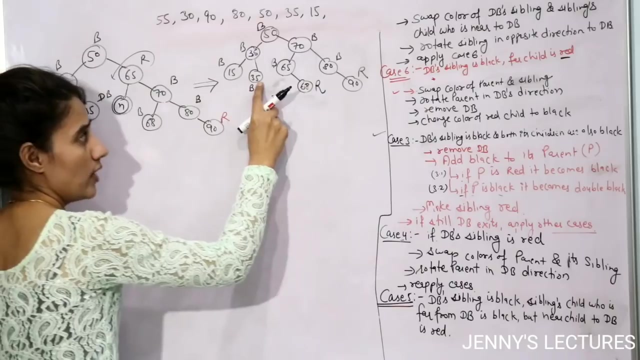 this 35 right and if we are going to replace it, we are not going to delete the internal node. that is why it will having its own color. that is black. only now 35. 35 to 35 are there. so now recursively called: delete on this in order: successor right. so we cannot directly delete. 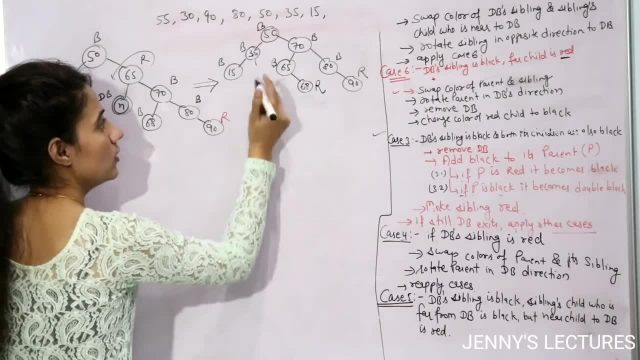 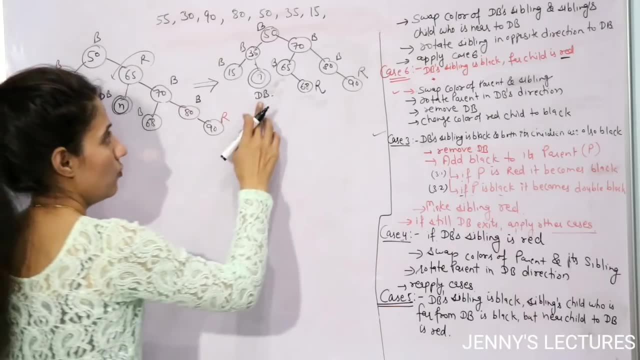 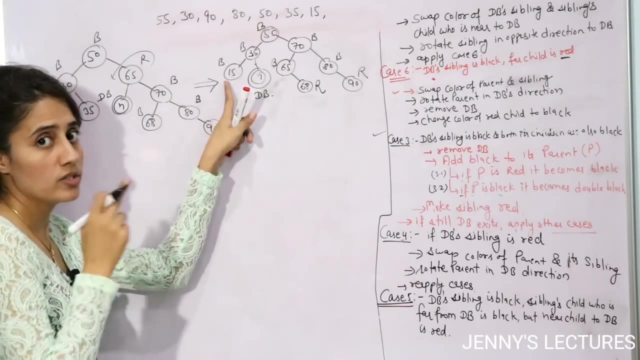 it because it is already black. so now we will replace it with nil and it would become now double black. right now the problem occurs now which case you need to apply. see now, check the siblings of double black. now sibling of double black is this one. so this is black. it's first of all check the. 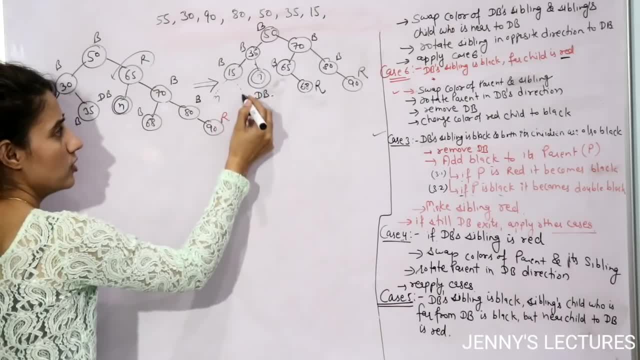 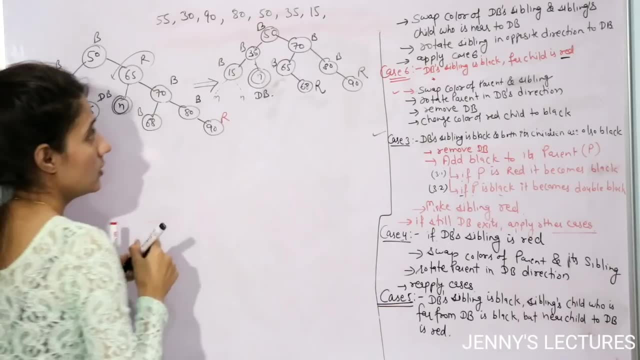 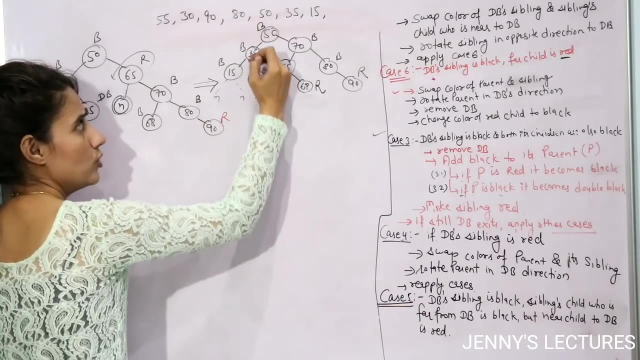 far child, this would be nil, that is black. near child, this is also black. now again, you will apply here this one case three. now in case three, what is the situation? see now, this double black will push its problem upward. you can say to its parent: because these are all black, no red is there. 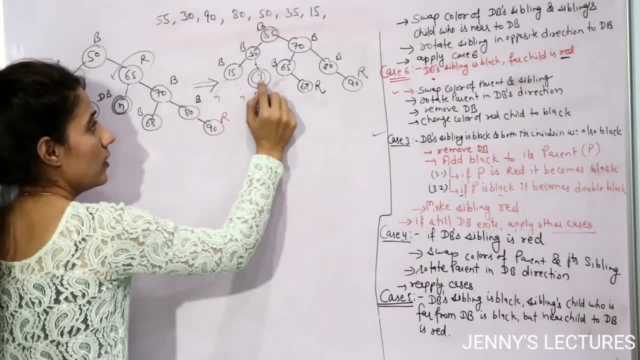 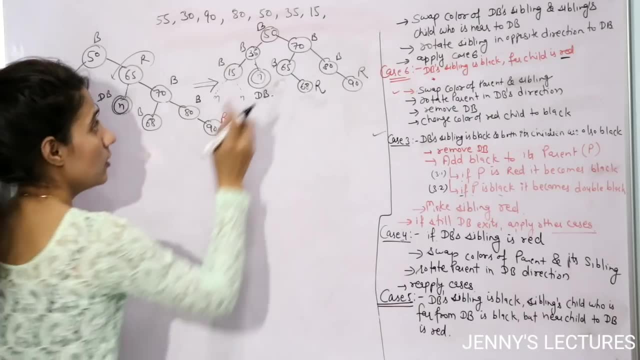 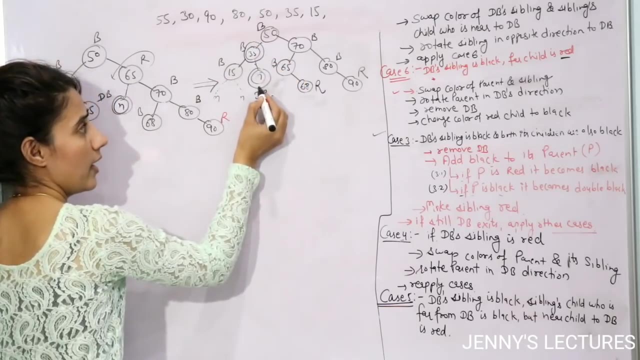 right sibling and its children. so now he'll give extra black to its parents. so now it third would become double black, right? so i'm updating here only now. this is 35, so this would become double black because this was already black and one extra black he has given to its parent. 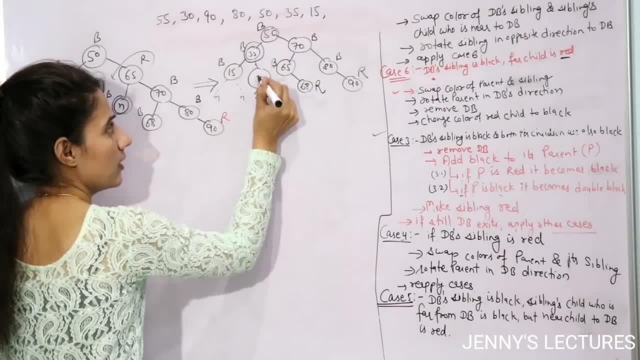 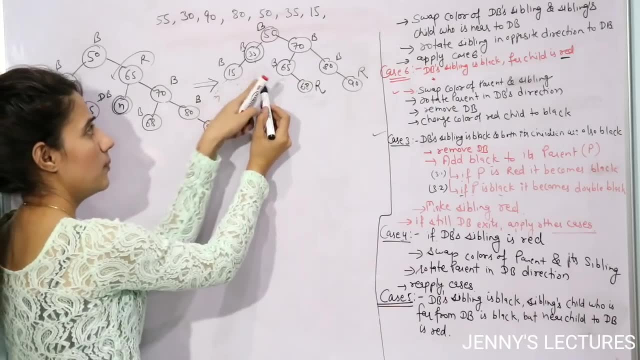 so it would become double black. now it would become single black. that is null. so if it is null, so you can no need to write down the null. now, after seeing this, the sibling of double black would become angry. that why you are giving your problem to our parent. 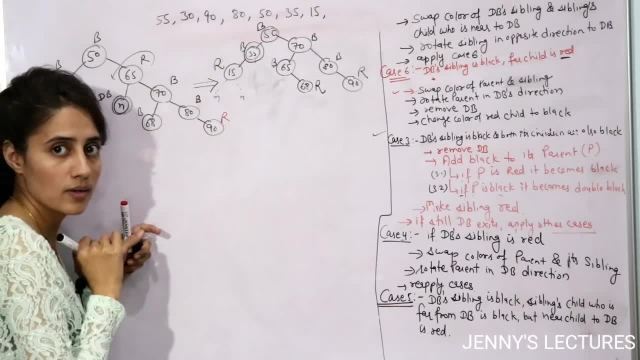 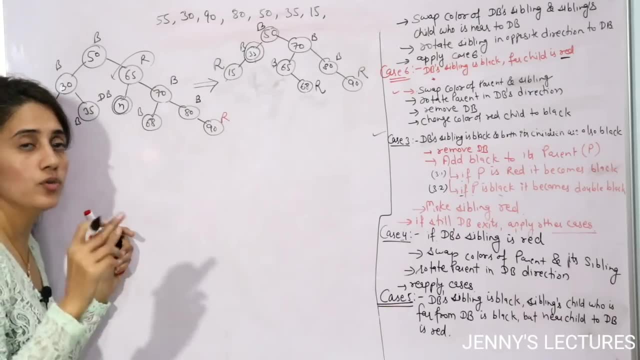 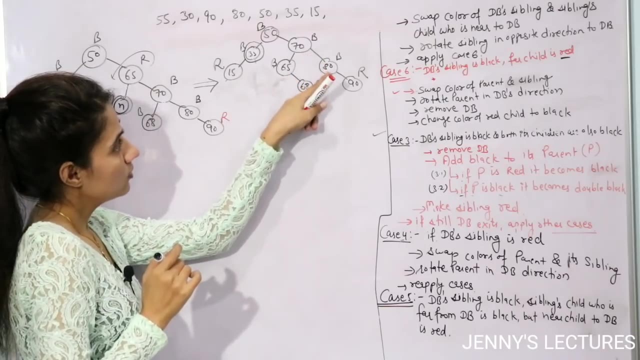 so that is why it will become red right now. still, the problem occurs now. double black problem is here now again. check out which case you need to apply now. check out the sibling of this one sibling is black right now. check out the far child from this double black. this is also black. now check. 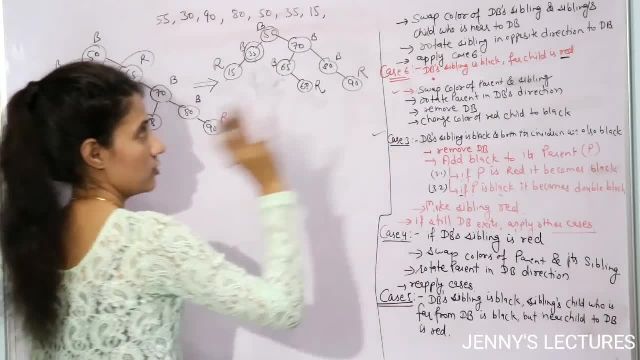 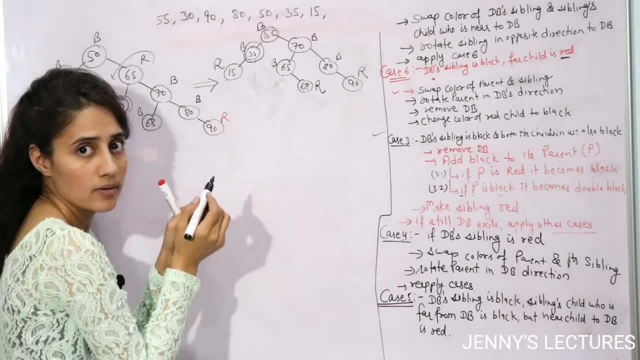 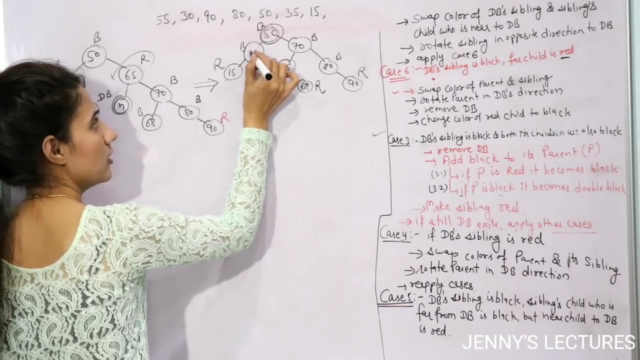 out the near child. this is also black. now again, you will apply this case only right now. it will give its extra black to its parent right now. the parent would become double black now, 50 would become double black and it would become single black- that is 35. only after seeing this, the sibling of double black was this: 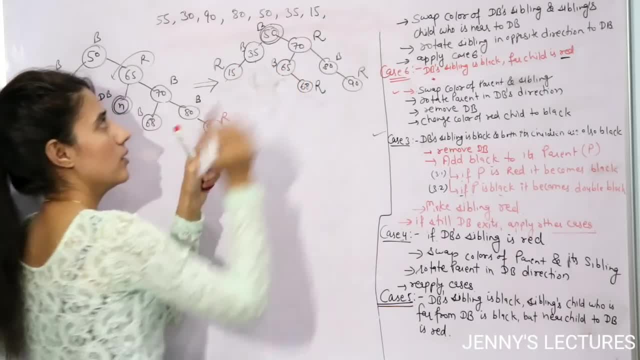 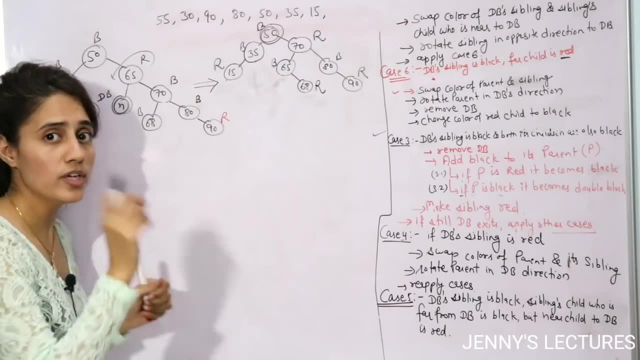 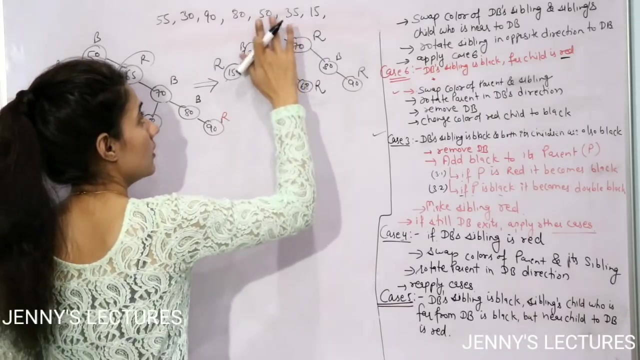 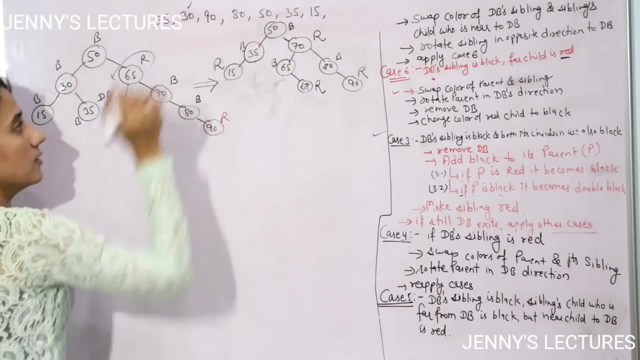 one. this would become angry, so it would become black to red. now the double black situation still exists, but here the double black is the root is double black. so in that case you will do what? simply remove double black, right? so simply remove it double black, and 50 is become single black now. so now this is the tree after deleting 30. 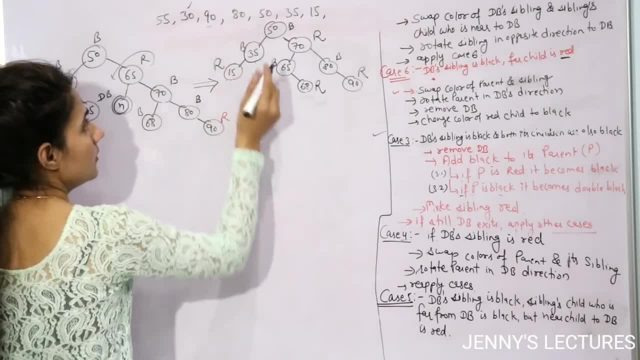 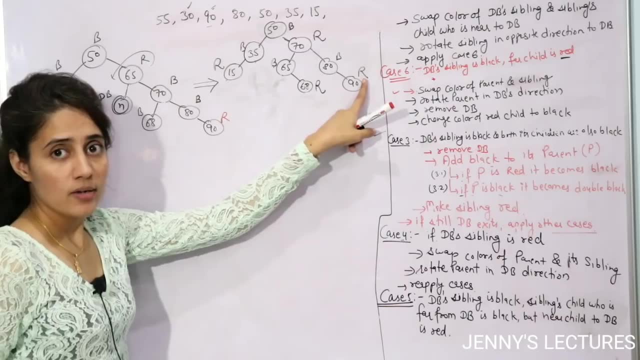 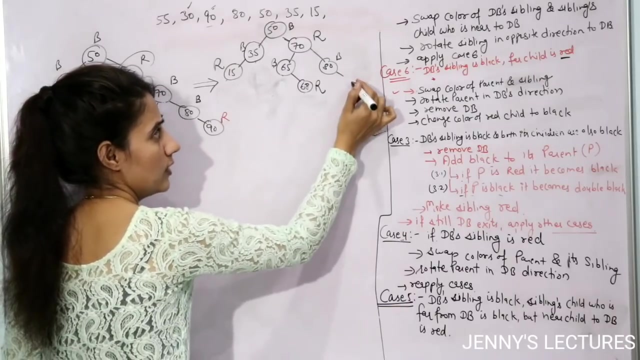 so this is. you can see it's a red black tree. now from here, delete 90. where is 90? here we have 90. see, now the node you want to delete is red, so you can simply delete it. no need to do anything right, because this is red. and if you will replace it with nil, then that would be a single black only. 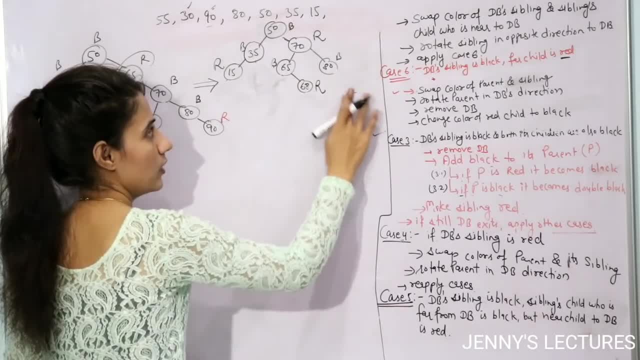 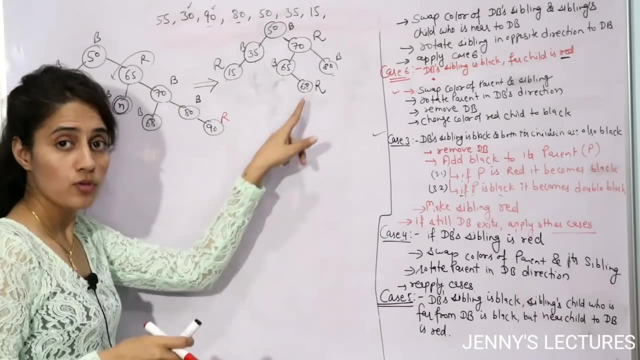 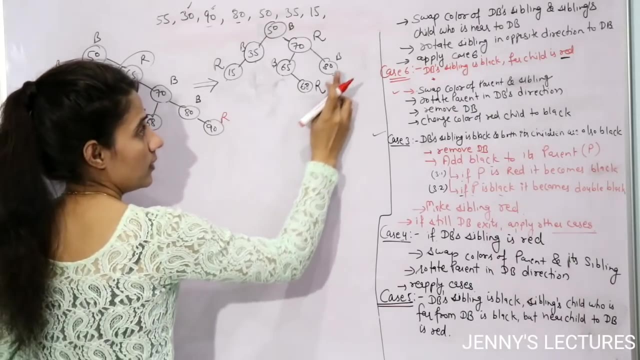 no double black situation is there no need to write down the nil, so you can directly delete this 90 right now. next we want to delete 80 from here. now you will see the mirror image of the case we have discussed earlier. see 80 you want to delete, but this is already black node, so you cannot simply delete it. 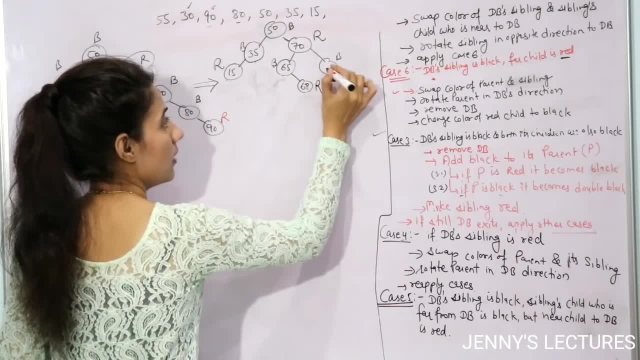 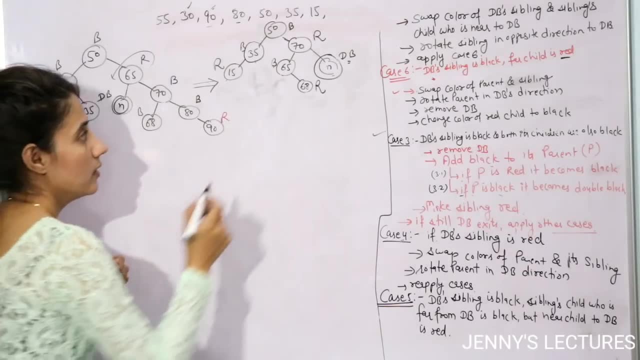 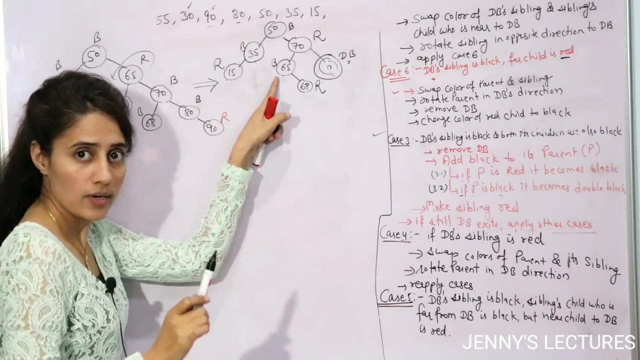 right, we will replace it with its nil and it would become now double black. now, here the problem exists. now you need to convert it into single black. right now. check out the sibling of double black. that is 65 is the sibling. sibling is black in color. right after that, check out the child of. 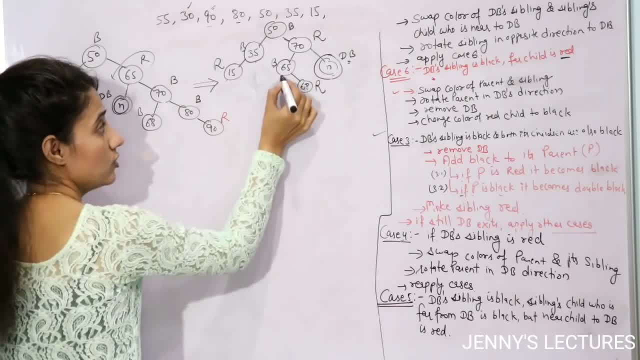 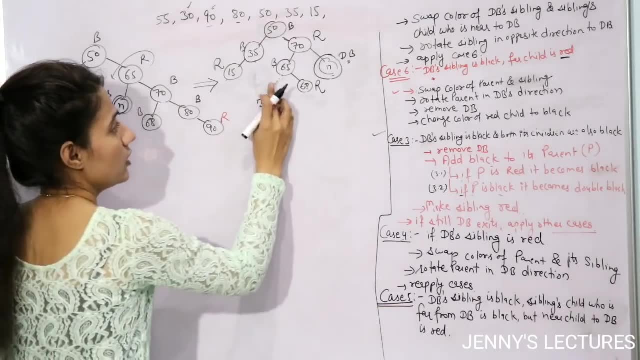 the sibling, which is far from double black. so this child is far from double black and this is nil, and this is black. only nil is always black. right now, check out the child which is near to the double black. this is red now. now which case you need to apply. see this one. 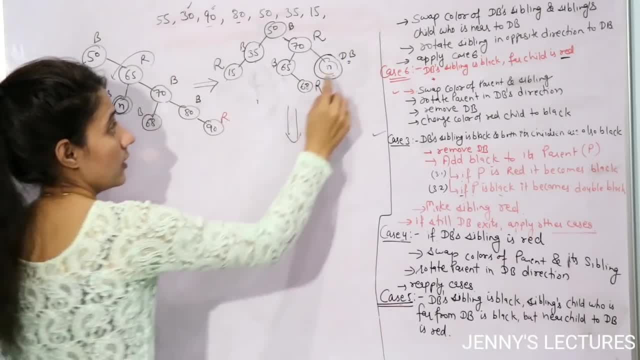 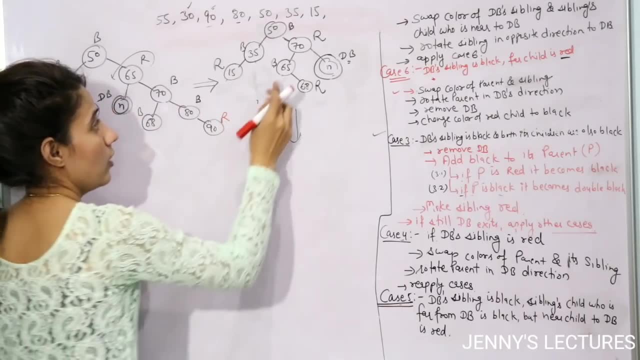 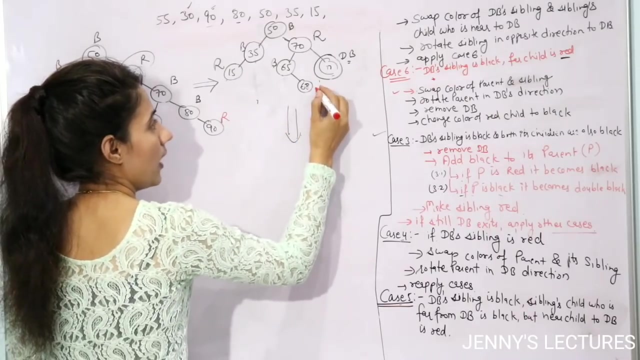 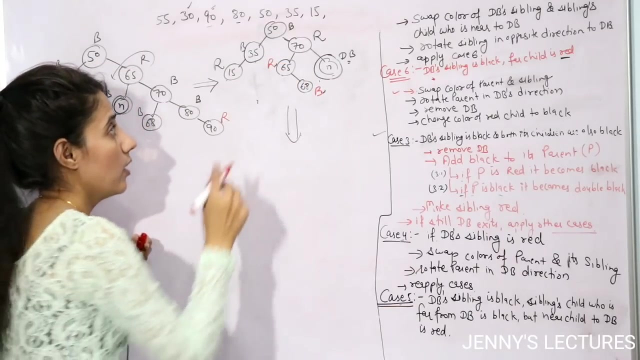 now, these are the steps, now what you will do. see, now he'll ask to its sibling that go to your child and cool him down, because he is angry right. so now he'll go to his child, to his child, and cool him down. that is why it become now black, but now the he become red right now. he was the one who went. 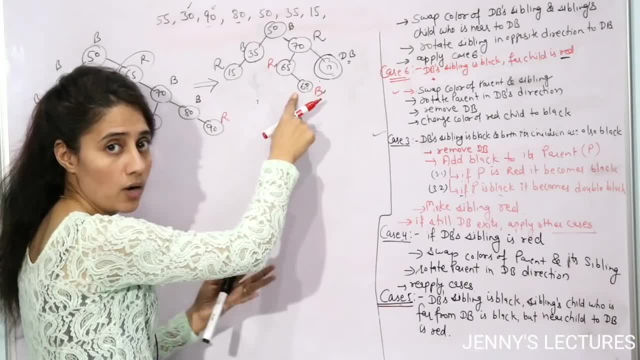 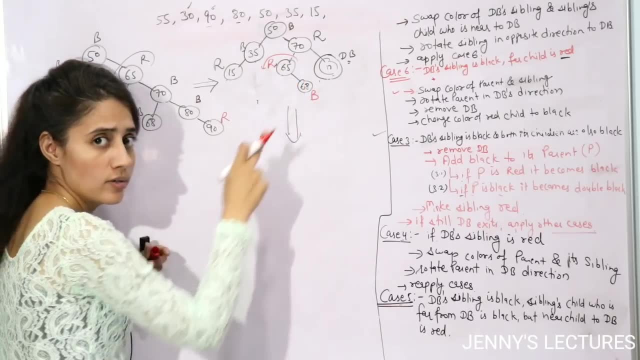 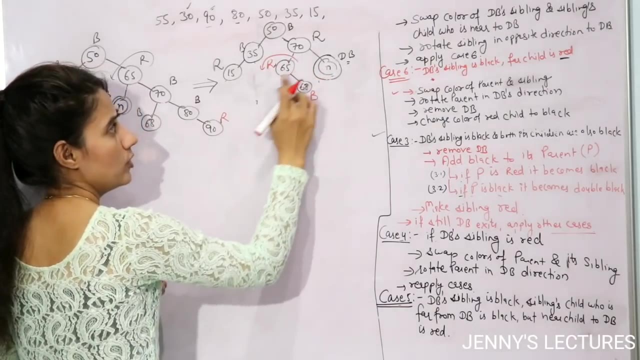 to cool his children, to cool his children, cool his child down. that is why he will rotate now. so now he will rotate because he was the one who went to cool him, to cool his child down. so that is why he will rotate. now he will rotate in opposite direction to db. why so? 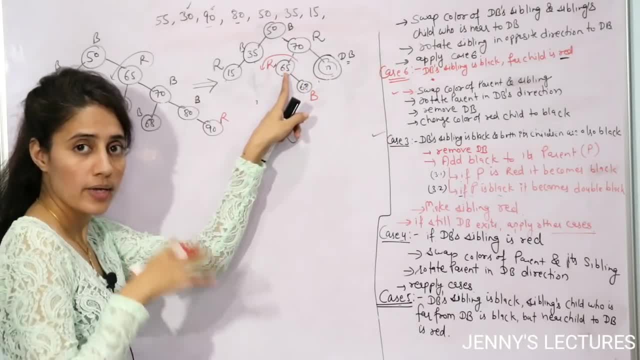 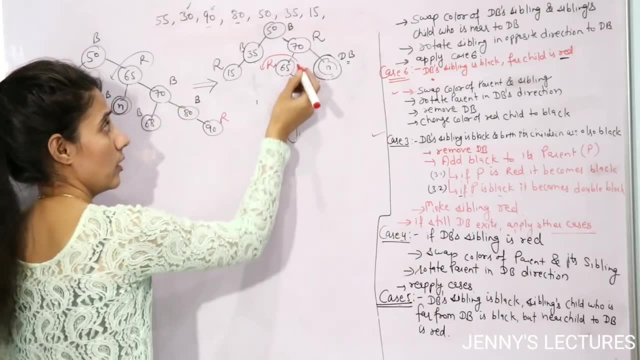 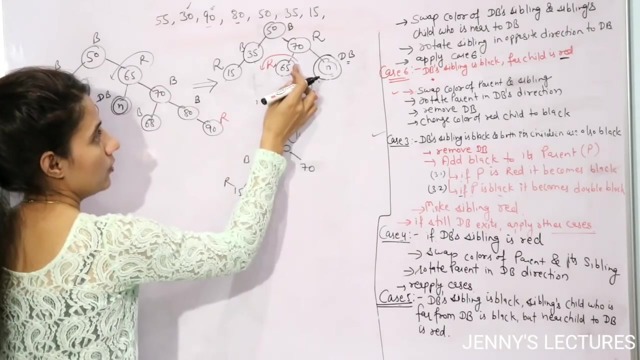 because he asked to go him to a child and pull him down. that is why he becomes angry now. he is angry with his sibling also, so now he will rotate in opposite direction to this db. so now the child. so now the tree would become. now it will rotate in opposite direction, so 68. 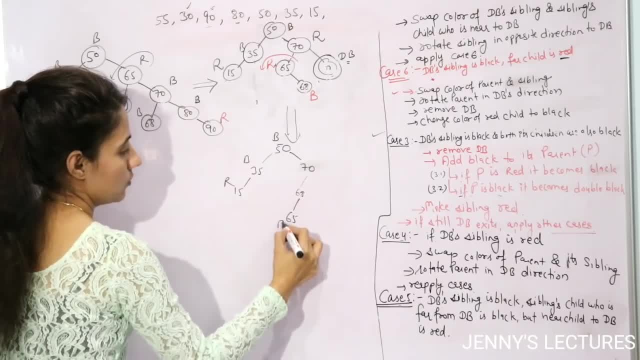 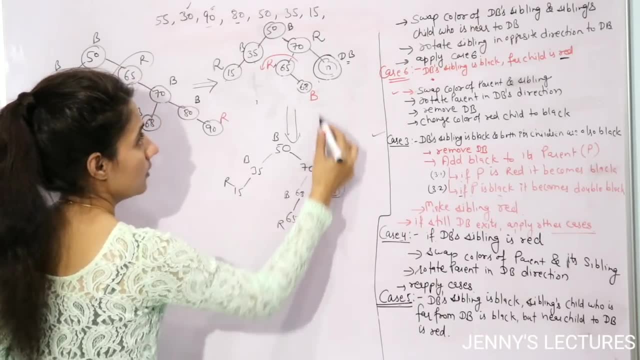 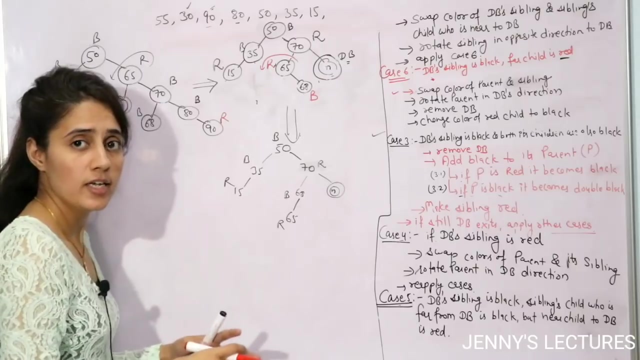 would go upward and 65 would go downward. now 65 is red and 68 is black, and this is still a double black problem. right, and 70 is red. now see, apply case 6, because once you apply case 5, definitely you will reach to a situation where you need to apply case 6. now. case 6 is what? this? 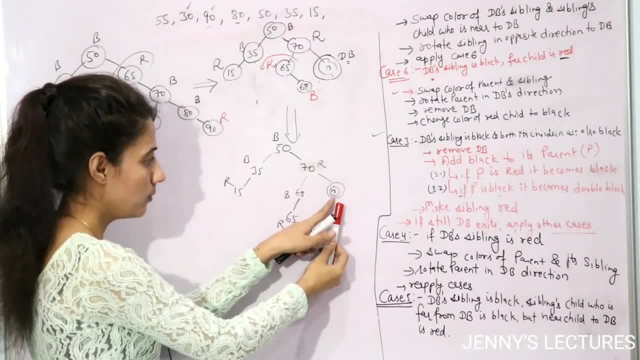 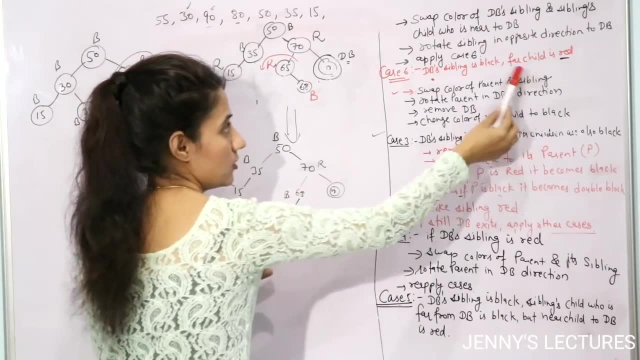 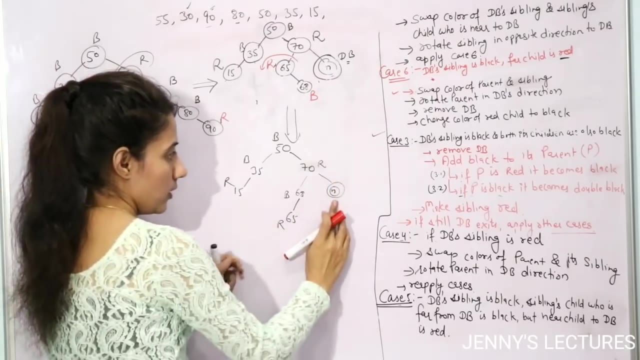 is the problem node having problem, db problem. so check out the sibling that is black. now check out the child which is far from db, which is red. far child is red. so that is why we've reached to case 6. ultimately, now applies case 6. now what you will do? now see, he'll ask to parent, his parent to go and 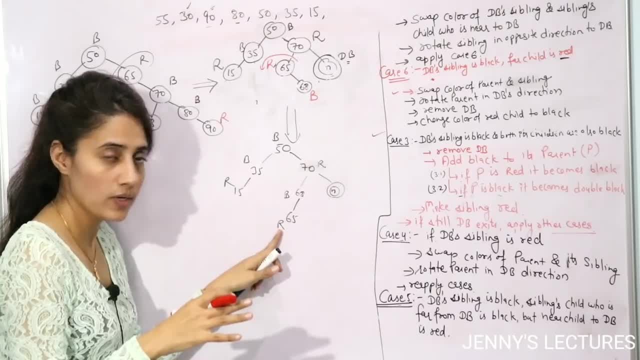 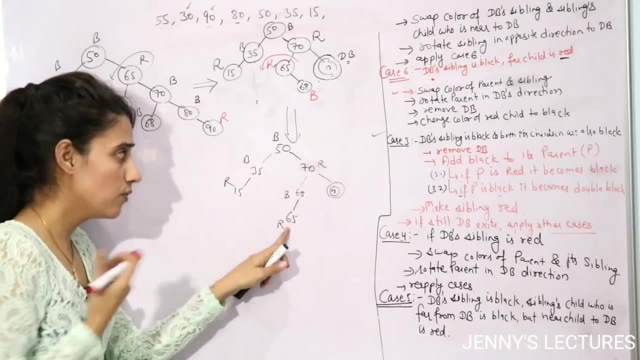 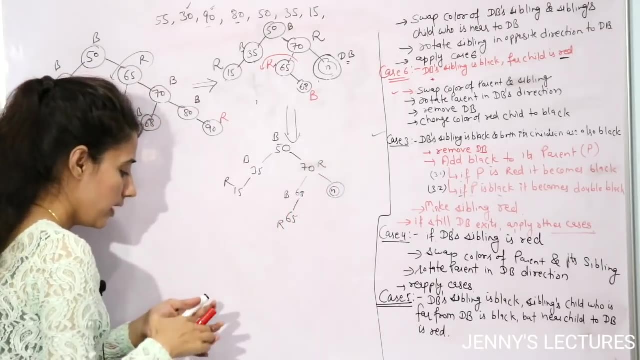 apply: calm his child down right now. he will not directly ask to sibling to go to its children. he will ask to parent, because this child is far from db right now. parent will go right. so that is why we are going to swap the color of parent and its sibling. so now see parent. 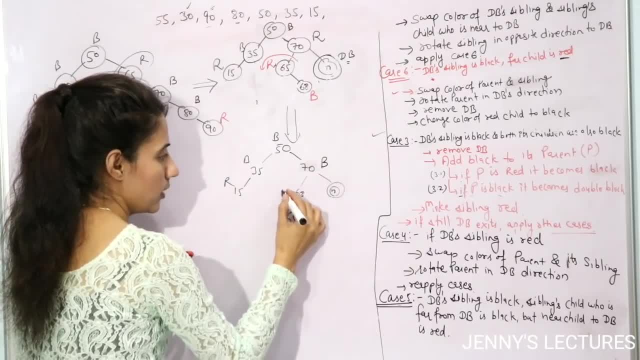 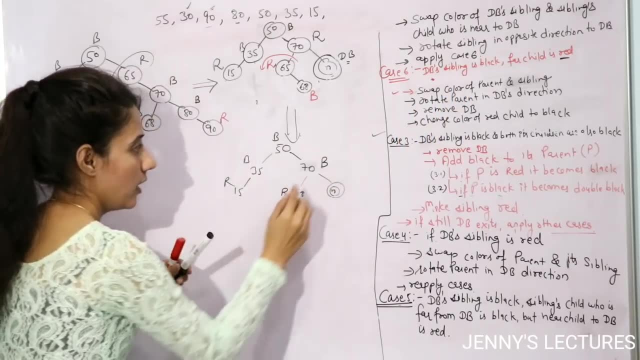 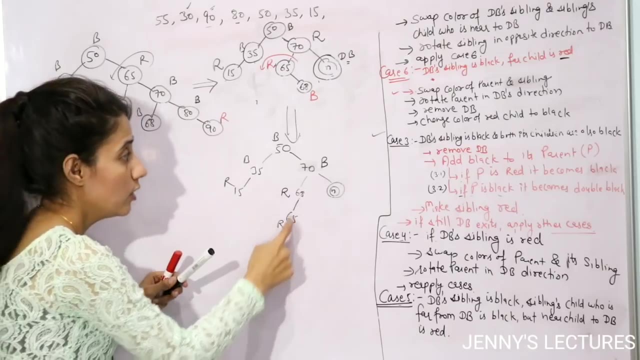 is red, so it will become black, and it is black, so it will become red. right after swapping color of, parent and sibling rotate. now he was the one who went to calm his children down, right, so now. that is why he will rotate now. so now he is parent of double black and parent will always. 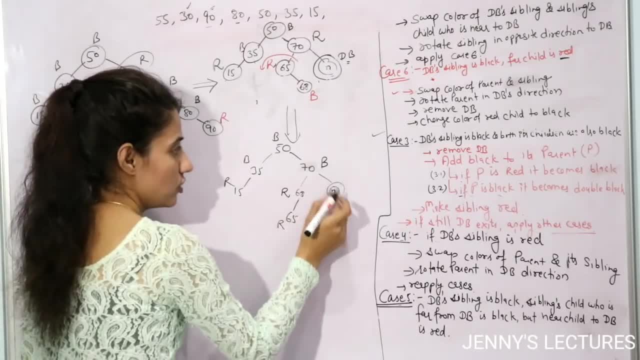 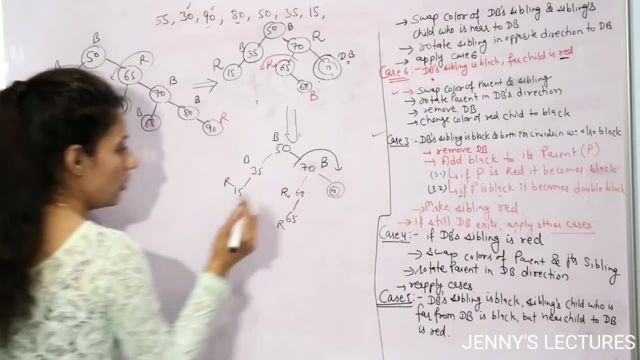 rotate in the direction of db right because this child is having problem. so parent will rotate in the direction of the children which is having problem right. so now, after, rotation tree would be something like this: 70 would go downwards, 70 would go down and 70 would go up and 70 would go. 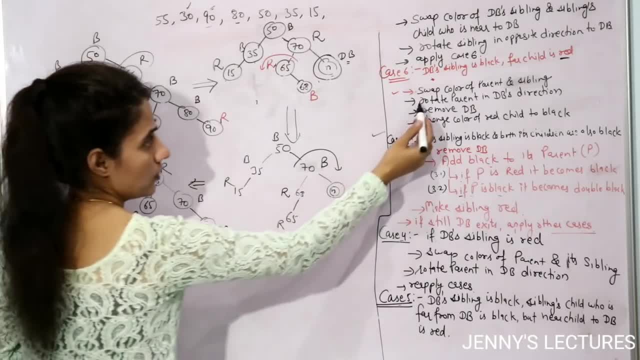 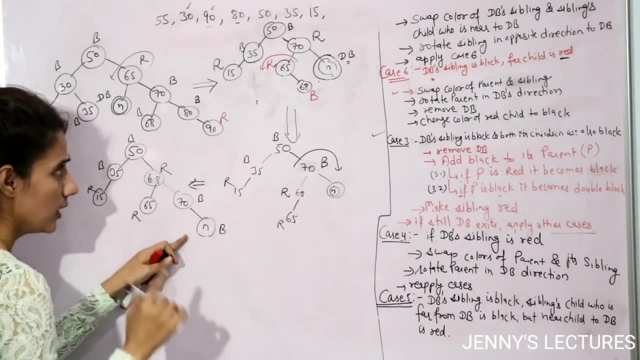 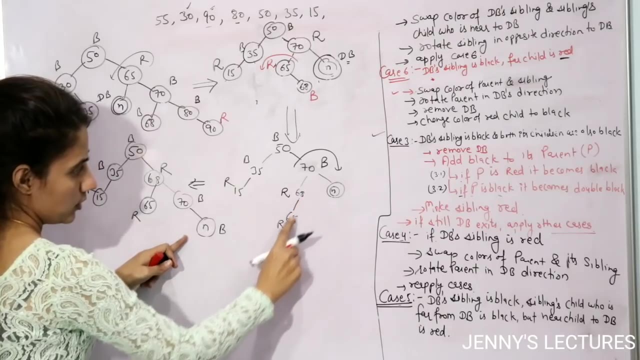 68 would go upwards. 68 is now red. now, after rotation, remove db. so db is this one. so remove this thing. this would become only null. that is, one black, and change the color of red child. see, the red child was this one because because of the 65 was red right, so 65, the far child was red, so 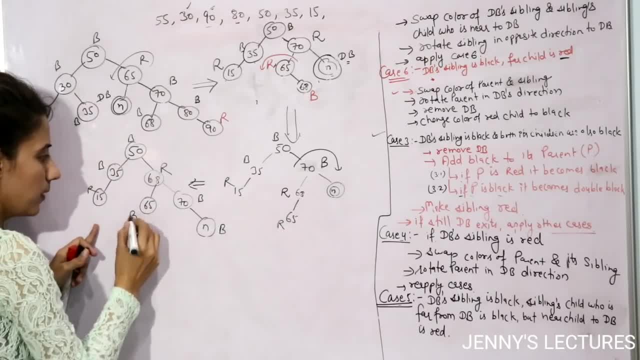 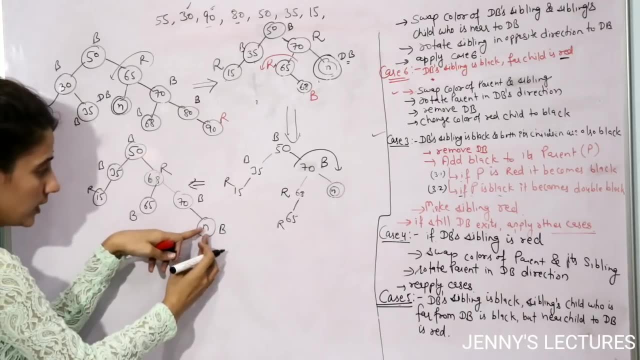 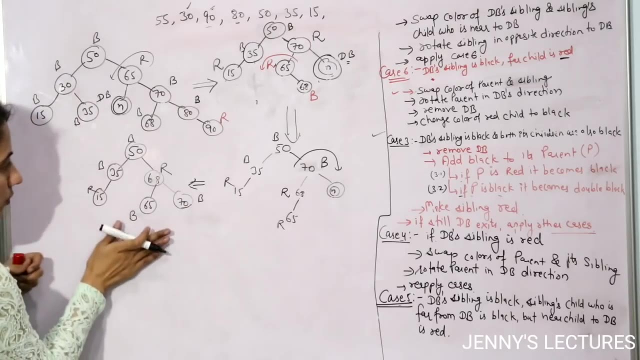 it would become now black. so 65 now becomes black. see, now it will push its problem upward, right. so 65 is one level up from this. so he can give one extra black to 65 now, right. so now this is only null, so you can remove it. no need to write it down. so now this is the tree, as you can see this. 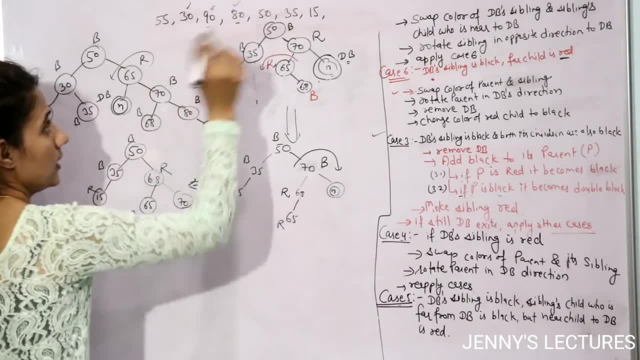 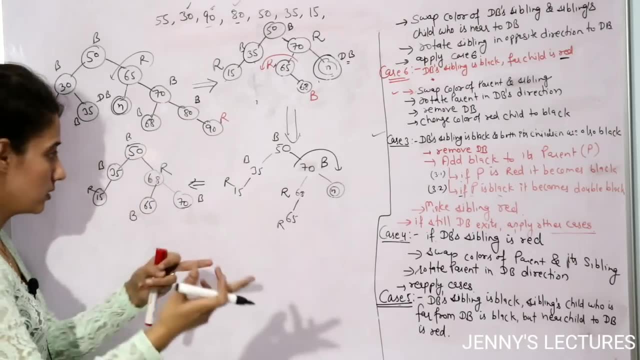 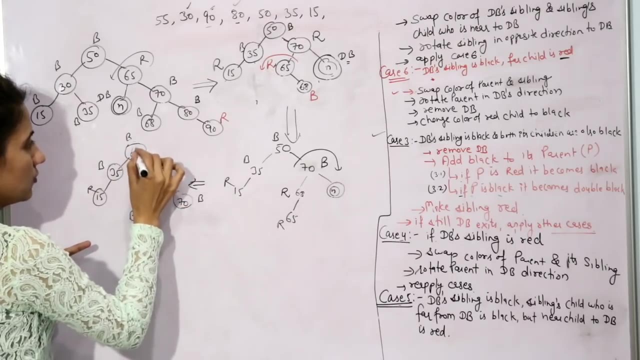 is now a red black tree. after deleting what, 80. now we will delete 50. 50 is having two child, so we will replace it with its in order successor. in order successor is what, from the right sub tree, find out? the smallest. smallest is 65, so here you will write 65. 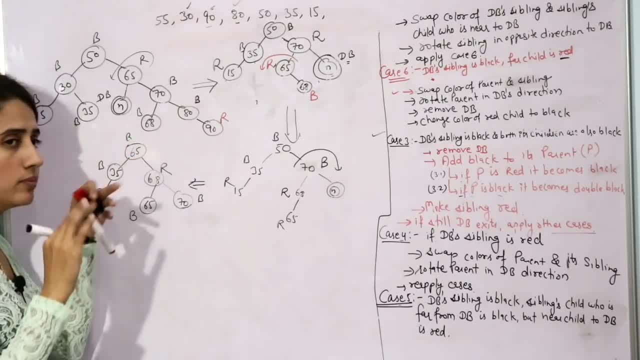 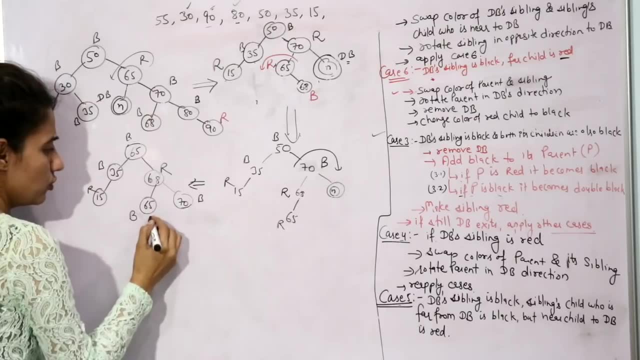 you are not deleting this, we are replacing the value only. so it would become, it would remain. it would you know, retain its color, right? that is black. now 265 are there, so we will call recursively the delete function on this in order successor. so we will delete this one, but this is black, so you. 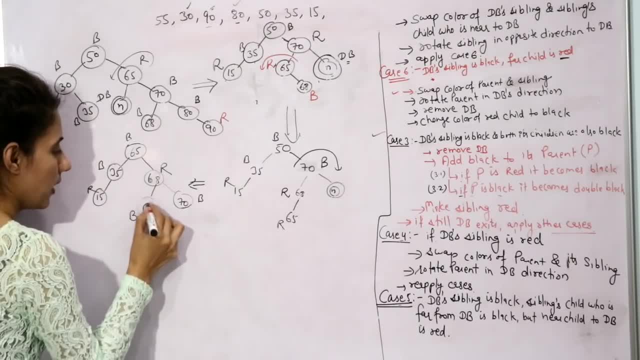 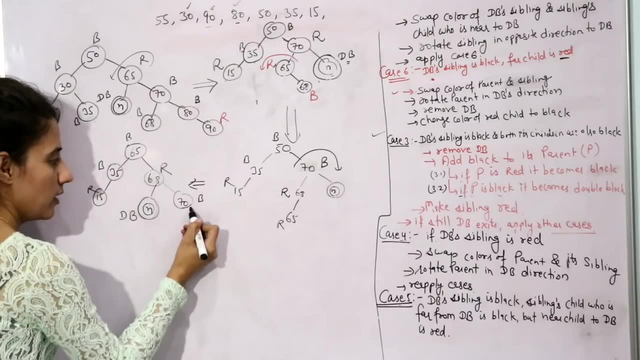 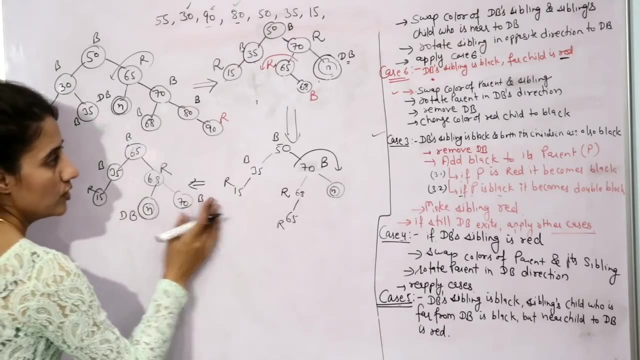 cannot directly delete it, so it would become now double black right. so now which case you need to apply sibling. check out the sibling which is black. check out the far child of sibling that is null. left child that is nil, that is also black. now which case you need to apply case three in this. 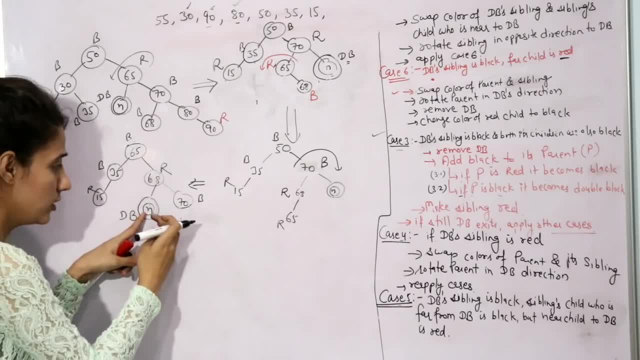 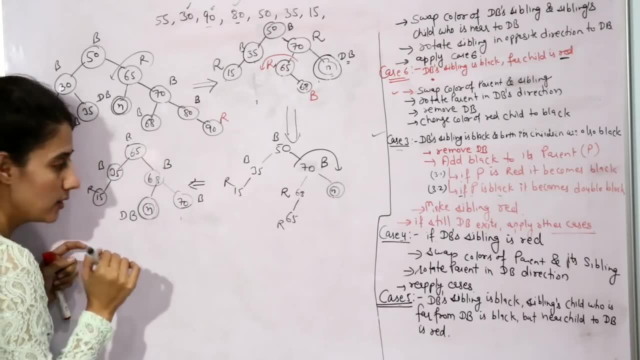 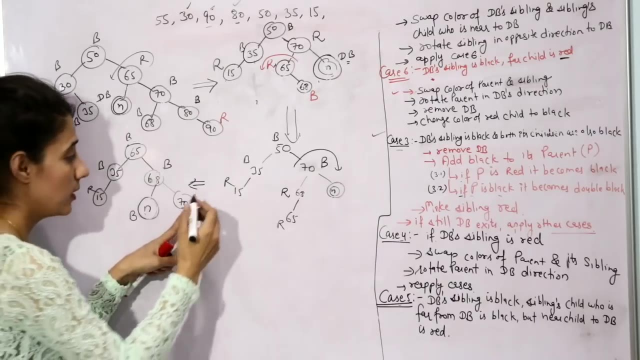 case he will push its problem. or you can say: it's extra black to its parent. right now, parent is red, so it would become now black. right, and it would become single black. now, after seeing this one, the sibling becomes angry, or you can say: becomes red. that why you are giving your problem to a parent. 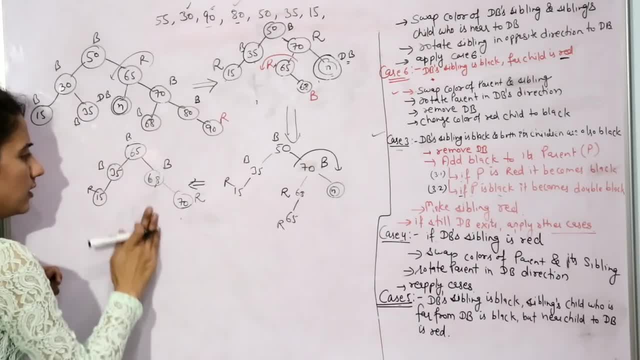 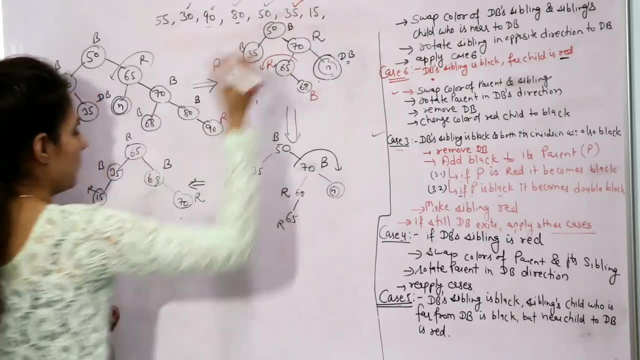 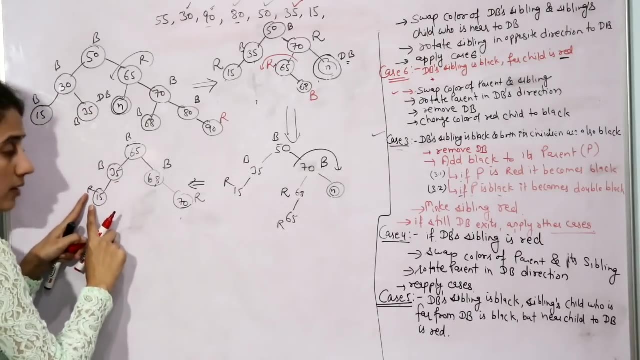 right now this is null or single black, so you can delete it, no need to write down the null. so now this is the tree. after deleting 50. now, next, i want to delete 35. see where is 35 less than 65. here we have 35, right, 35 is having one child, that is red child. so simply, first of all, we will replace this. 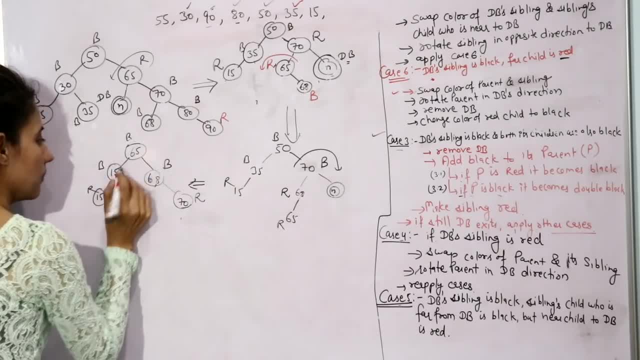 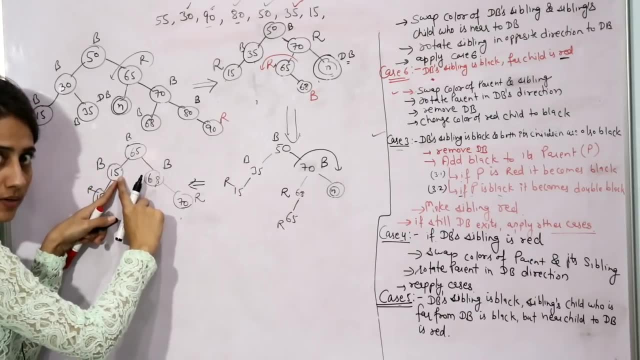 35 with its child. that is 15, but the color would be same. that is black because we are not going to delete the node, we are just going to delete the node and we are going to delete the node, so we are just replacing the value. right now we need to delete this 15, right? so now 15 is red, so you can. 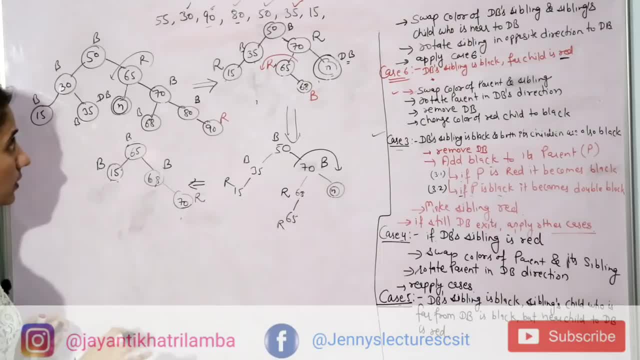 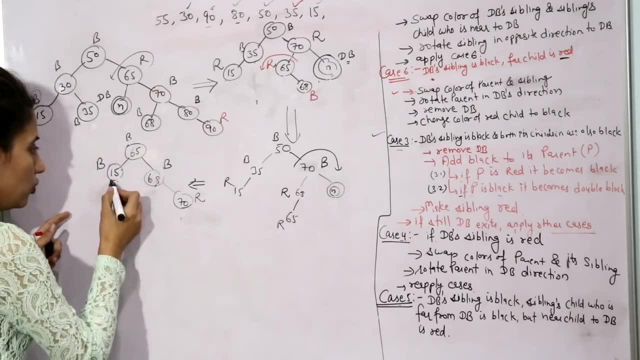 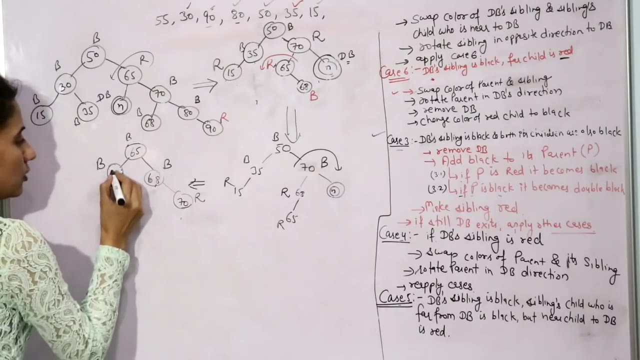 simply delete it, no need to do anything. so this is now a red black tree right now. next, delete 15. here we have 15. 15 is black and it is having two nil child. those are also black. so you cannot directly delete it, right? so we will replace it with null and it would become now double black. 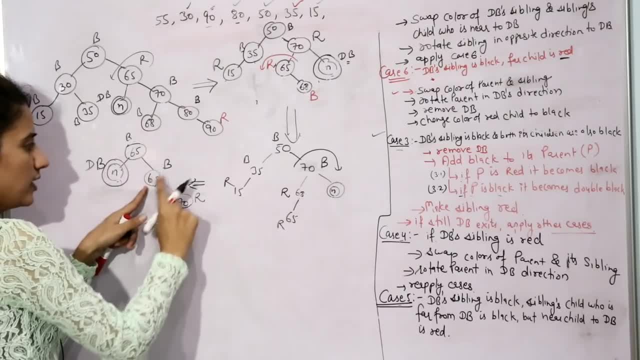 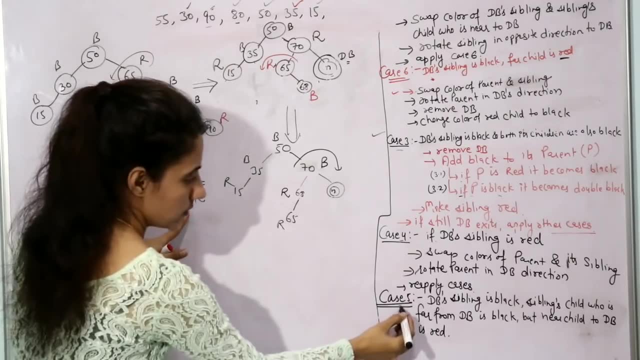 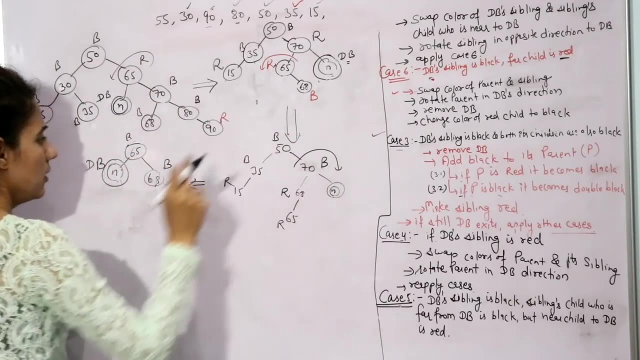 which case you need to apply double black sibling is black. check out the far child, far child of double black is red. now the situation is this, one sorry situation is this one case six directly. you need to apply case six now, right now, what you need to do? so now he will ask to its parent to go and 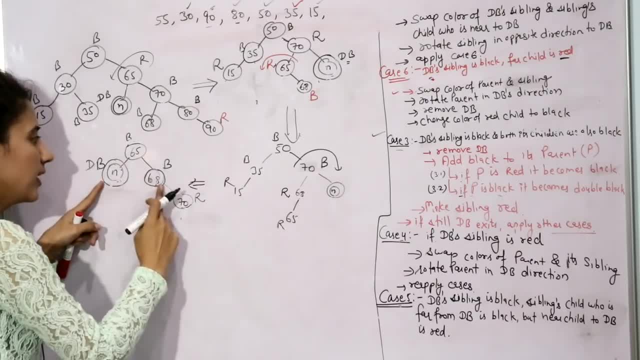 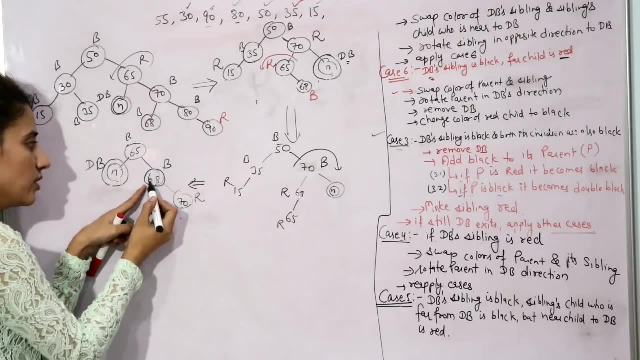 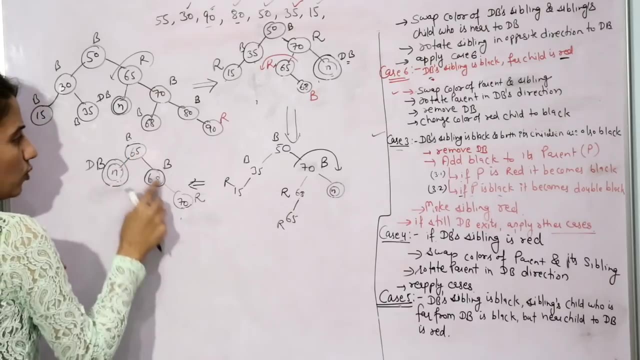 ask you can say, his sibling to cool his child down. he will not directly ask to his sibling in this case. if the case is the case is far child is red. if near child is red, then he will directly ask to his sibling to go and cool his child down right now. if parent will go, then parent and we will swap the color of. 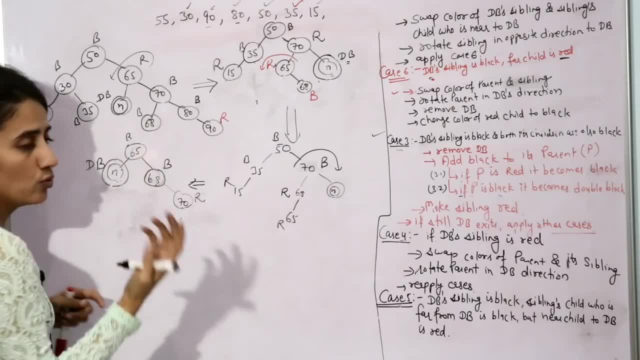 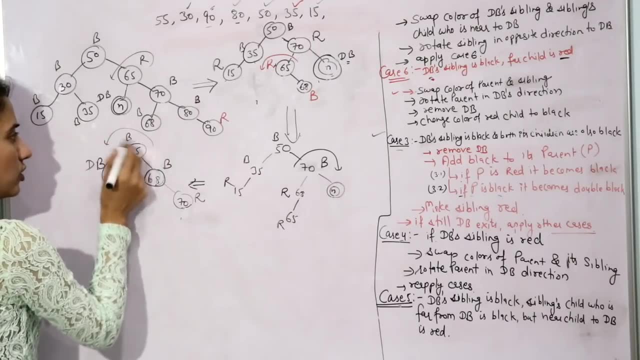 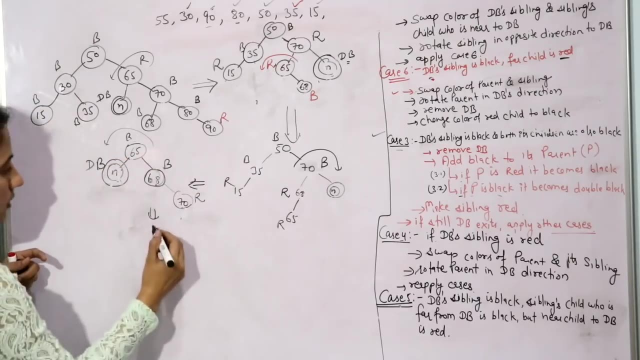 parent and this sibling, but both are black, so no need to do any swapping right now. after this, after swapping, this parent will rotate. in which direction? towards db direction. so now the situation would be: 65 would be rotated towards this, 68 would go upward 60. it is black, here we. 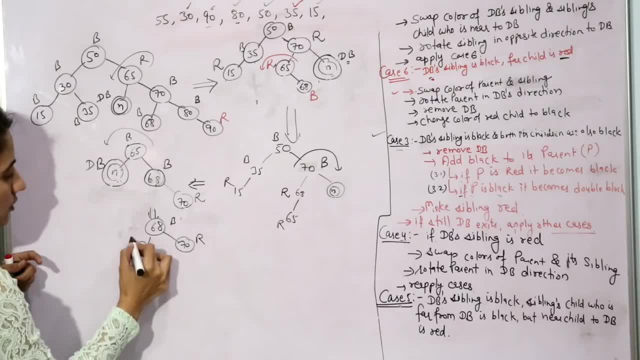 have 70, which is red, 65 is black, and here we have now double black, right now. now see this: this child was red, he was angry. right, the far child, 70. so now the 70 is one level upward to double black. so now he can give its extra black to this 70.. so now he can give its extra black to this 70.. so 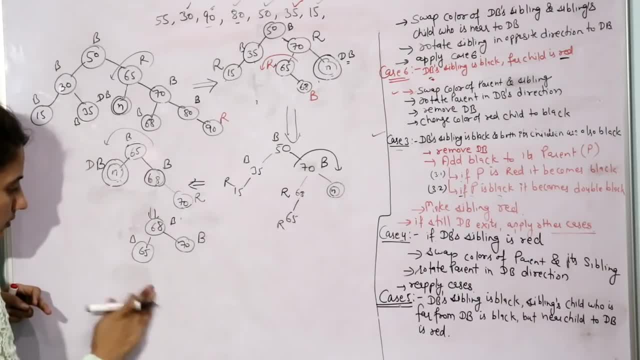 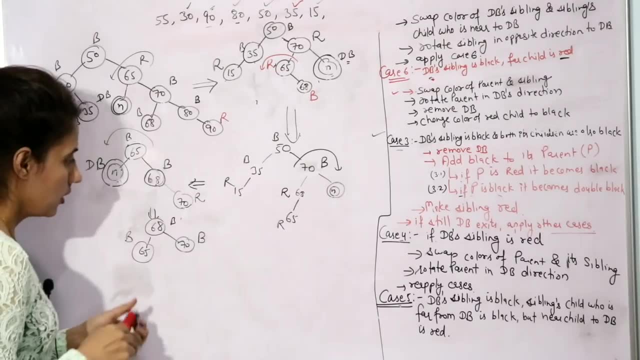 now 70 becomes black and it would become single black, so you can remove it, no need to write down this thing. so this is the tree after deleting 15. so this is now you can see a red black tree. so now, suppose, if you delete 65, i want to delete 65, see where is 65 here we have, but this is black. 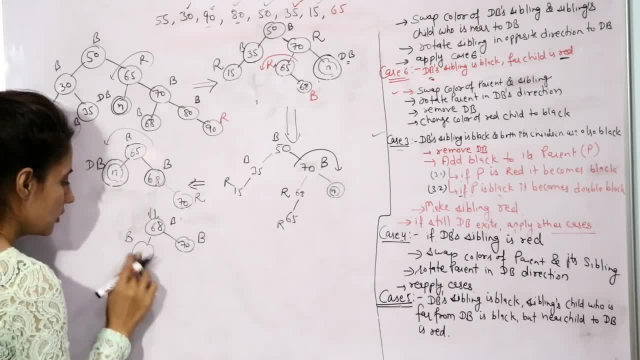 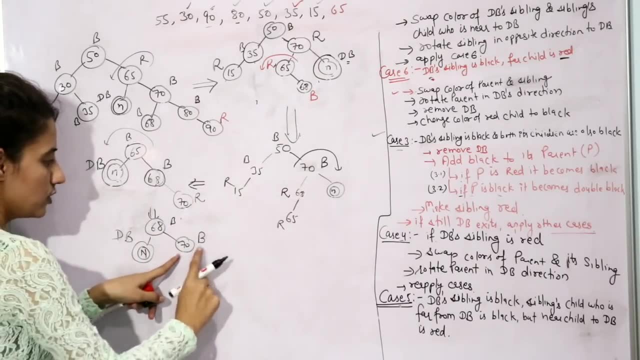 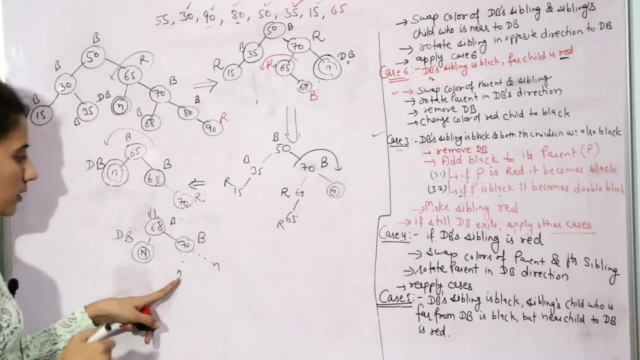 you cannot directly delete it, right? so after deleting this, this would become: would be replaced by null, so it would become now double black. now check out which case you need to apply. check out the sibling, which is black. the first child is also black. the child is also black because both are null. so which case you need to apply this thing now he will. 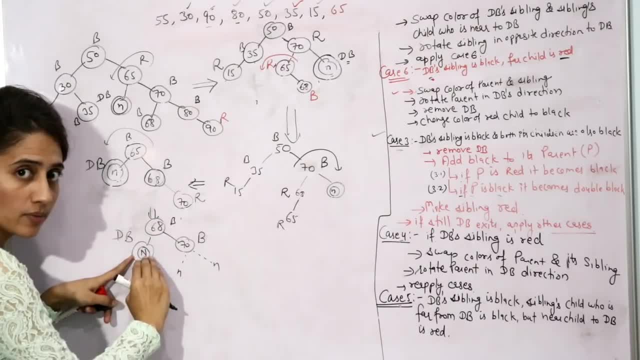 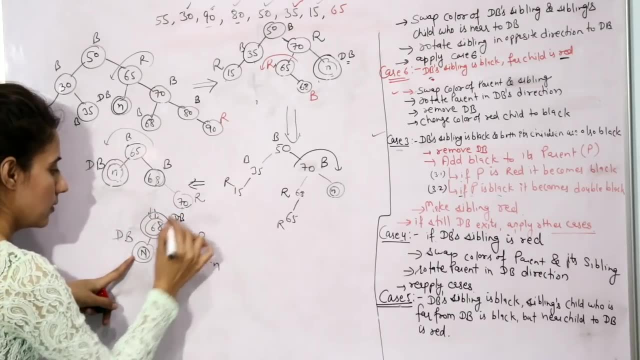 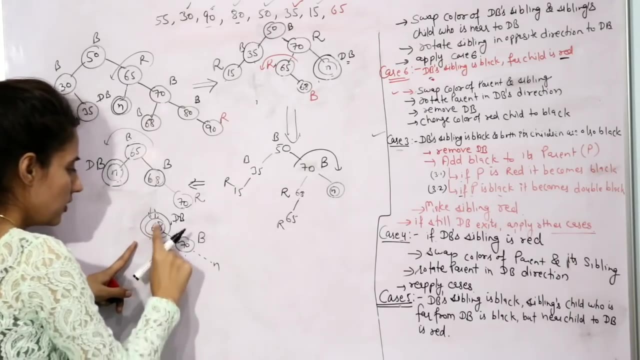 push its problem to its parent. that is the extra black he will give to its parent. now, parent is already black, so it would become double black, right. and now it would become single black, right. so this, this is null, so no need to write down this thing now, after seeing this situation.